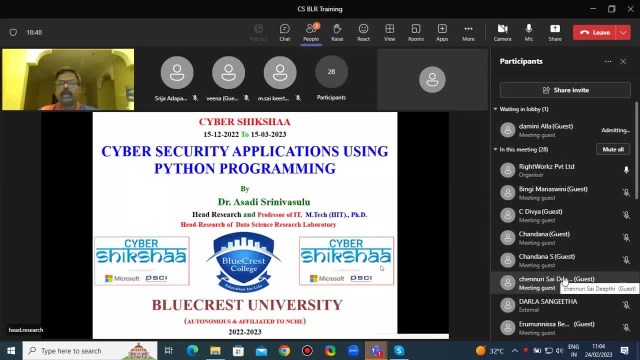 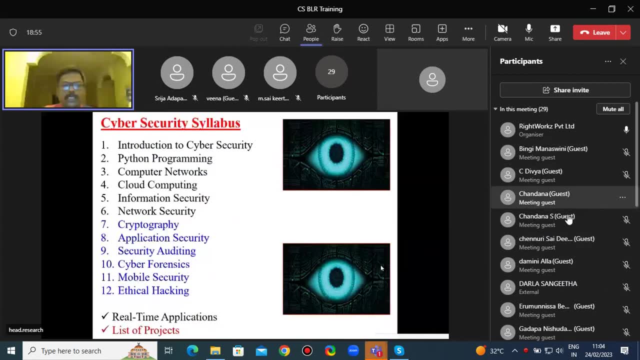 Today I am going to explain another module called yeah. there are 12 modules- Introduction to cyber security: Python programming, computer networks, cloud computing, information security, network security, cryptography, application security, security, auditing, cyber forensics, mobile security. 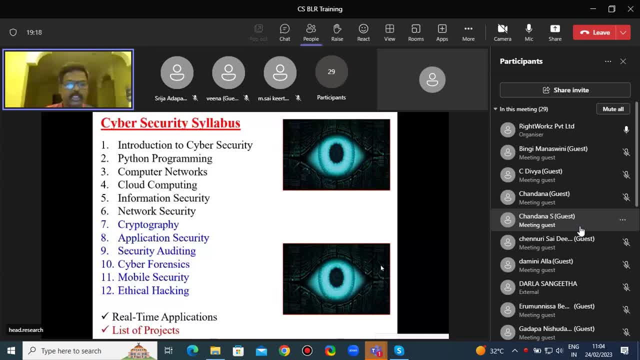 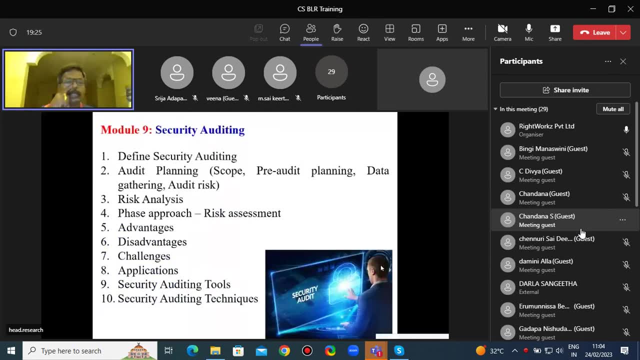 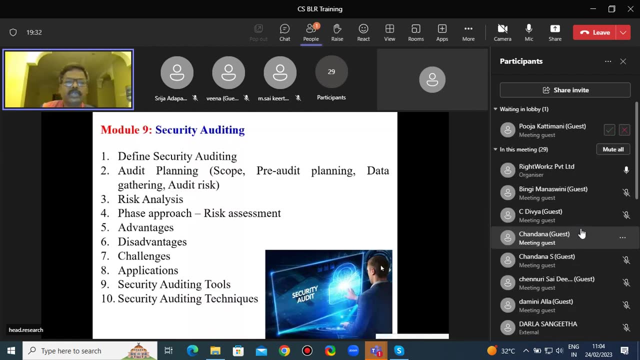 ethical hacking. So, out of 12 modules, today I am going to explain 9th module, security auditing. 9th module: security auditing: What is meant by security auditing and define security auditing and, in this audit planning, what is audit planning? In this one, we need to explain what is meant by scope of audit planning. 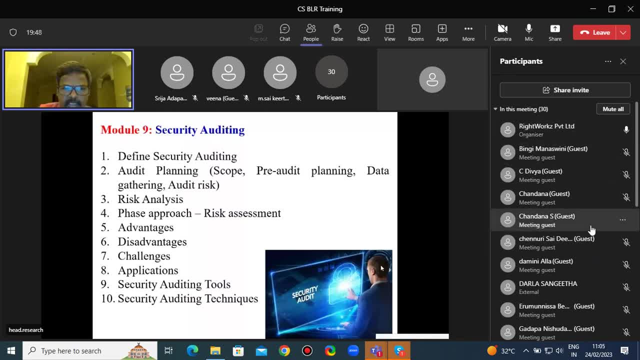 Pre-audit planning, data gathering, audit, risk, then followed by the risk analysis phase approach, that is, risk assessment. what are the advantages of security auditing? what are the disadvantages of security auditing? what are the research challenges? research challenges of security auditing. 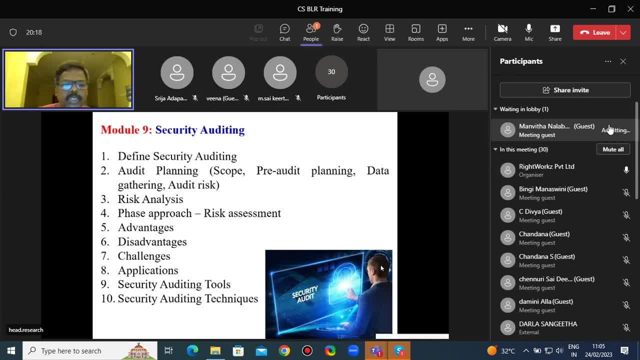 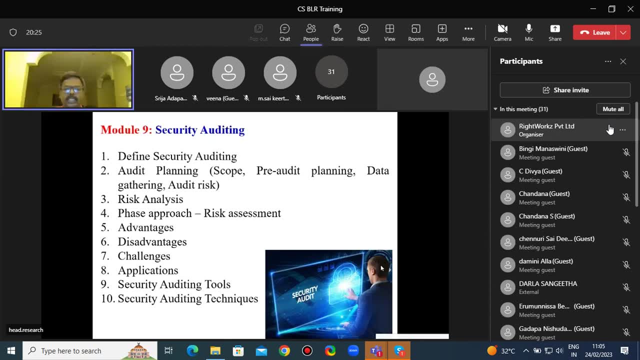 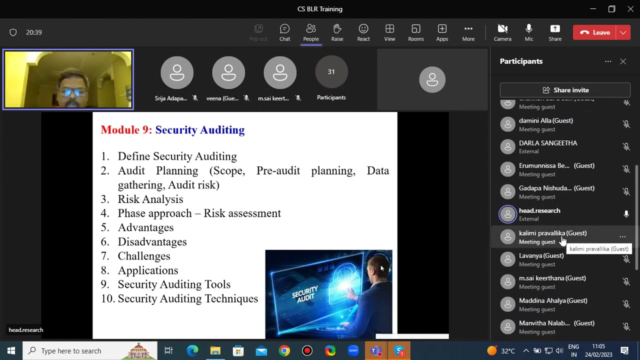 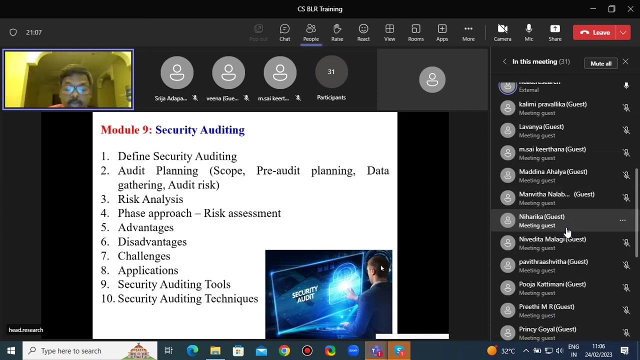 security auditing, security auditing tools, security auditing techniques. So these are the 10 topics today I would like to cover and followed by the project implementation Today, complete project implementation and there are 11 terms I have identified in cyber security, Each tool for each group. I am giving today for homework. you need to identify that tool, features, services and you need to do the presentation next week. So cyber security tools are 15 tools are there, but out of 15 tools I have chosen best 11 tools for 11 batches. 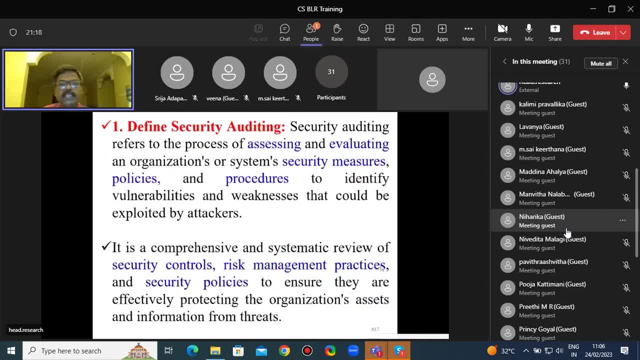 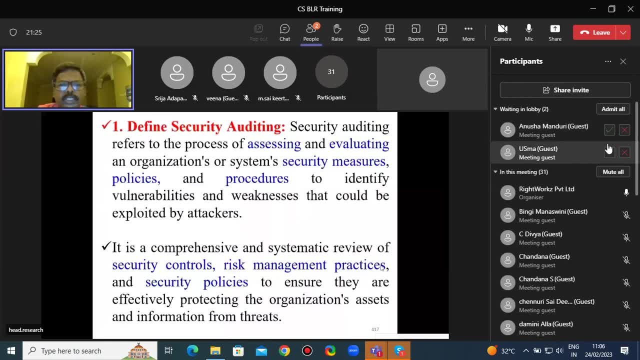 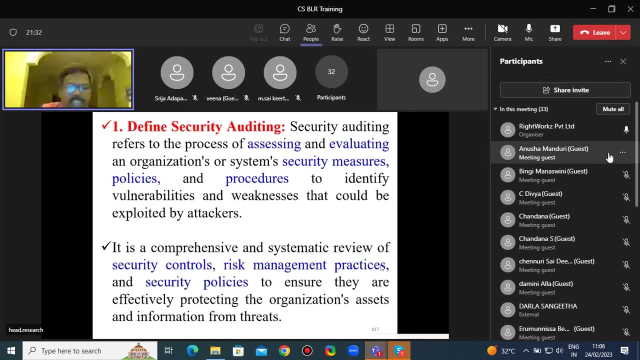 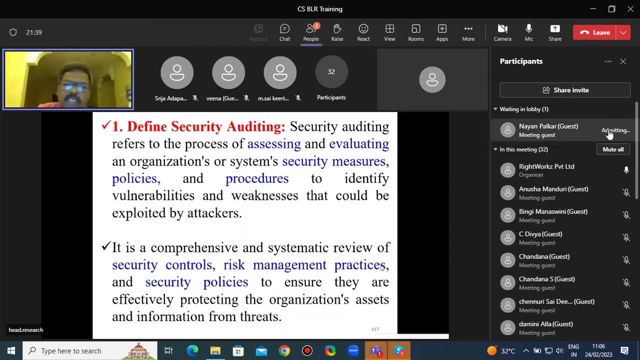 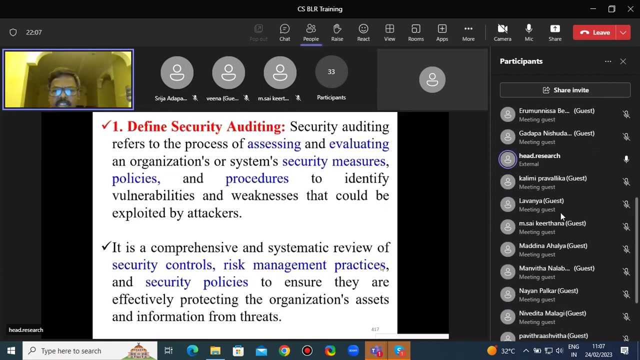 Okay, so what is meant by define security auditing? See any organization or any university. there is an auditing committee. they are checking the quality of education, the quality of the product and they are checking the employees of that organization. These parameters they are checking auditing team. Security auditing refers to the process of assessing the quality of the product, assessing the employees- how many are working- and evaluating an organization's or system's security measures, what sort of security measures they are using and what are the rules and conditions. 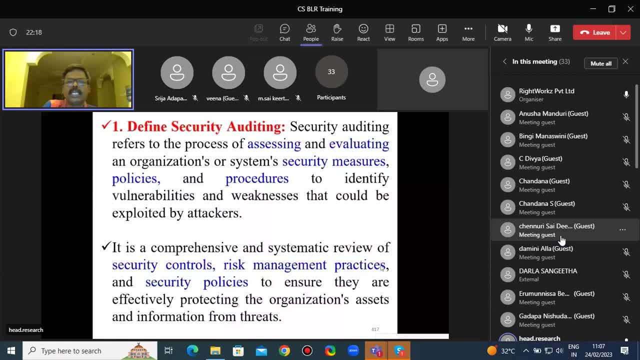 That is part of policies and the procedures. what type of procedures and protocols they are using to identify vulnerabilities means security issues and weaknesses, or errors or mistakes, or any cyber attacks, cyber crimes, what not? So vulnerabilities and weaknesses that can be identified? Security auditing could be exploited by attackers, malicious attackers or cyber criminals. 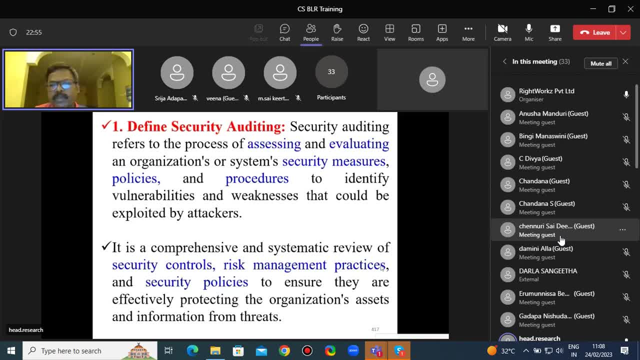 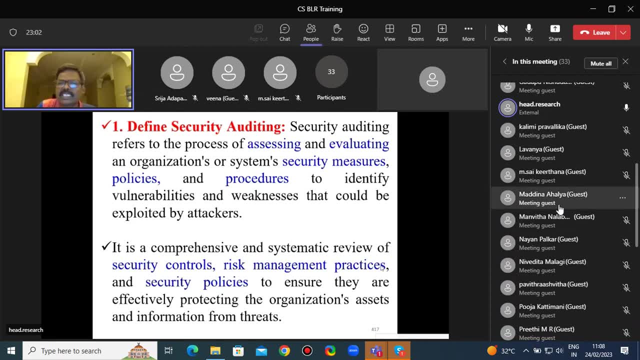 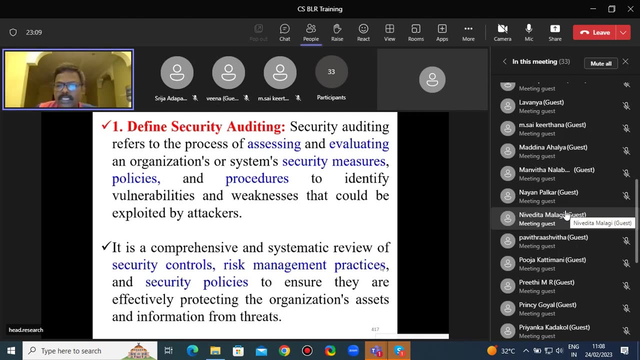 Such type of information is called security auditing. Keep in mind security auditing. they are assessing and evaluating organizations or systems, security measures, policies, protocols, procedures, rules and regulations. Why, Why, Why? What is security auditing for? To identify vulnerabilities or any weaknesses that could be exploited by attackers. 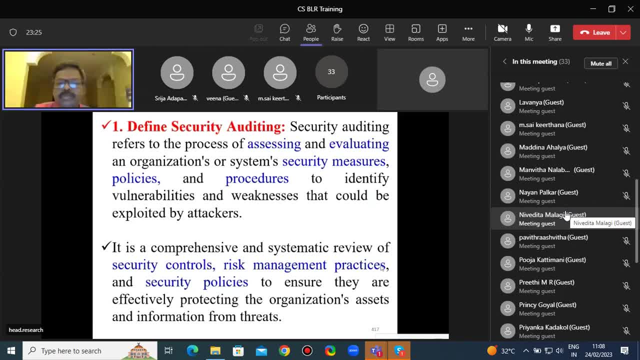 It is a comprehensive and a systematic review of security. controls means security measures, risk management practices and security policies To ensure they are effectively protecting the organization's assets and information. Why assets and information from threats. So they are doing comprehensive and systematic review. 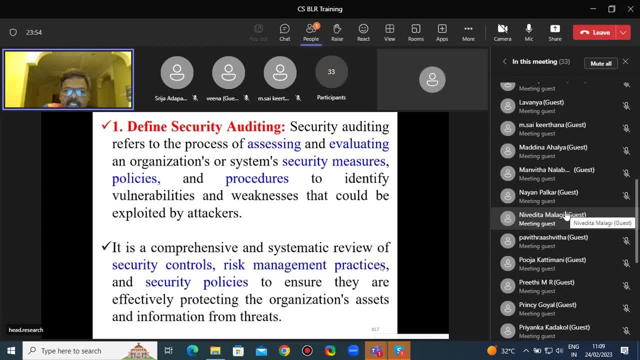 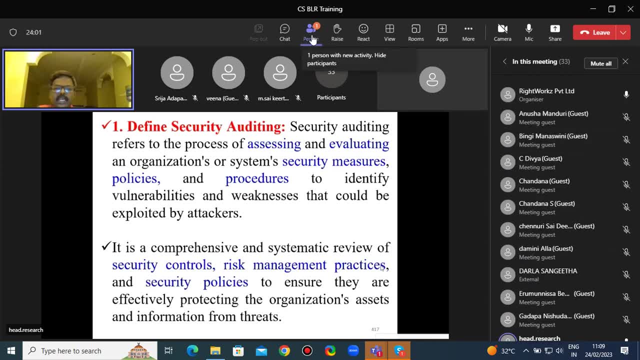 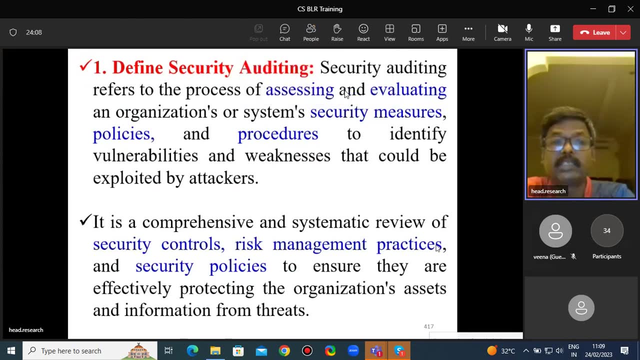 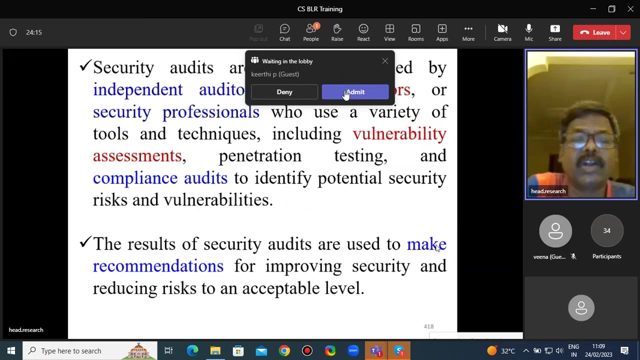 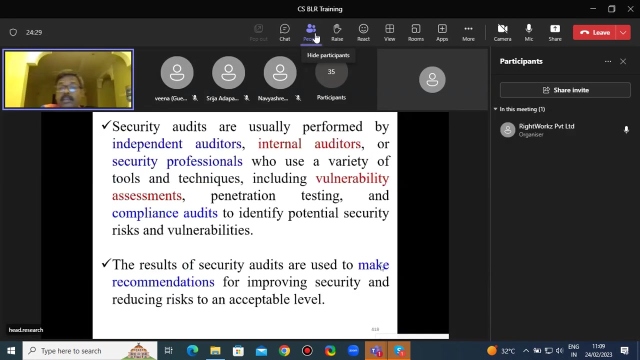 in order to identify various types of vulnerabilities and weaknesses. So why they are doing? They are effectively protecting the organization's assets and information from the threats. Security audits are usually performed by independent auditors. Maybe they are conducting, as independent auditors- internal auditors- before visiting external auditors in order to assess and evaluation. 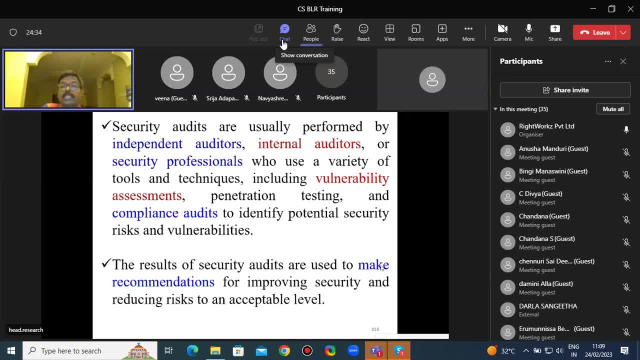 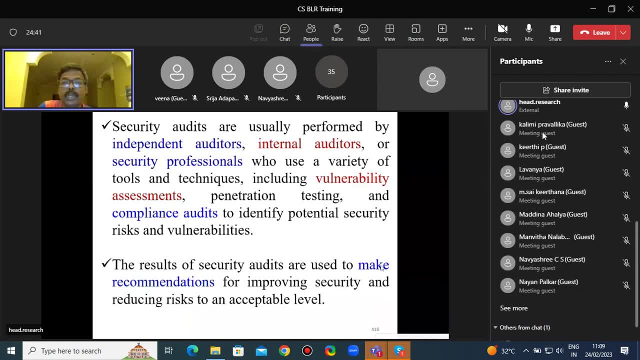 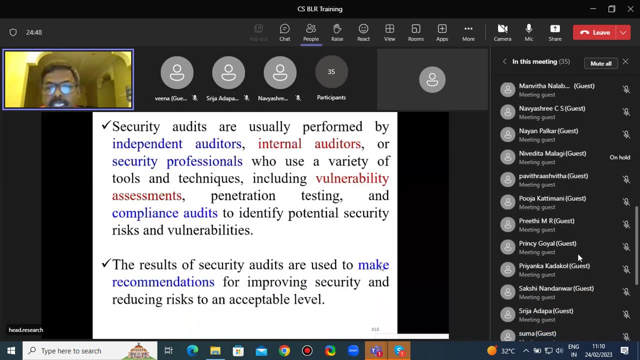 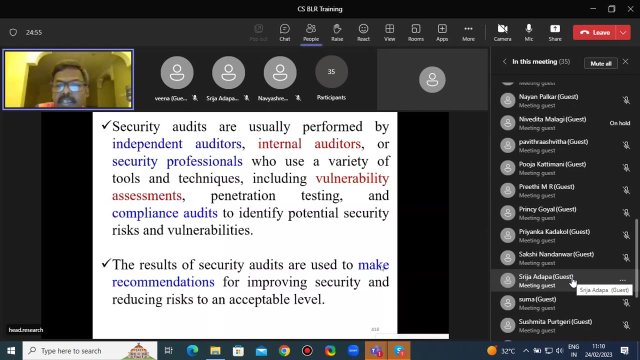 in order to perform, companies and the organization, assessment and evaluation of the employee and the quality of the product, Or security professionals, who use a variety of tools and techniques, including vulnerability assessments, penetration testing. they are checking whether that organization having some rules and regulations, protocols and employment policy notification of the employee. 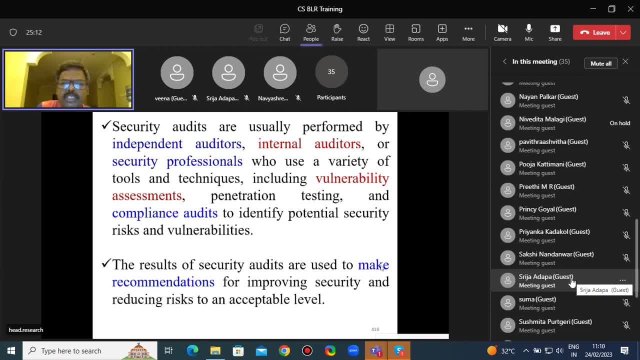 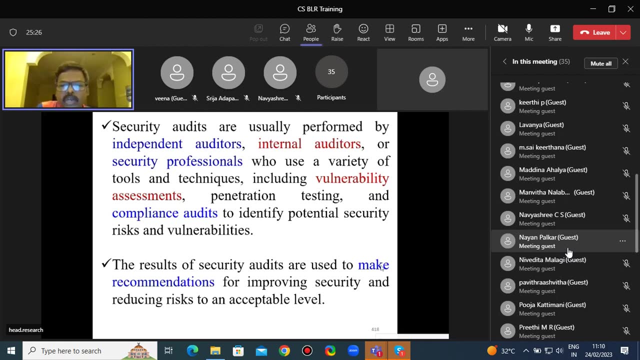 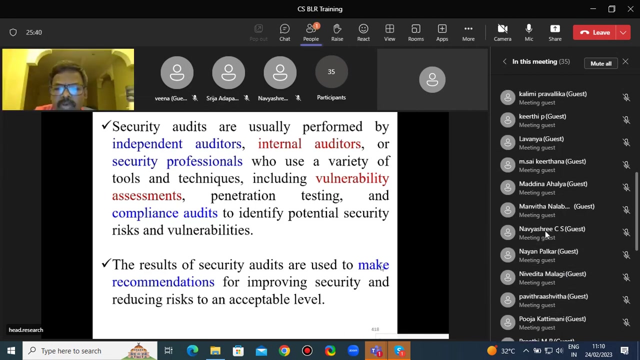 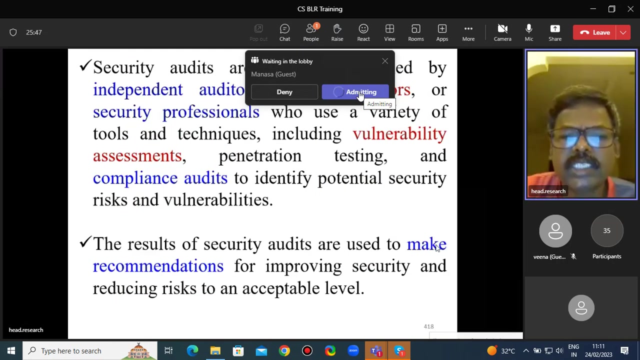 welfare. Various things are being done, Since they are going to check insurance and compliance audits to identify potential security risks and vulnerabilities. Then the results of security audits are used to make recommendations. The results of security audits are used to make recommendations. They are going to give suggestions and conclusions for you. 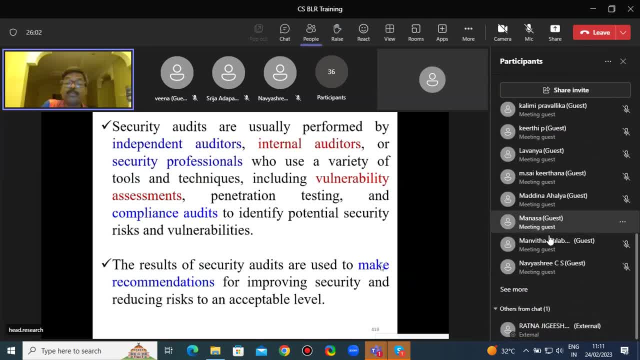 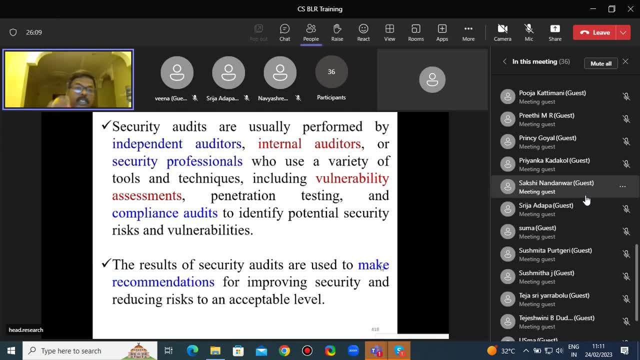 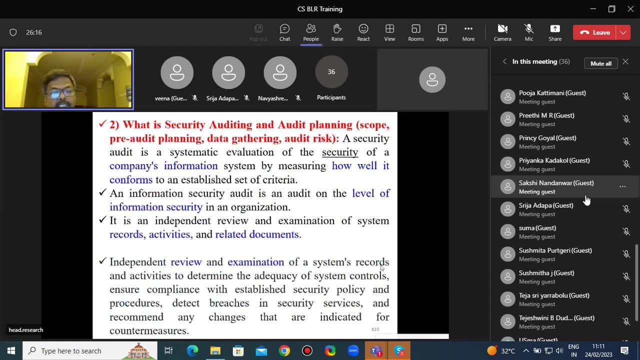 In an organization or in a system. So the second concept is: what is security auditing and audit planning? It includes scope, pre-audit planning, data gathering, audit risk. If you see a security audit is a systematic evaluation. If you see a security audit is a systematic evaluation. 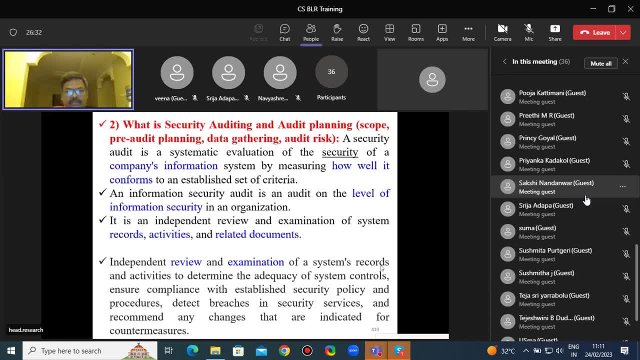 It is an evaluation of the security of a company's information system by measuring how well it conforms to an established set of criteria. So that is called a security audit. An information security audit is an audit on the level of information security in an organization. 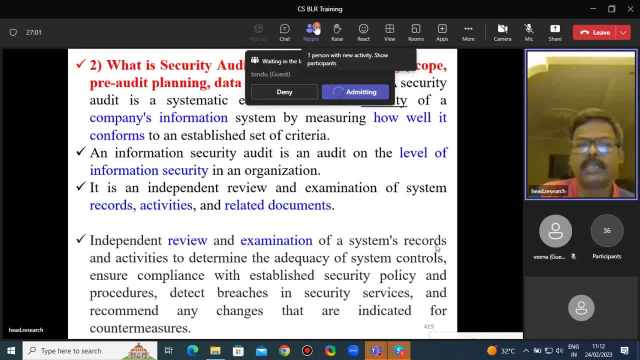 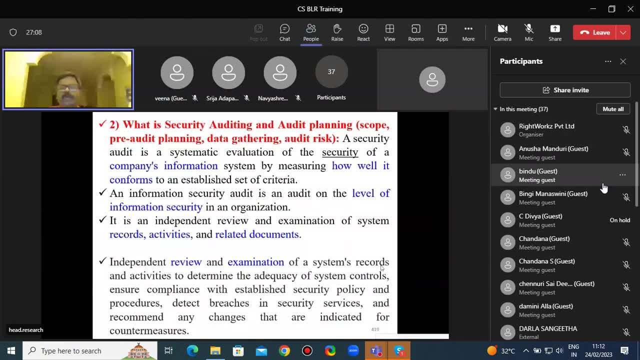 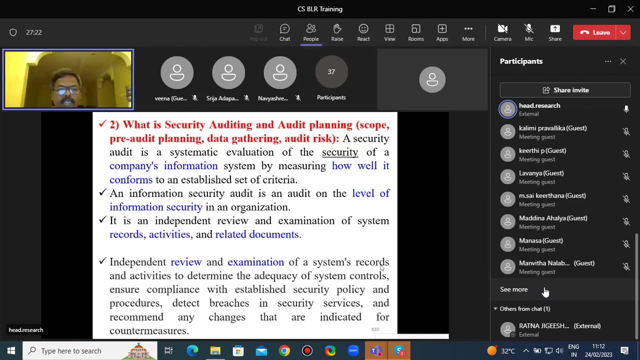 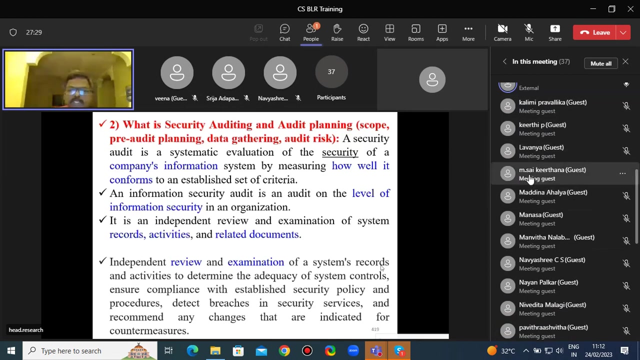 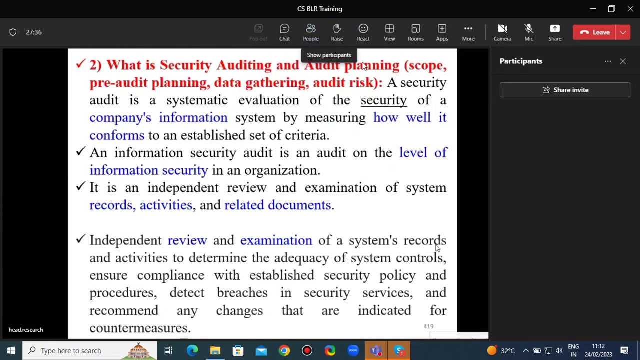 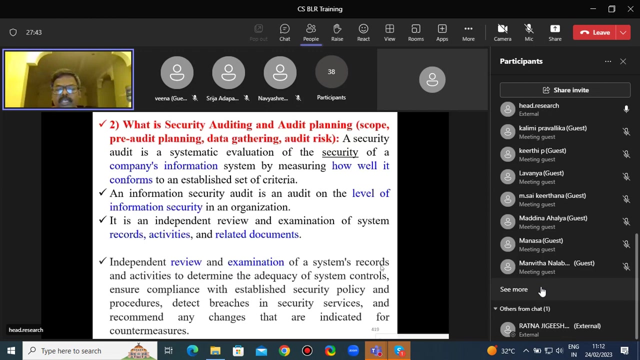 What are the major components they're implementing as information security? How well they're performing security auditing, assessing and evaluation in an organization? Maybe they're using CLA, trirhont and confidentiality. integrity and availability is an independent review Or examination of a system records. they are verifying documents, files, activities, employee policies, employee welfare and product of the quality and related documents. 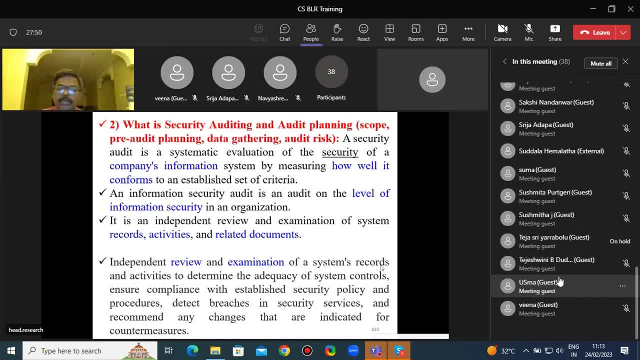 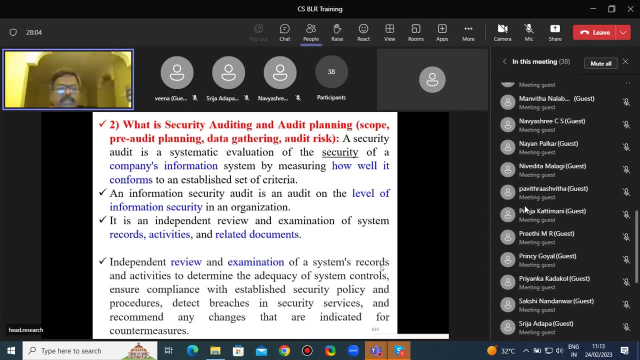 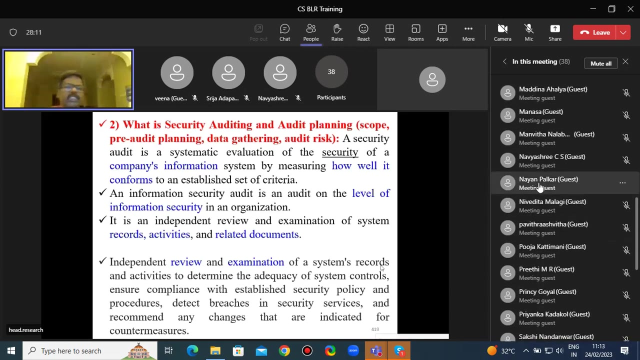 They are checking, they are reviewing, may be internal auditors or external auditors. So, even as an employee, I am checking yearly my audit of the income tax. I am paying income tax for the Indian government and I have one auditor who is going to assessing and evaluation of my annual salary. How do I do that? How much? Whether I am across, that is 30% of your monthly salary. That means, suppose you are taking per month 1 lakh, you need to pay 30,000 for tax for the government and 70% you are getting. 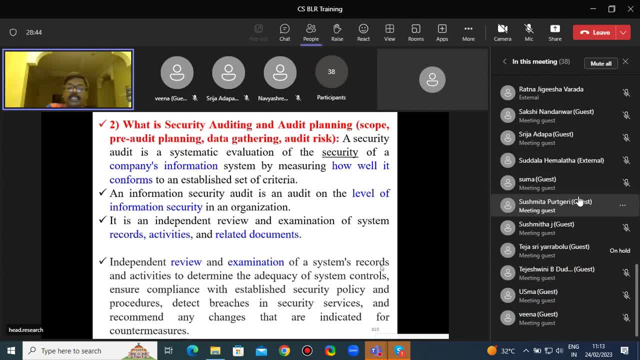 So: independent review and examination of a system records and activities To determine the adequacy of system controls. ensure compliance with the established security policy needs. any type of protocols and rules and regulations and procedures. detect breaches. You need to identify any activities: criminal activities happened or any attacks happened or any malicious activities. 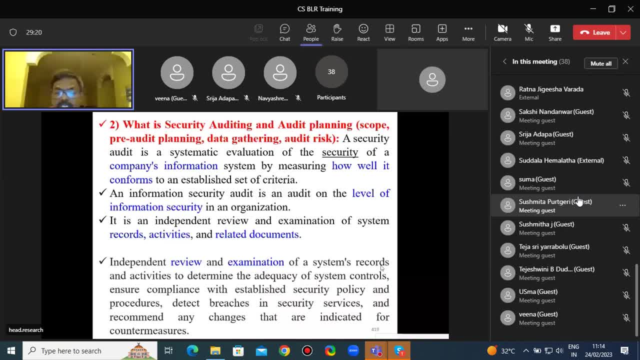 Activity happened in security services and they recommend any changes that are indicated for outer chaos. So that's why internal auditors or external auditors, are giving the reports at the end of the day, which consists of what type of attacks happened, breaches happened, malicious attacks happened-. 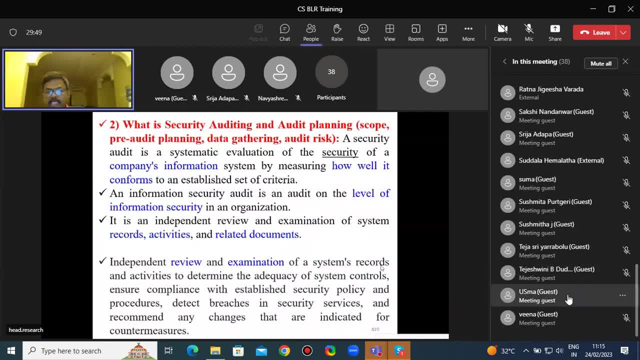 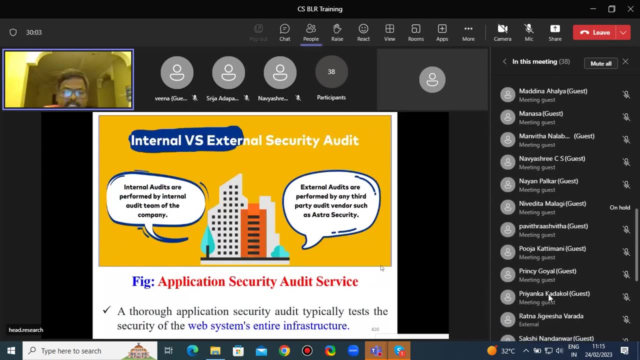 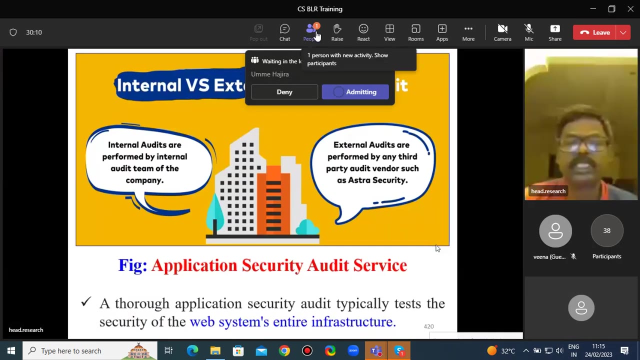 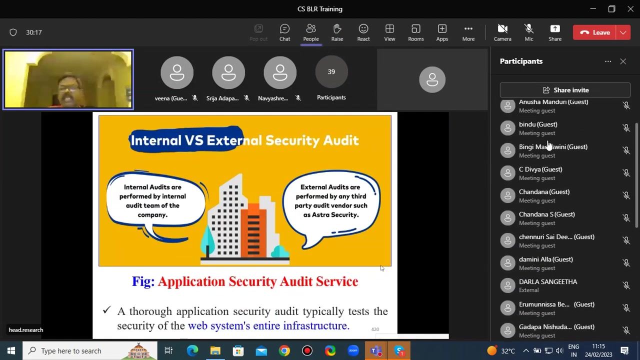 Presidential Jami besten Samman- Kamala, What type of security measures you are taking? They are giving recommendations and they are giving conclusions, observations of the organization. So see the difference between internal versus external security audit. But internal audits are performed by internal audit team of the company. External audits are performed by any third party audit vendor, such as Astros and JVP. 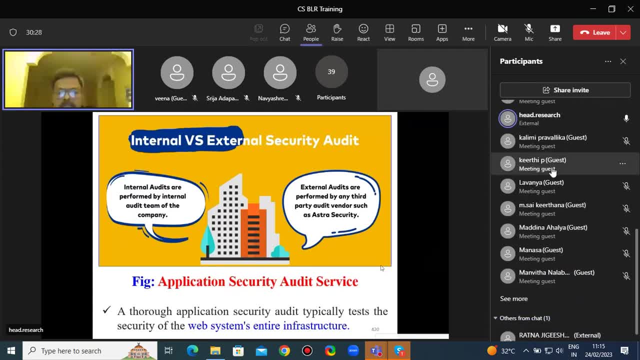 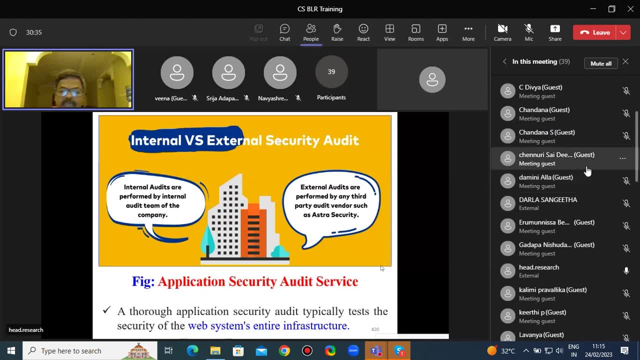 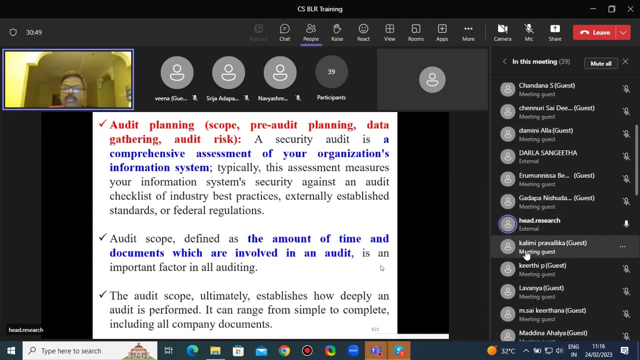 So a through application security update typically tests the security of the company, Security of the web system's entire infrastructure. So that is the difference between internal versus external security audit. So audit planning is nothing but a security audit is a comprehensive assessment of the organization's information system. 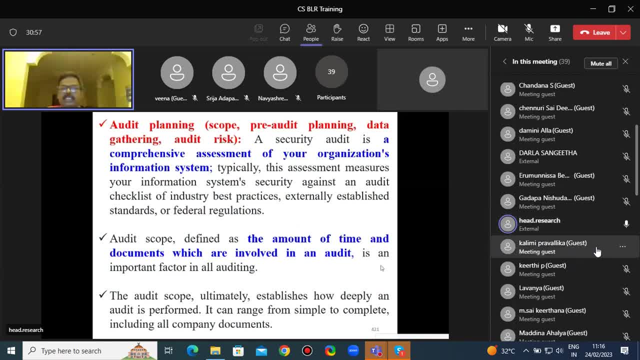 Typically, this assessment measures your information system security against an audit checklist Of industry best practices. Did you drop the mail? to our ma'am Standards? Yeah, did you drop the mail? It is gone. Okay then, Security of documents which are involved in an audit is an important factor in all audits. 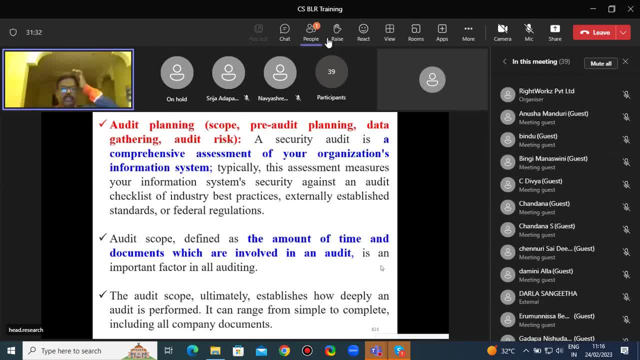 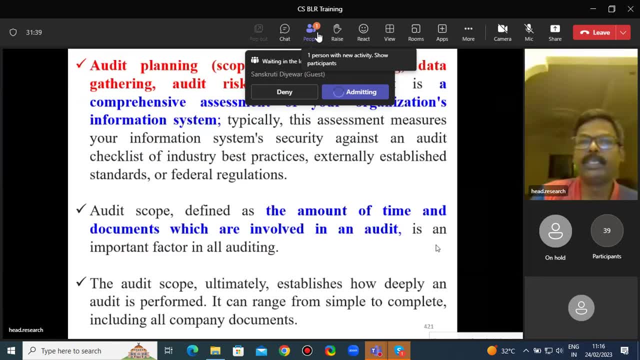 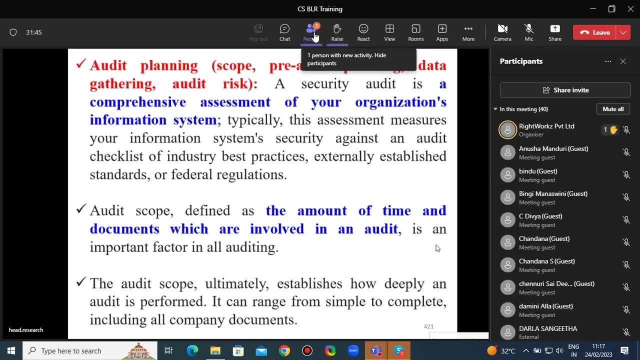 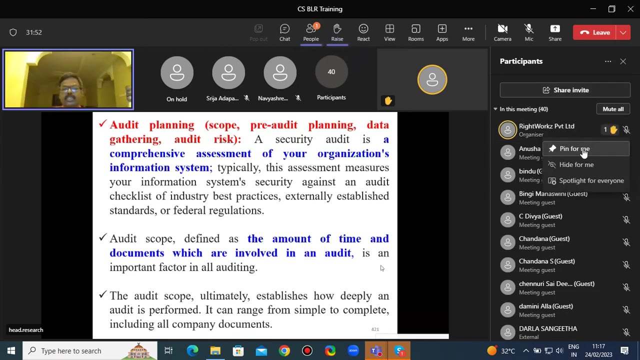 Audit team. So the audit team, The audit team. The audit scope ultimately establishes how deeply an audit is performed. Maybe external auditors, internal auditors? They are checking each and every record of the organization. Okay, So the audit scope ultimately establishes how deeply an audit is performed. 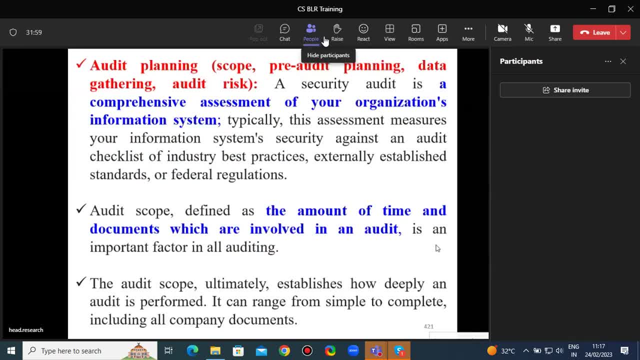 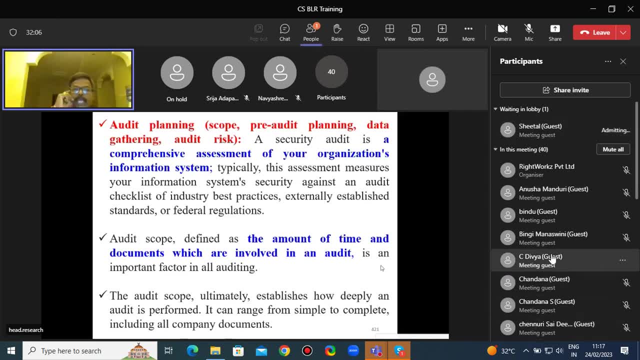 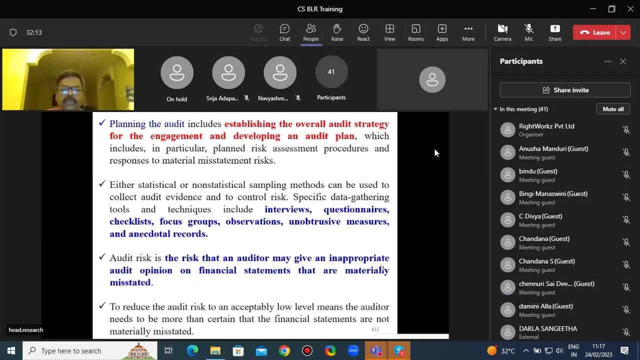 It can be range from simple to complete, including all company documents. That is called an audit scope. So planning the audit includes establishing the overall audit strategy for the engagement and developing an audit plan Which includes, in particular, planned risk assessment procedures or protocols and responses to materials misstatement uses. 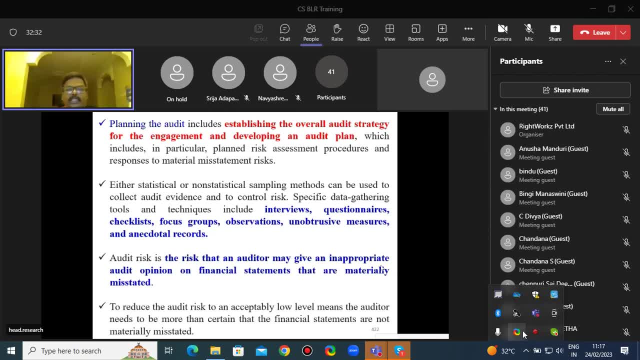 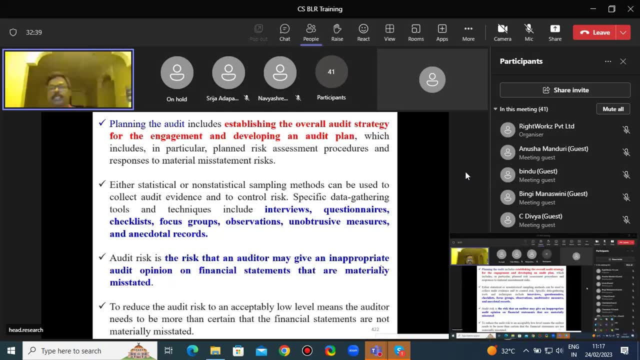 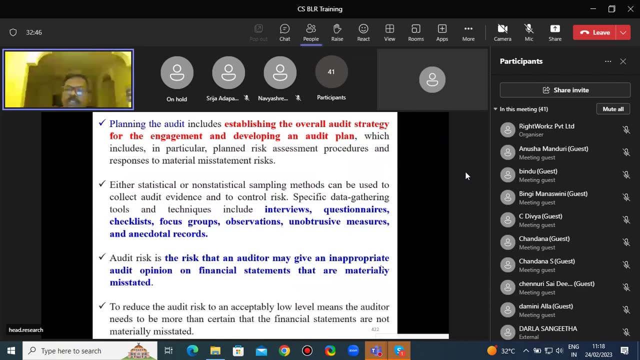 That is called a planning, the audit. Either statistical or non-statistical sampling methods can be used to collect audit evidence and to control risk. So specific data gathering tools and techniques include what they are doing, the internal and external auditors. They are conducting interviews, questionnaires, checklists. 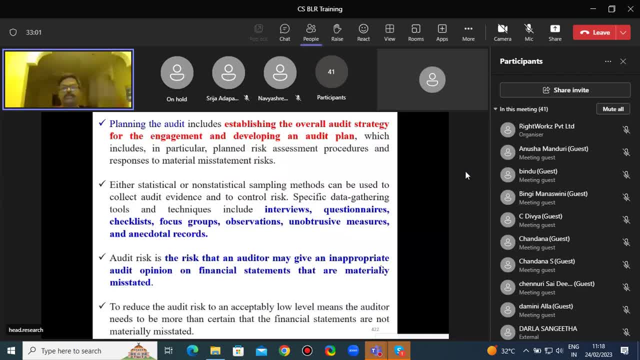 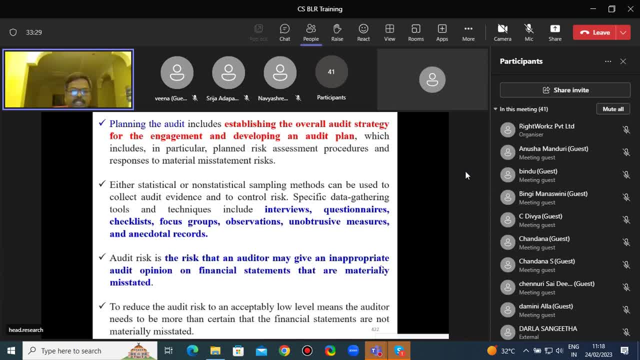 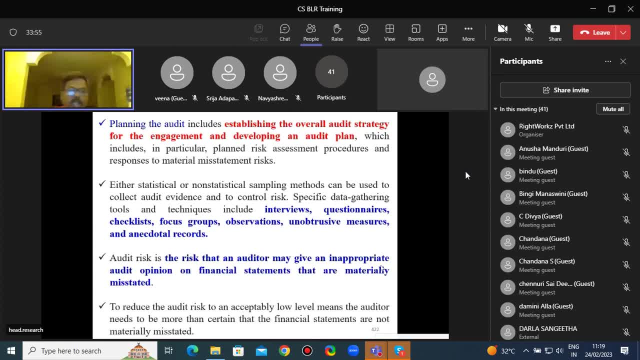 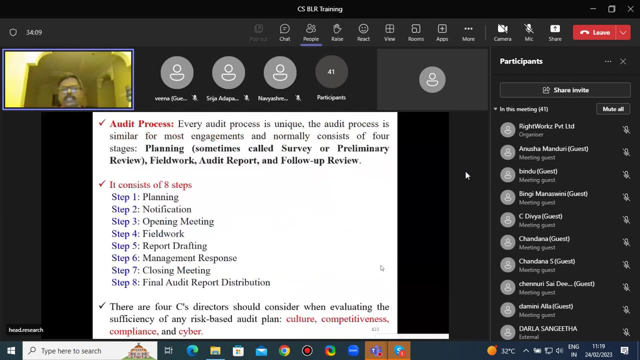 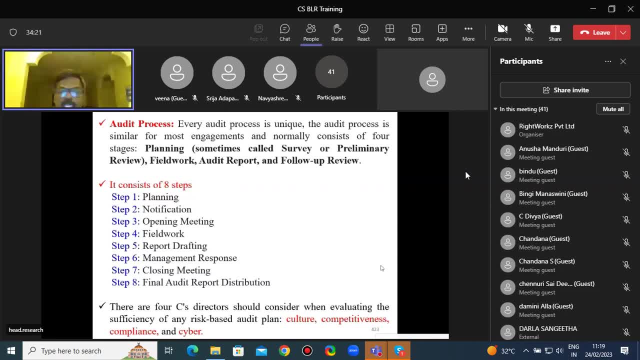 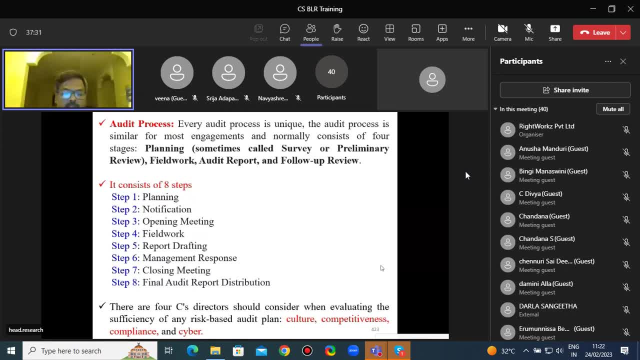 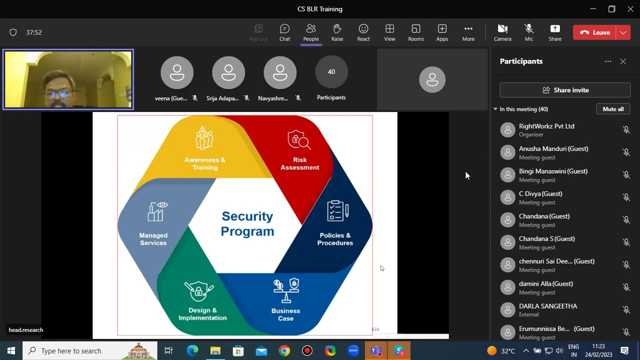 Cyber is a term or jargon of IT or virtual reality or augmented reality or related to computers. So for evaluating the sufficiency of any risk based audit plan, Then these are the important elements of security program. Security is nothing but protecting our company's information and policies, protocols, etc. 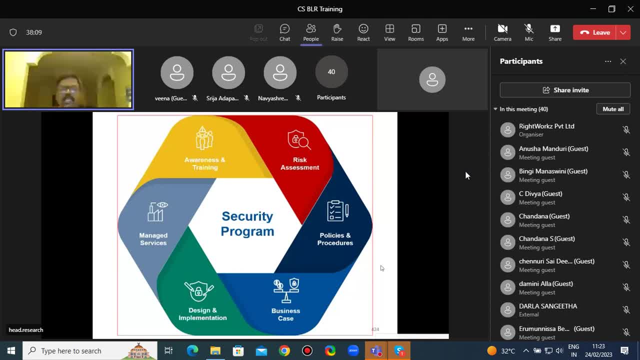 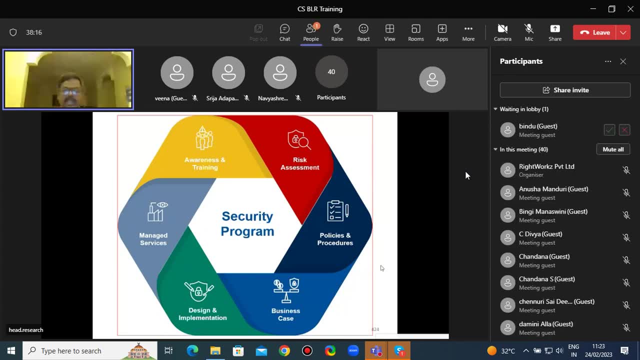 Program is nothing but collection of instructions or procedures, Rules and regulations. Security program is to do the training on awareness of organization's policies and protocols for assessing and evaluation of their product and employees in welfare. Then security program is assessing the risk assessment of the organization. 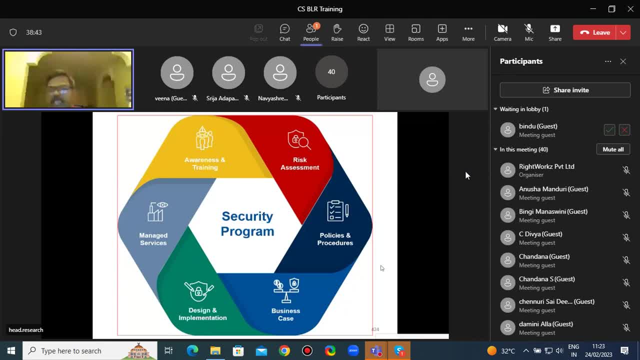 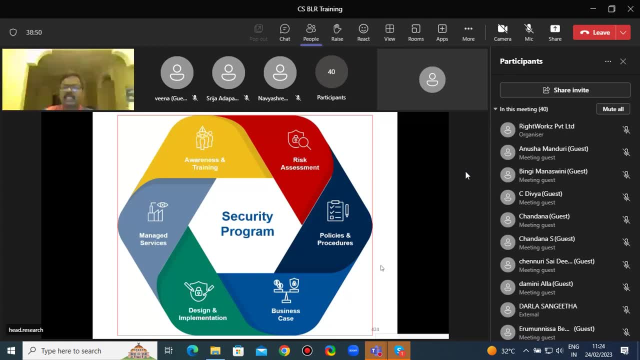 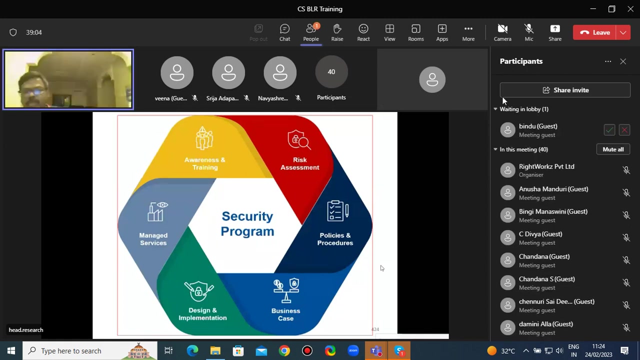 Then this security program conducts meetings and campaigns regarding policies and procedures to get the awareness of employees, existing people in the organization. This security program takes and performs business cases like projects, external projects, internal projects, etc. This security program is to design and implementation in order to perform assessment and evaluation of the organization's information. 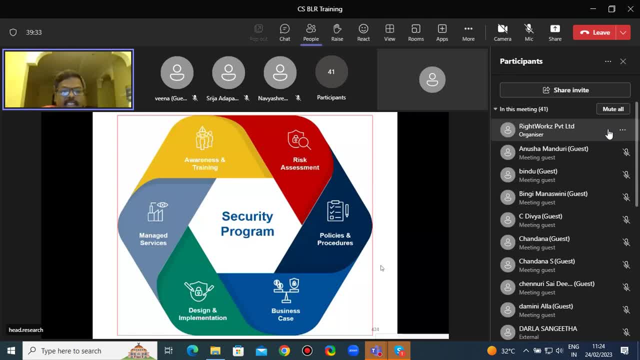 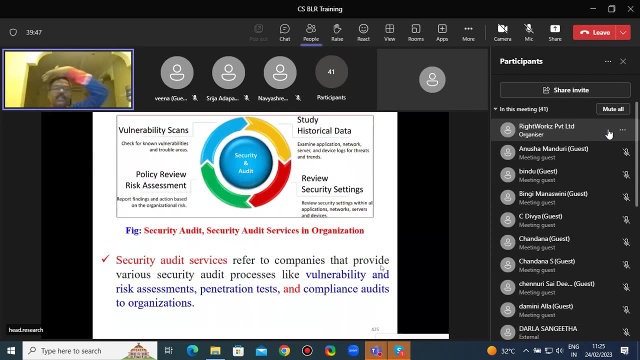 Then security program is managed services of the organization, So these are the major components of security program. Then if you see security audit services in an organization, So security audit services refers to companies that provide various security audit processes Like vulnerability assessment and risk assessment. 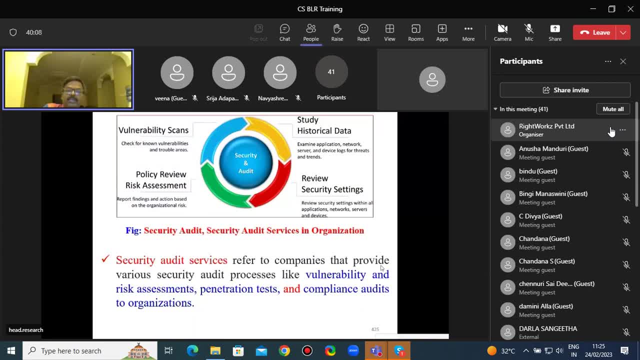 What type of attacks happened during 2021 to 2022. And penetration testing. They are checking how many threats, attack happened, incidents happened, breaches happened and compliance audits to organizations. If you see security and audit what they are going to do in security audit. 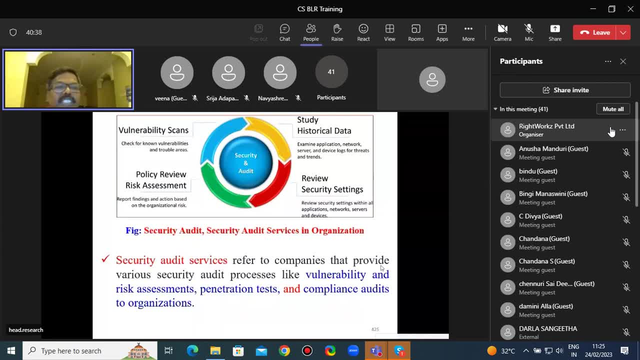 Vulnerability scans. It is nothing but check for no vulnerabilities, trouble areas They are checking for. any errors or root holes are there in the organization That is called vulnerability scans, Policy review, risk assessment? What type of protocol they have implemented? 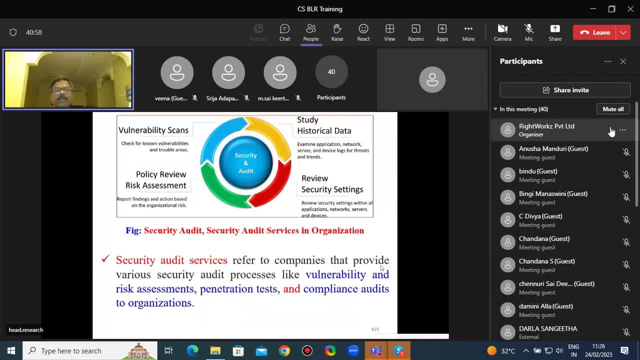 They have implemented and circulated among the employees. They are giving report, findings and action based on the organizational risk. That is called a policy review, risk assessment Study, historical data, That means so the legacy of the employees, Welfare or health services and rules. 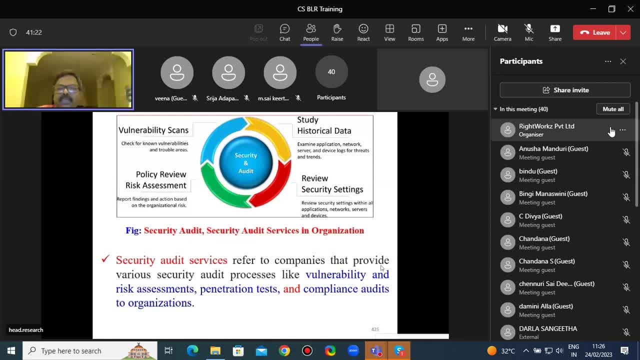 Examine application network server and devices And device logs for threats and threats. So study historical data concentrates how well this organization given best services past 10 years or more. They are checking those study historical data. Then the last one is reviews and security settings. 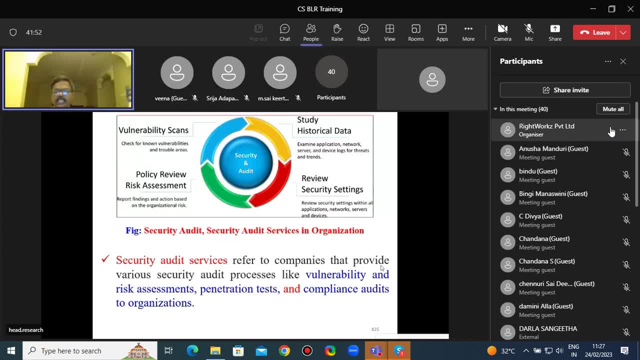 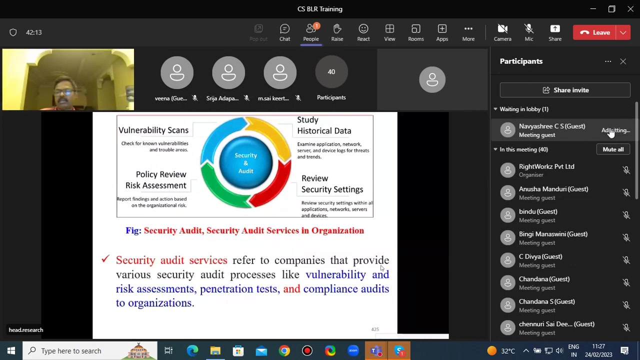 After visiting external auditors, internal auditors, They have given the excellent report of the organization And they are reviewing security settings, like within all applications, The networks and servers and devices. You need to use these many servers. These many employees are available. 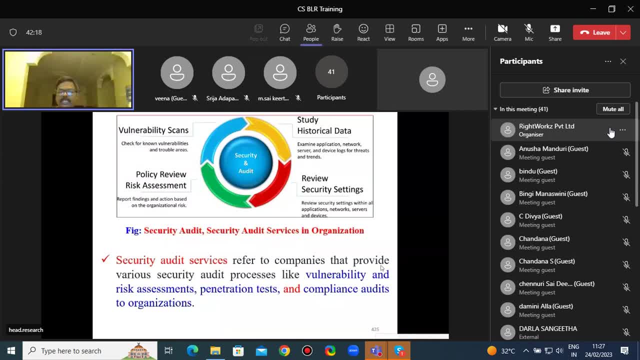 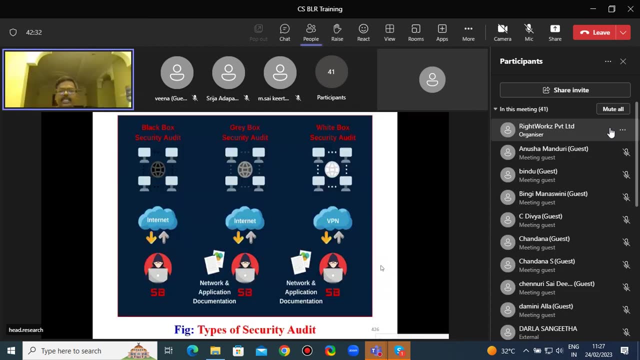 These many security holes and measures are there. You need to take counter measures In order to protect company's information, rules and regulations, protocols, etc. Then see the types of security audit: Usually black box security audit, grey box security audit, white box security audit. 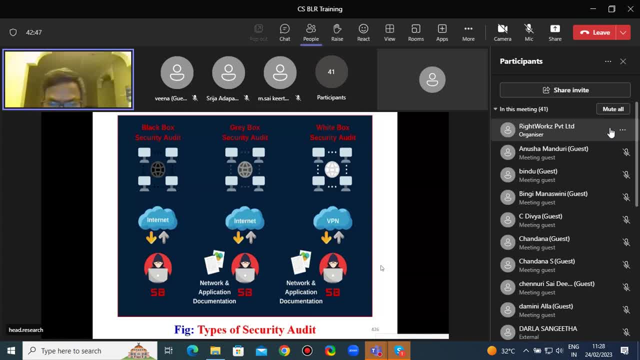 See: white box security audit is nothing but everybody knows who is coming For assessing and evaluation of the organization And black box security audit we don't know In the background level. they are checking, they are assessing and evaluation of the organization's information. 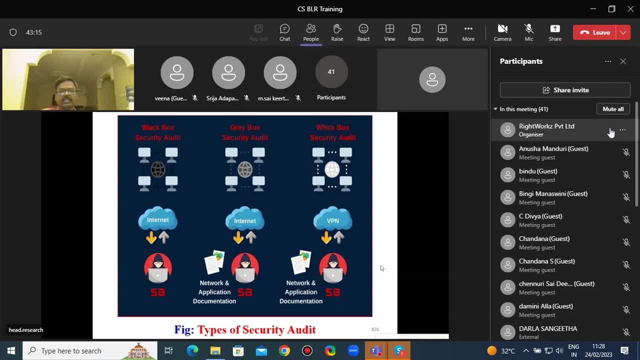 And welfare of the employee's information Through. they are doing a review Through. they are doing a review Through. they are doing a review. Any breaches or any security happen. Security incident And audits. malicious attacks happen. Any hacker attacking through internet in the background level. 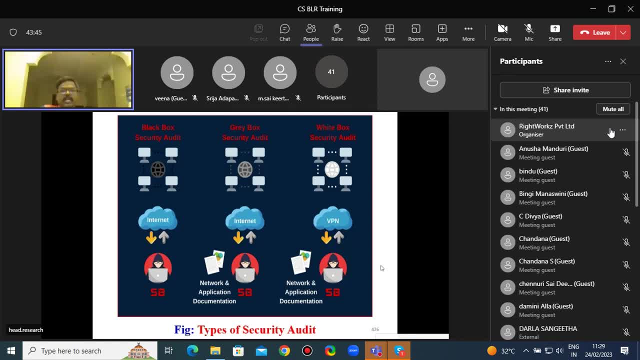 Such type of incidents are identified by the external or internal auditors. That comes under blockage. So you need to know this. security auditing, White box security auditing- we know when the external and internal auditors are coming to visit or through virtual private network, if any attacker entering into our 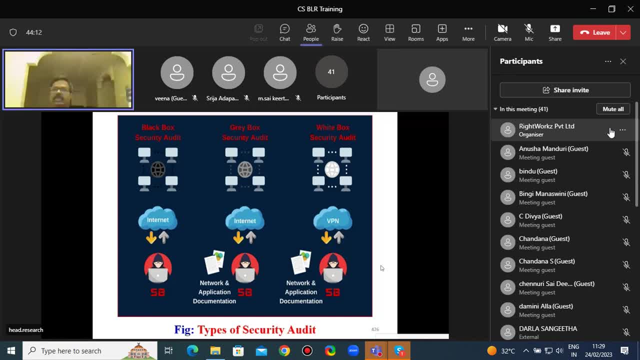 organization. so these people are identified through this virtual private network. So they are preparing network and application of our organization. Grey box security auditing is nothing but so 50% of black box security auditing groups and 50% of white box security auditing groups they are implementing in this grey box security auditing. These are 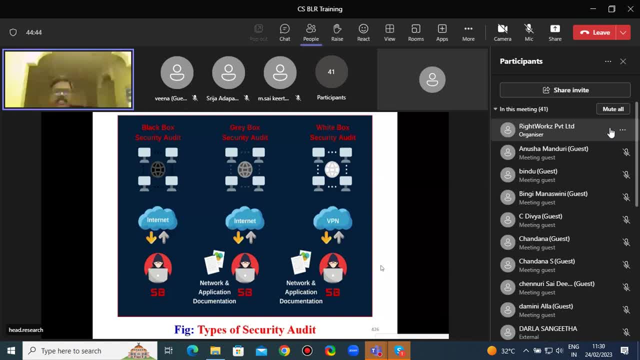 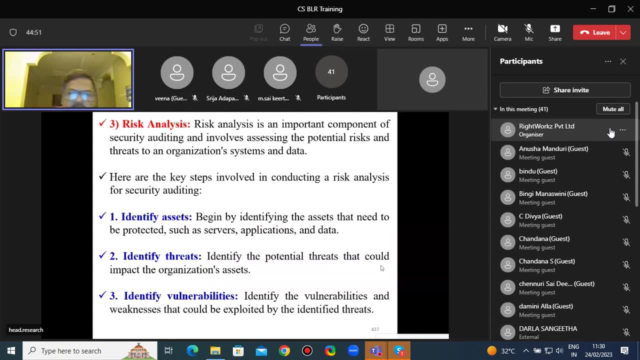 the types of security auditing. Then the third concept in today's security auditing, we will talk about risk analysis. Risk analysis is an important component of security auditing and involves assessing the potential risks and threats to an organization systems. and then here are the key steps involved in including conducting a risk analysis for security auditing. The first one is: identify assets. How many assets of the organizations? Begin with the data, By identifying the assets that need to be protected, such as servers, applications and data. So how many servers are at risk, Sometimes with viruses and malware attacks? 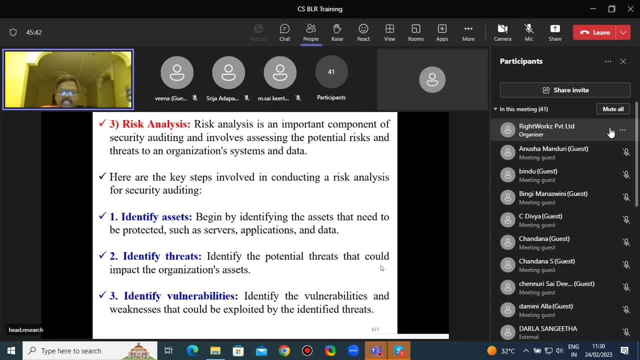 even our system says your system is at risk because of those malware, those viruses and attacks. So how many servers are at risk Sometimes with viruses and malware attacks? even our system says your system is at risk because of those malware attacks, some threats. 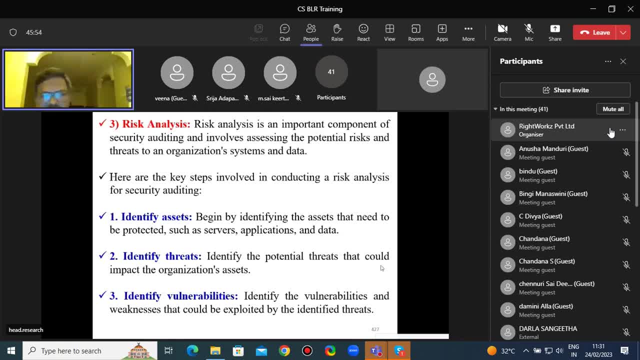 etc. Identify threats In risk analysis. why do we want to do risk analysis? We identify what types of potential risks and threats are there in the organization. So identify threats. we are identifying potential threats that could impact the organization's assets. Assets is nothing, but how many employees are there? How many employees are there? How? 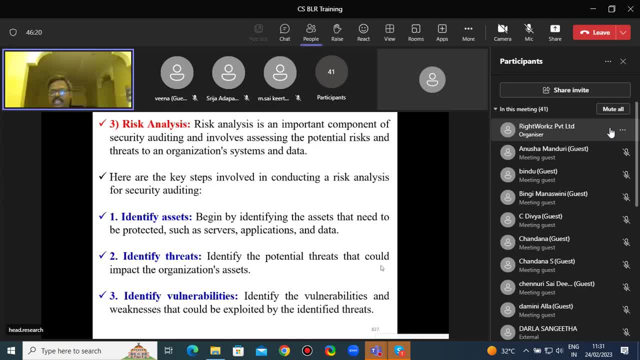 much infrastructure we are using And there are various assets of the organizations. Identify vulnerabilities. So in this risk analysis, we identify the vulnerabilities and the weaknesses that could be exploited by identifying threats. So what type of threats do we identify? We identify implicit vulnerabilities�, soient incidents. 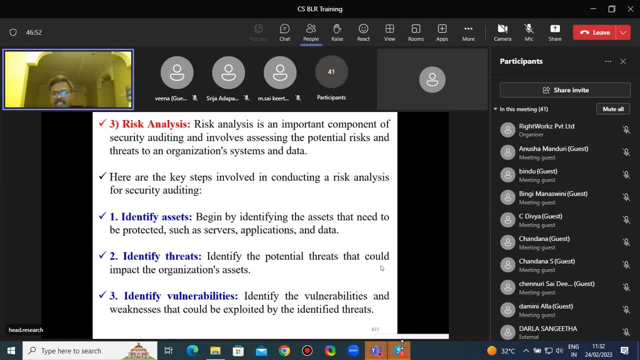 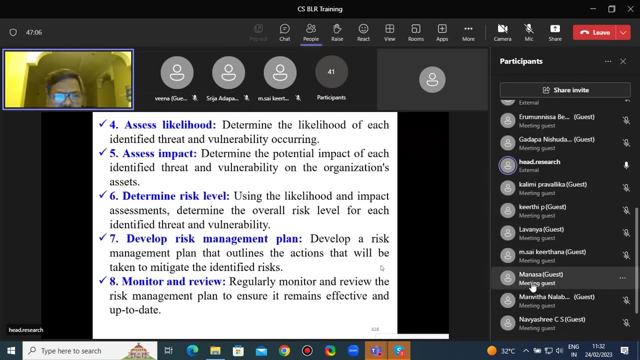 Cyber attacks, malicious attacks, safer malware attacks. meinen USD g methy portion calories, which is incidents, cyber attacks, malicious attacks, Threat or incident or breach is going to happen in the future. That is called assessing likelihood. Then assess impact, Determine the potential impact of each identified threat and vulnerability of the organization's assets. 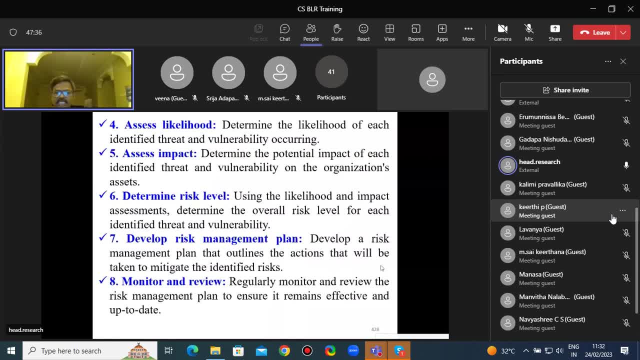 We are assessing the impact With this server. what type of online examination I can conduct With this data center. what type of project I can implement. That is called assessing impact. Determine risk level using the likelihood and impact assessment. Determine the overall risk level for each identified threat and vulnerability of the organization. 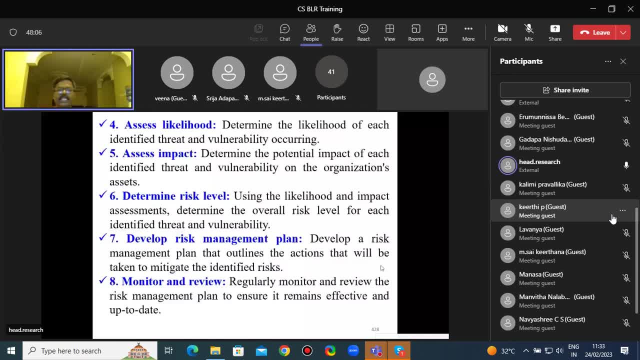 So we are identifying overall what type of risk has happened and for each identified threat and vulnerability. Then, seventh one is develop risk management plan. So, as a security auditor, you need to develop a risk management plan that outlines, that highlights the actions that will be taken to protect the organization. 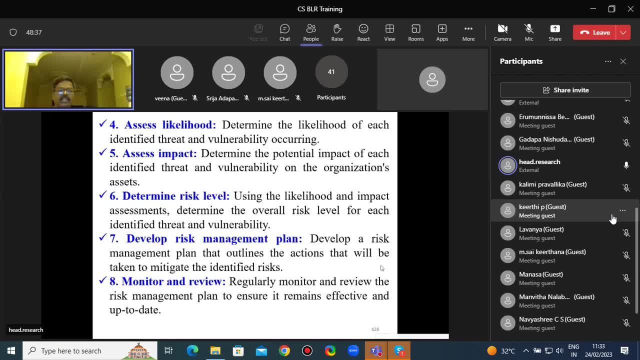 Then you need to develop and mitigate the identified risk. That is called a develop a risk management plan. The eighth one is monitoring. What is meant by monitoring and review? as a security auditor, Regularly monitor and review the risk management plan to show it remains effective and up to date. 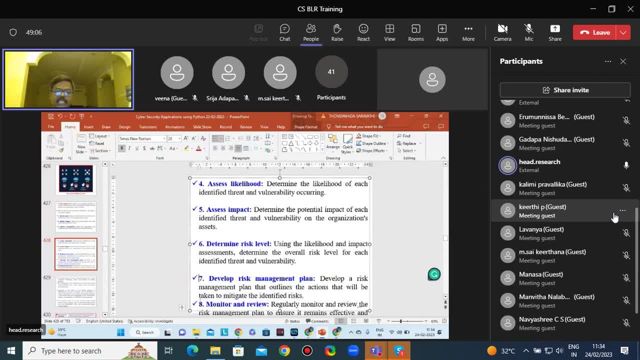 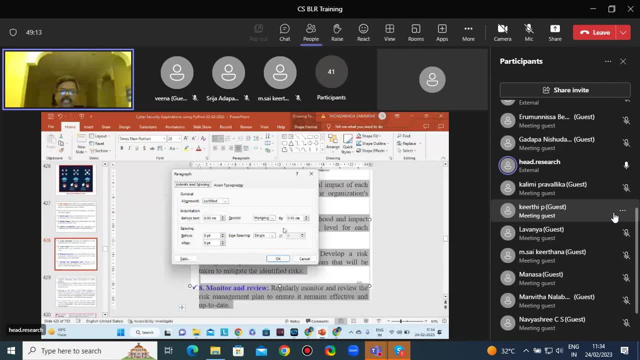 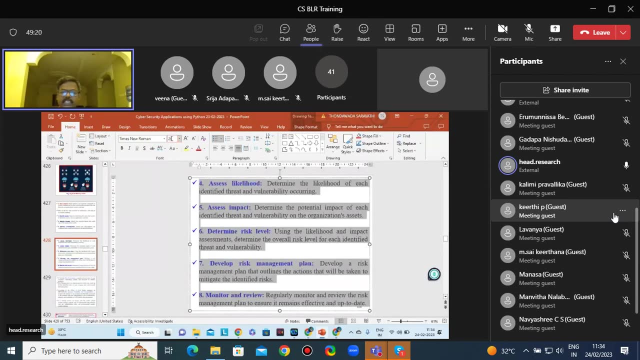 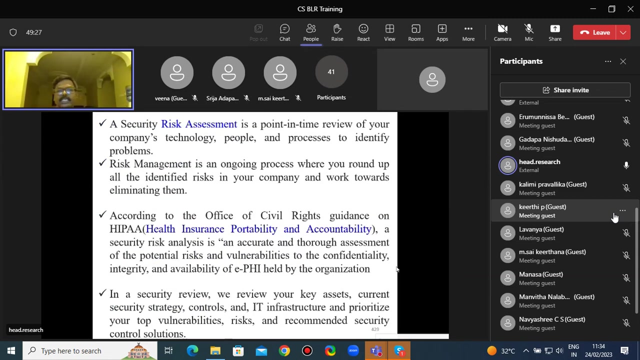 organization's assets and employees' welfare- everything I am checking and auditing and reviewing how best I can do for the organization by conducting this risk analysis. Then a security risk assessment is a point in time review of your company's technology, what type of technology you are using, how many people are working and processes to identify. 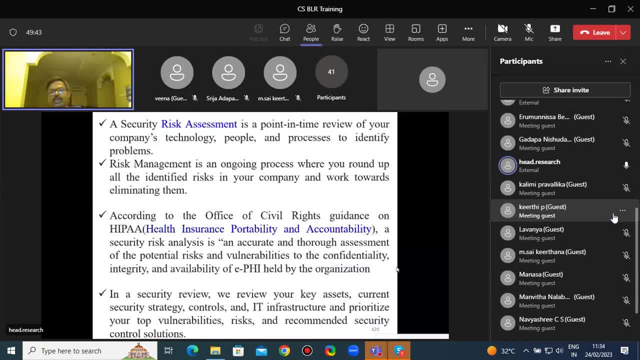 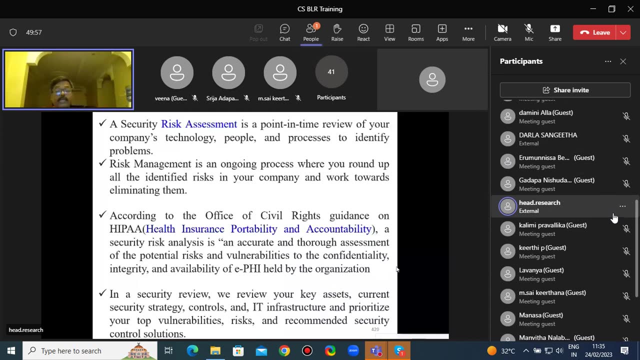 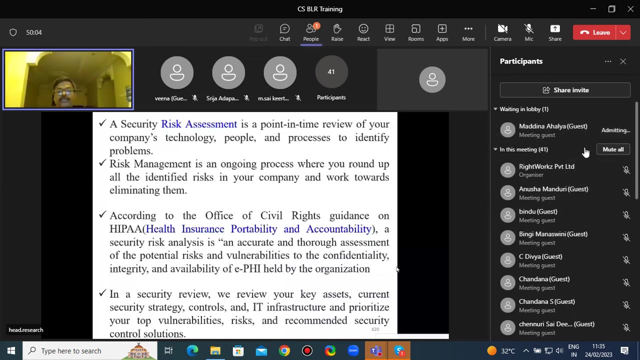 problems. what are the rules and regulations protocols using to identify problems? Risk management is an ongoing process where you round up all the identified risks in your company and work towards eliminating them. That is called risk management. According to the Office of Civil Rights Guidance on HIPAA, HIPAA is nothing but health insurance. 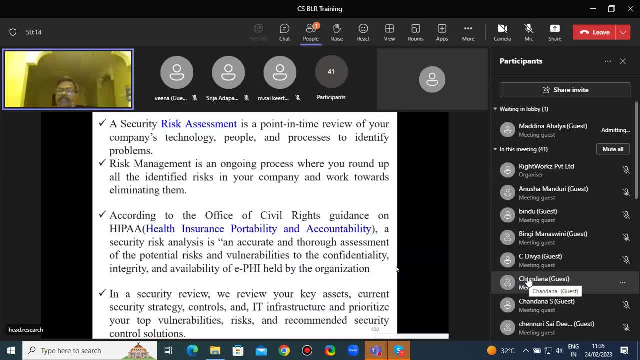 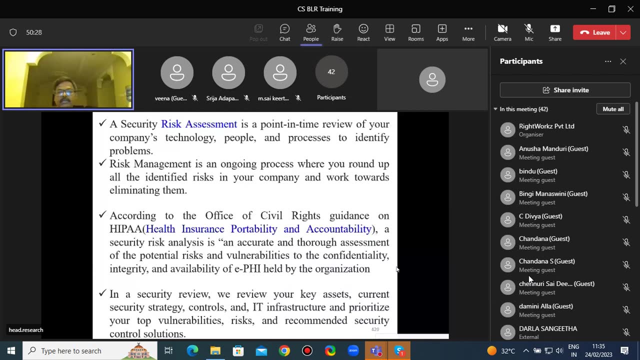 portability and accountability for every employee in an organization. they are doing group policy or health insurance policy, some insurance and a security analysis is ended. Accurate and thorough assessment of the potential risks and vulnerabilities to the confidentiality, integrity and availability of eBHI health by the organization. 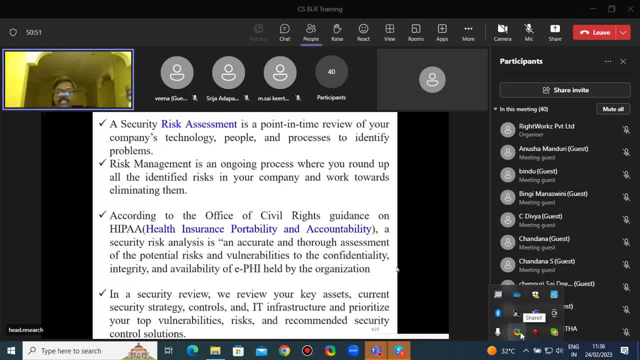 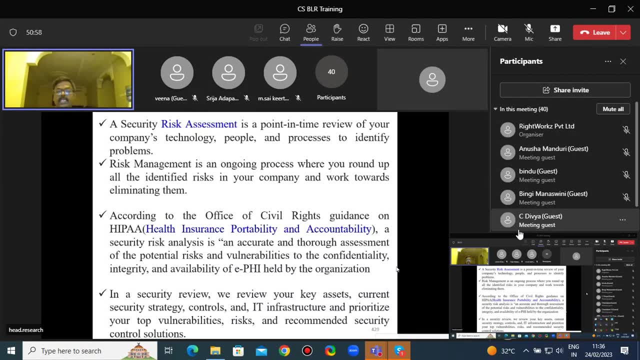 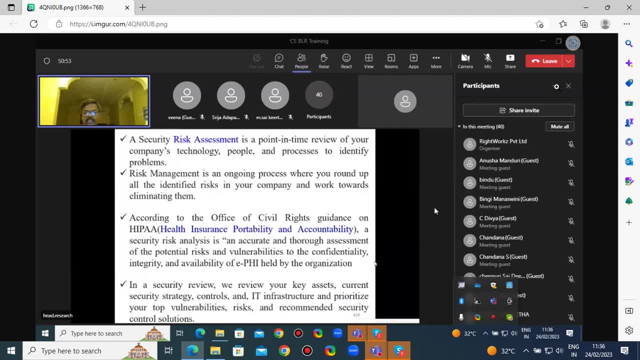 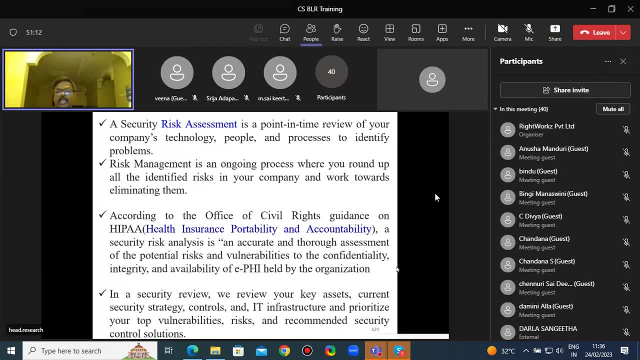 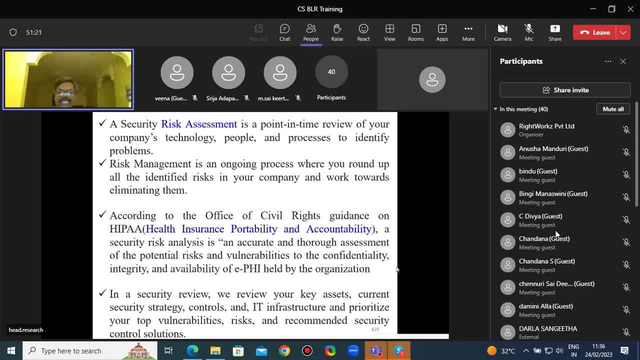 In a security review. we review your key assets, yes, organizations, infrastructure and current security strategy. what type of fire walls? what type of security system? what type of security technology? what type of security system? We review the security department. we review the organizations in force, function and the 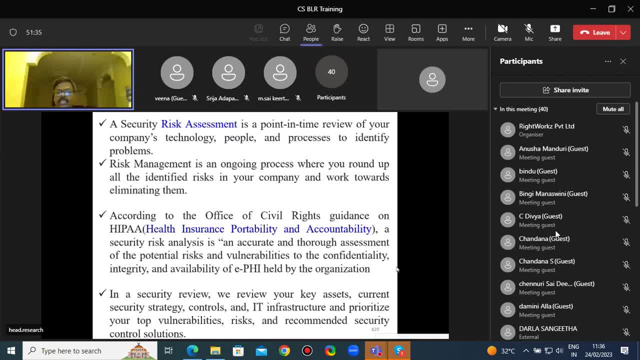 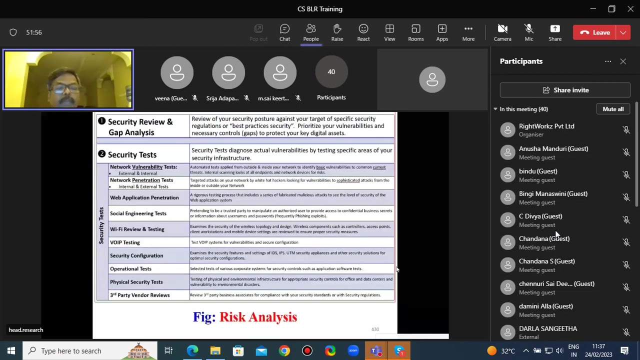 security measures you are using and controls and information technology infrastructure and prioritize your top, whatever it is, risks and recommended security solutions. you see risk analysis. there are two tests we are performing: major security review and a gap analysis. what we are doing in this security review and the gap analysis. 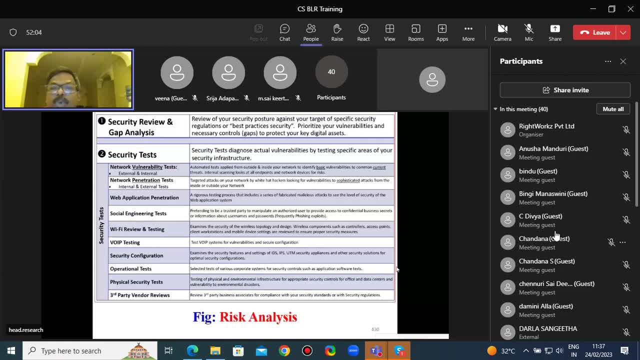 is see just a review of your security posture against your target of specific security regulations, which. what are? the protocols, best practices, security and prioritize your vulnerabilities and necessary controls. that means gaps. you are identifying gaps of the organization to protect your key digital assets and comes under security review and the gap analysis. 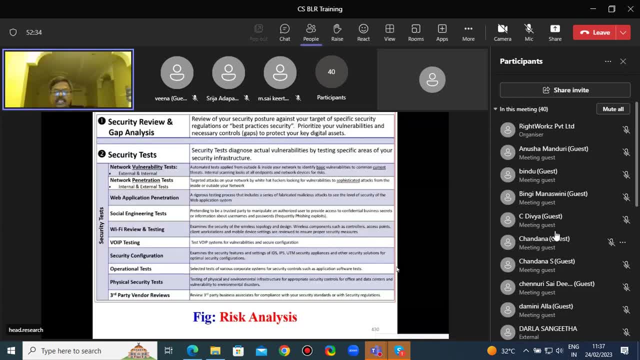 that's why, you see, the university is an organization. they are conducting bridge courses and bridge workshops and they are conducting the bridge gap between the university and industry. so what type of courses they need to study implement in the industrial level? they are including their industrial industry standard curriculum. 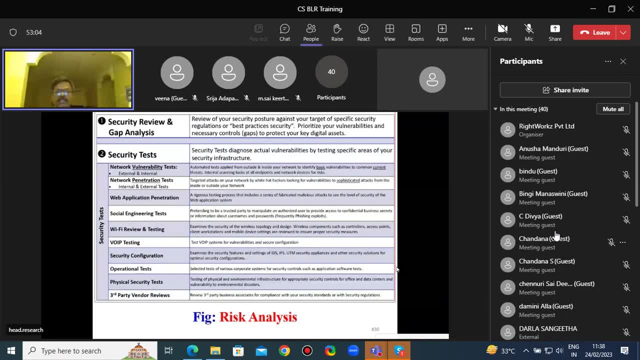 that is to fill the gap analysis between organization and the employees. that second one is security test. security test diagnose actual vulnerabilities by testing specific areas of your security infrastructure. it consists of network. vulnerability test may be external, so it automated test applies from outside and inside your network to identify basic vulnerabilities. 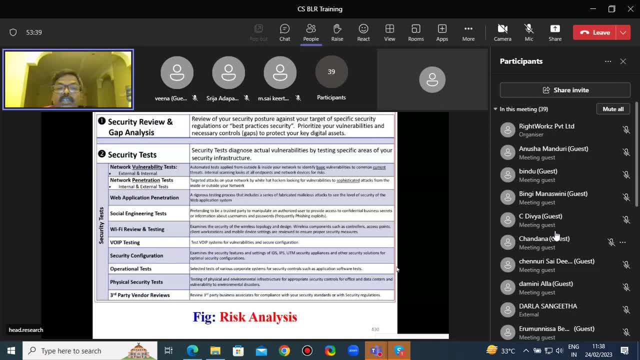 to common current threats. internal scanning looks at all endpoints and network devices. then network penetration tests what they are doing, internal and external tests, so targeted attacks on your network by white hat hackers looking for vulnerabilities to sophisticated attacks from the inside or outside of your network. then this security test consists of social engineering tests. so what is meant by social 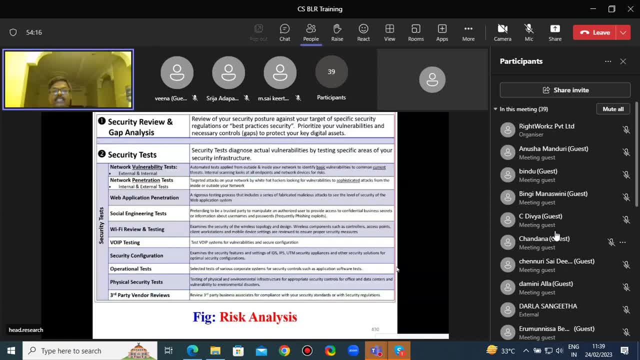 engineering, pretending to be a trusted party to manipulate and authorize the user to provide access to confidential business secrets or information about the username of passwords. that is called frequently phishing exploits. then the securities test covering the wi-fi review and testing. wi-fi is nothing but wireless virility. 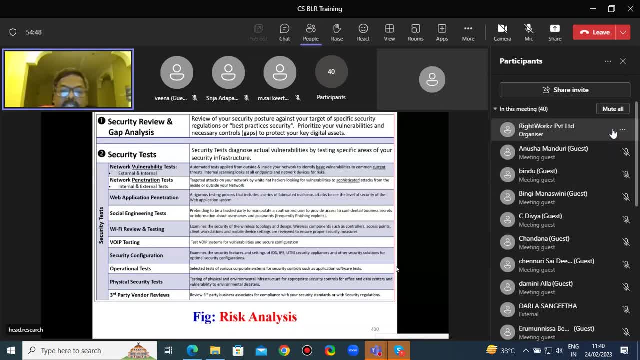 and what they are doing. examines the security of the wireless for policy and design wireless components such as controllers, access points, client workstations and mobile device settings, or review to ensure proper security measures. then security tests: performing voip testing wise over internet protocol. keep in mind, wise over internet protocol testing, what it is. 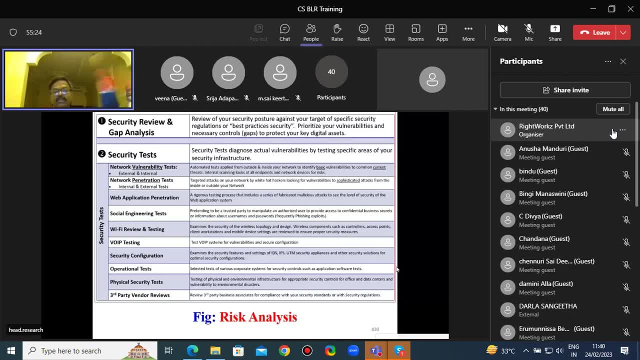 they are doing test system for vulnerabilities and secure configuration. see that means as a customer, as an employee, you would like to interact with the organization. how do you will interact? there is a toll-free number. so that the toll-free number comes under the ui testing. they are. 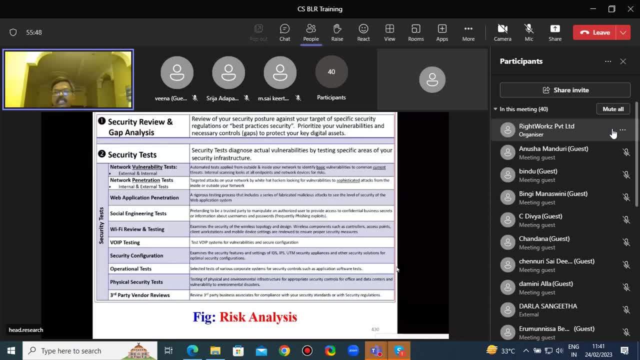 testing whether your organization toll-free number is working or not. so nowadays chart reports, replaced by that, voip candidates, usually we can call it as a bp receptionist, etc. security configuration is nothing but examines the security features and settings of ids, inclusion detection system, intrusion prevention system and ultimate test monitoring security appliances and other. 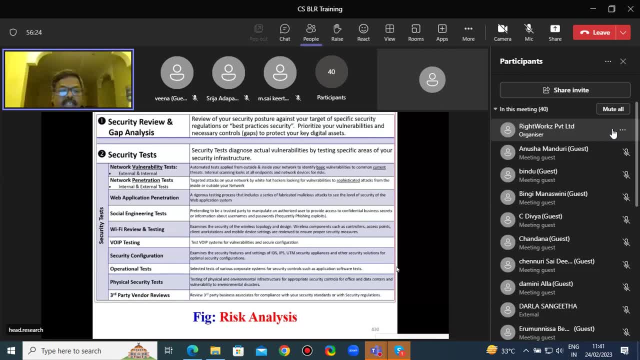 security solutions from the security configuration system. we can call it as a bp for receptionists: optimal security for patients. Then security test performs operational test. Selected test of various corporate systems for security controls, such as application software test, Physical security test, what they are going to do- Testing of physical and environmental infrastructure for appropriate security controls for office and data centers and vulnerability to environmental disasters. 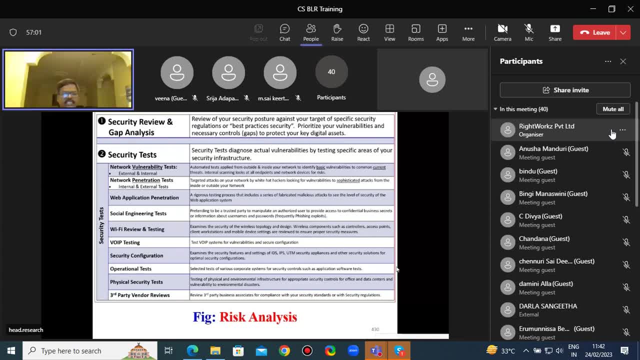 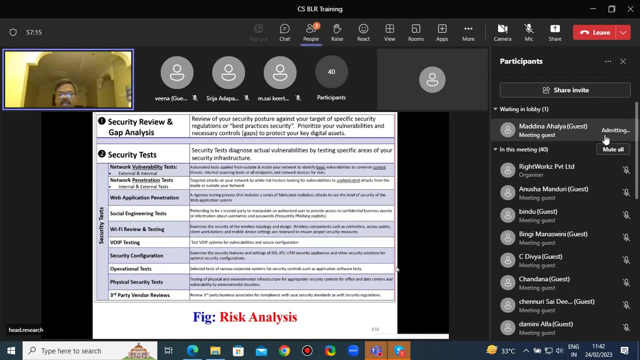 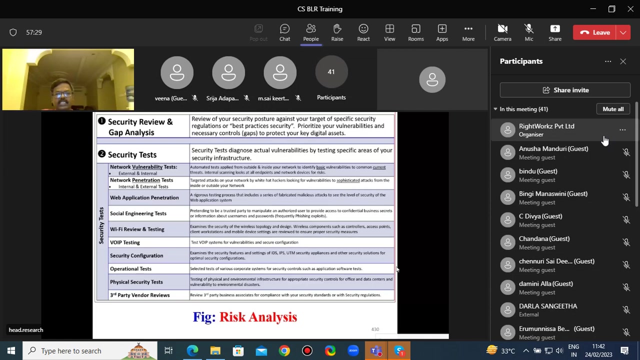 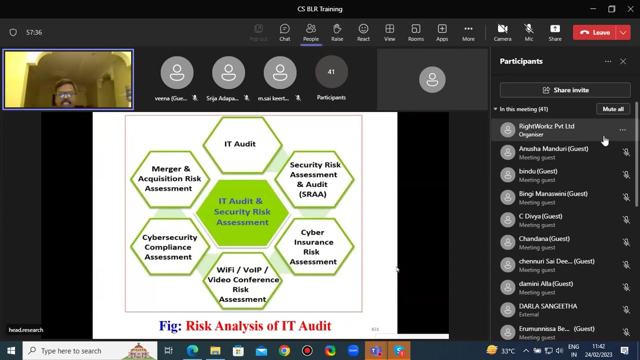 Then the last phase: third party vendor reviews. What they are going to do: review third party business associates For compliance with your security standards or with the security regulations. That is called a security test of third party vendor reviews. This is a comprehensive and complete description of risk analysis. So risk analysis of IT audit consists of: IT audit means information technology audit. 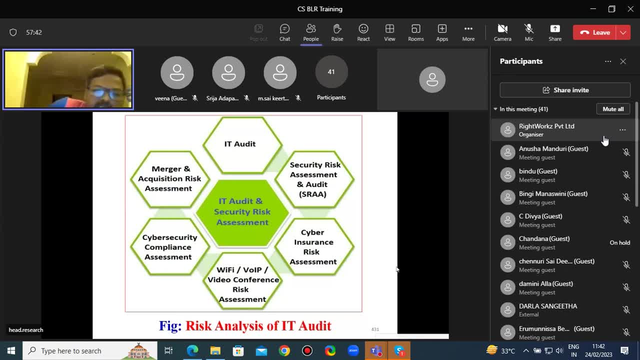 What type of technology you are using in the organization, and this IT audit and security risk assessment consists of security risk assessment and audit. that is called a strike- And they are assessing cyber insurance risk assessment- whether your organization is giving insurance related to cyber insurance risk assessment. 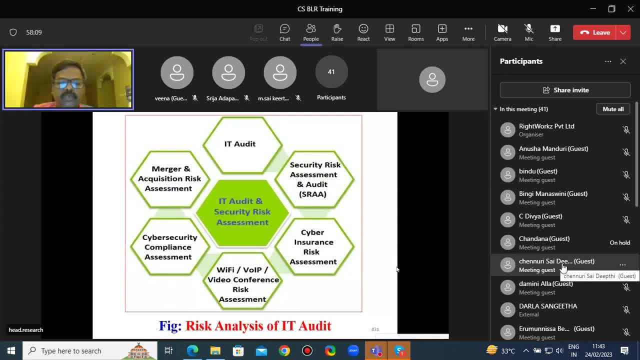 Whether your organization is following Wi-Fi, wireless connectivity related to internet and VOIP, voice over, internet protocol, video conference, risk assessment, etc. Then this IT audit and risk assessment: what security risk assessment? what they are doing, cyber security compliance assessment, what type of protocols you are implementing, what type of assessments you are using? 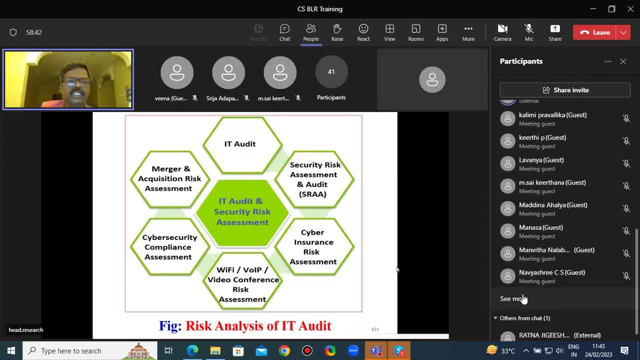 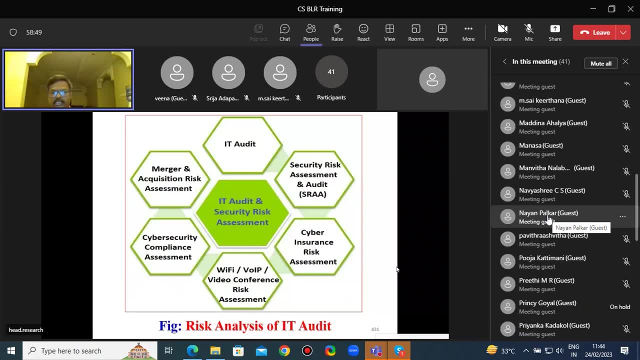 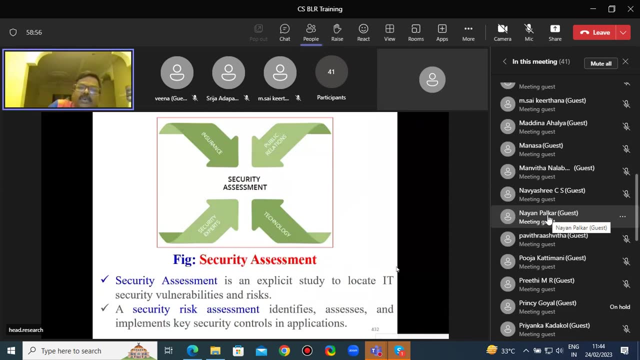 Then finally, merger and acquisition risk assessment- any combined rules you are using. This is about risk analysis of IT audit, Then security risk assessment. If you see, security assessment consists of what type of relations you are maintaining with the public and what type of technology you are using in the organization and what type of security experts are visiting to the organization in order to find out the loopholes, security measures and assessments. 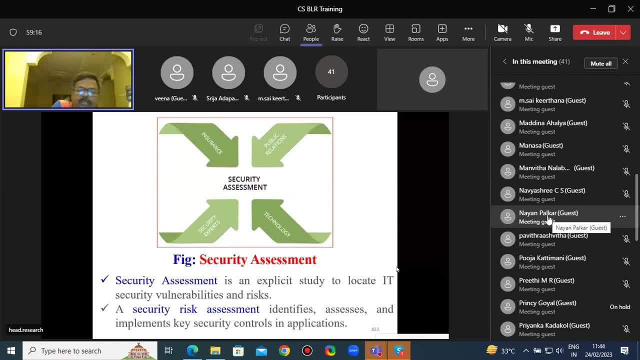 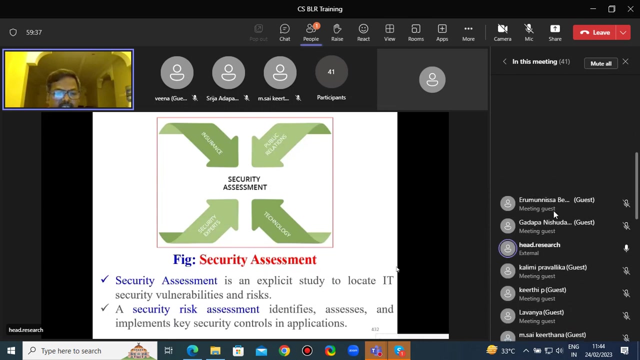 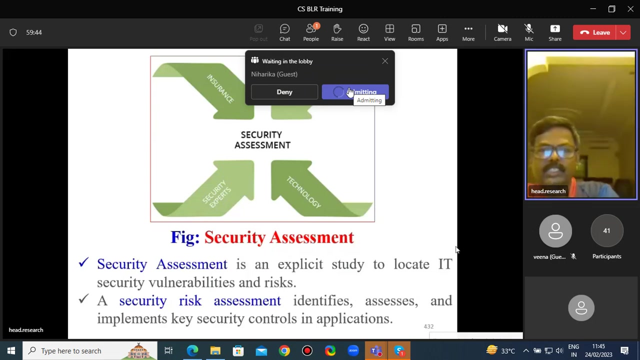 Then, finally, employees are having insurance or not. That comes under security assessment, Security assessment. Security assessment is an explicit study to locate IT security vulnerabilities and risks. A security risk assessment identifies, assesses and implements key security controls in applications. This is called a security assessment. 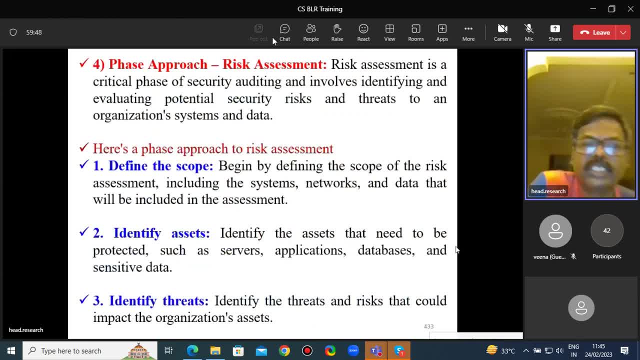 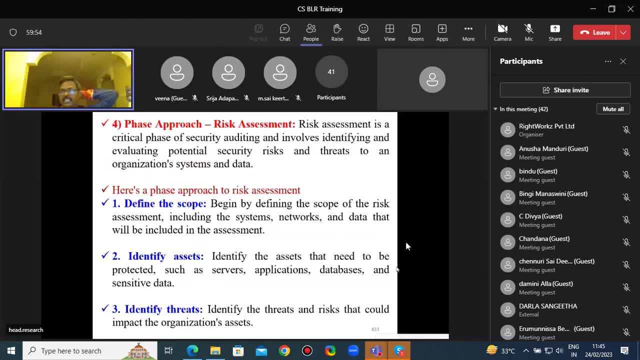 Then the fourth concept in this security audit is fail-safe, Fail-safe, Fail-safe. This is known as a face approach or risk assessment. Risk assessment is a critical phase of security audit and involves identifying and evaluating potential security risks and threats to an organization system's income. 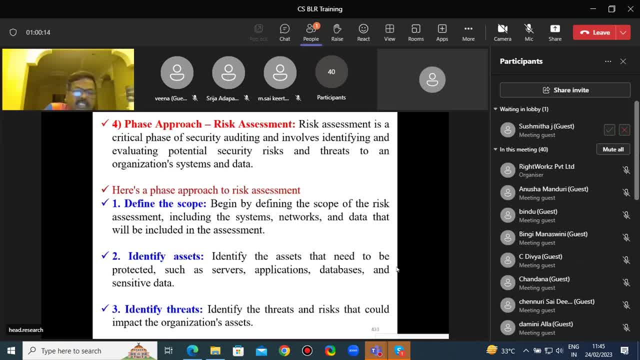 Here is a face approach to risk assessment. There are eight concepts are presented. One is define the scope. So begin by defining the scope of the risk assessment, including the systems, networks, servers, data center and data that will be included in the assessment. 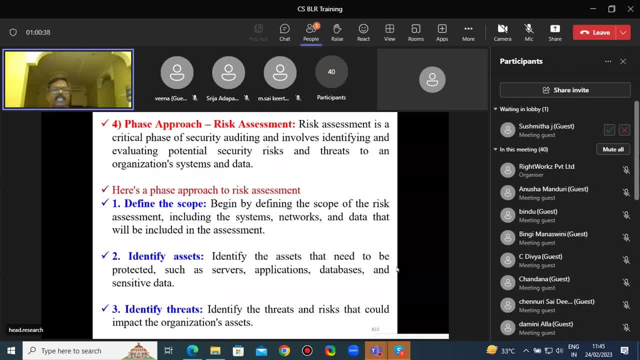 That is called define the scope. Then second one is phase approach is identify assets: Identify the assets that need to be protected, such as servers, applications, databases and sensitive data. Identify threats: Identify the threats and risks that could impact the organization's assets. Then, fourth one is assess vulnerabilities. 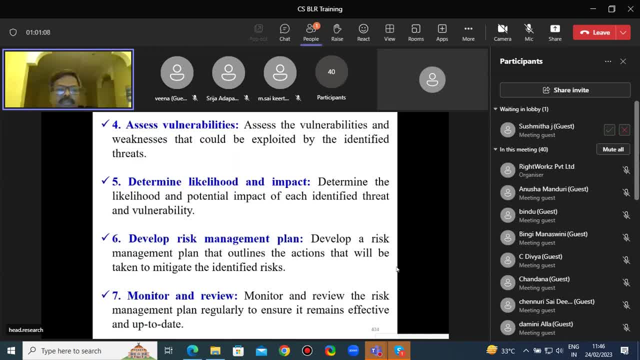 Assess the vulnerabilities and weaknesses that could be exploited by the identified threats. Determine likelihood and impact. Determine the likelihood and the potential impact of each identified threat and vulnerability. Develop risk management plan. Develop a risk management plan that outlines the actions that will be taken to mitigate the risk. 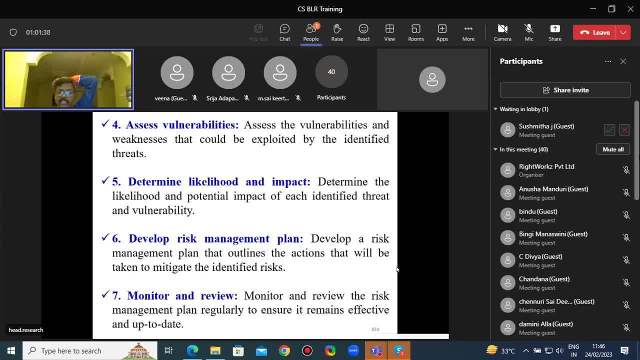 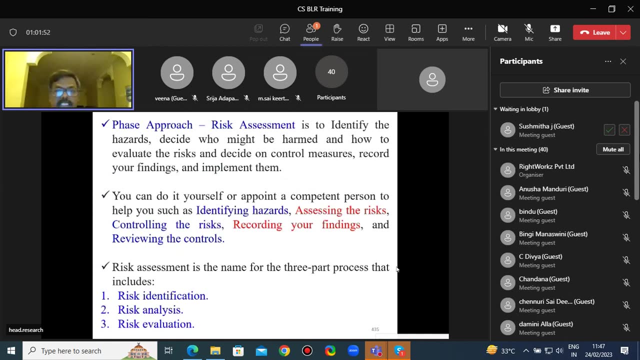 Investigate the identified risk. Then monitor and review The risk management plan regularly to ensure it remains effective and up to date. Then see the phase approach. risk assessment is to identify the hazards, decide how might be harmed and how to evaluate the risks and decide on control measures, record even findings. 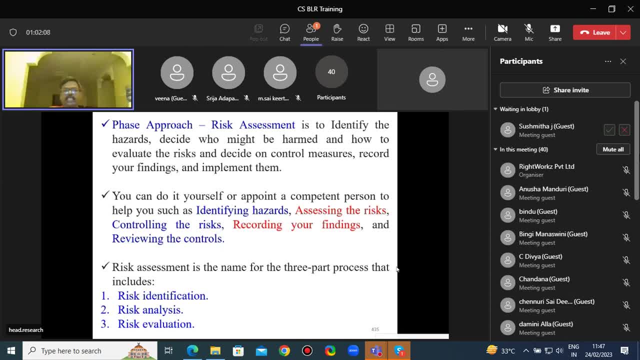 Then see the phase approach. risk assessment is to identify the hazards, decide how might be harmed and how to evaluate the risks and decide on control measures. record even findings. Then see the phase approach. risk assessment is to identify the hazards, decide how might be harmed and how to evaluate the risks and decide on control measures. record even findings. 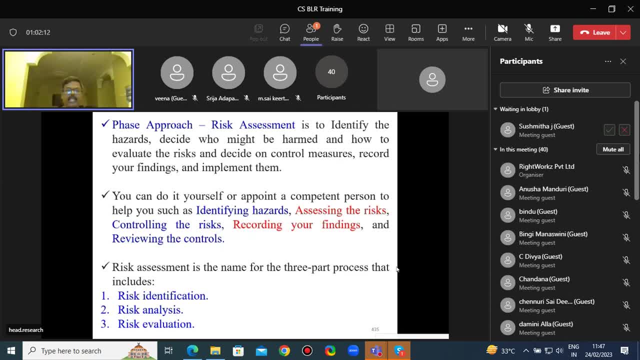 Then see the phase approach. risk assessment is to identify the hazards, decide how might be harmed and how to evaluate the risks and decide on control measures. record even findings. Then see the phase approach. risk assessment is to identify the hazards, decide how might be harmed and how to evaluate the risks and decide on control measures. record even findings. 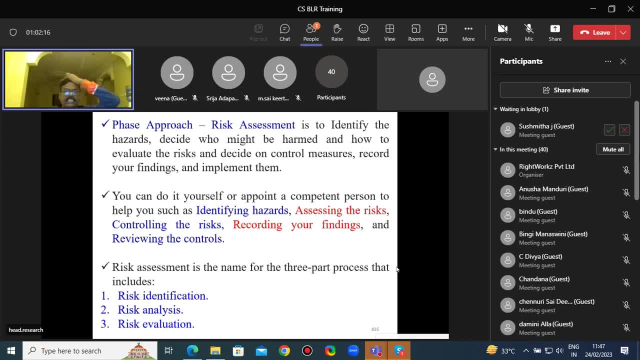 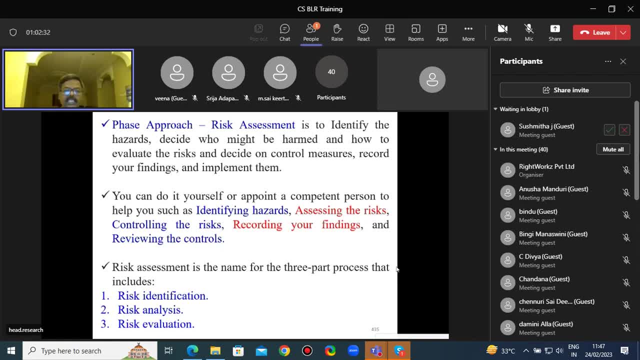 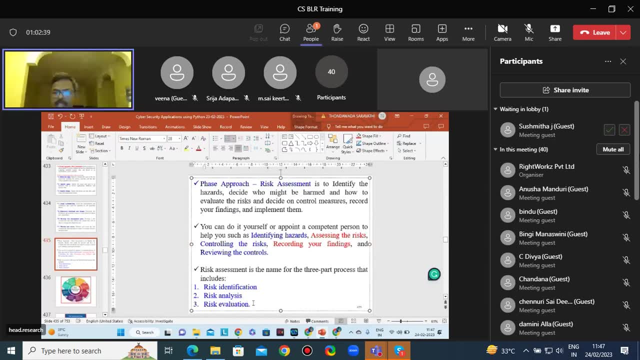 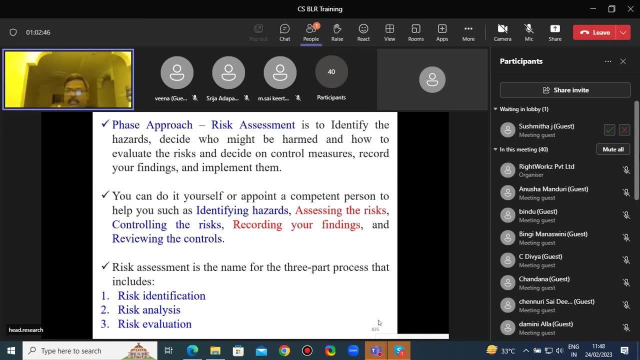 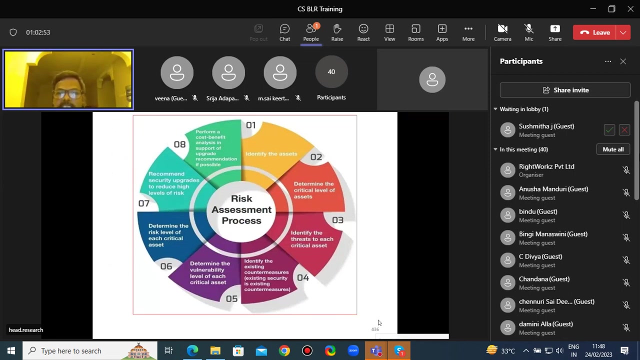 risk analysis and risk evaluation. So this is called a risk assessment, Then followed by the risk assessment process. There are 8 steps involved in the risk assessment process. The first step is identify the assets. may be hardware related infrastructure, software related infrastructure- that comes under identify the assets. The second one is determine the. 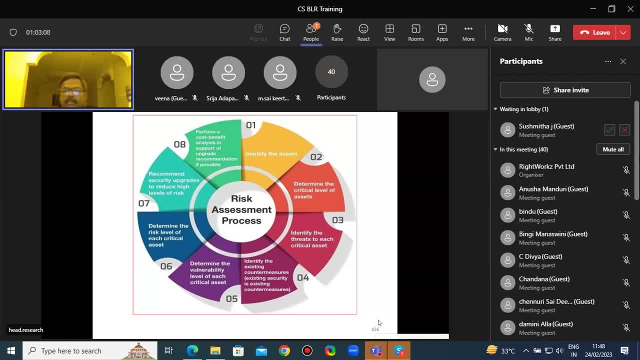 critical level of assets, what type of security roles are presented, what type of vulnerable attacks happen? Then, third one, identify the threats to each critical assets. Then identify the existing customer Countermeasures. that means existing security is existing countermeasures. Then determine 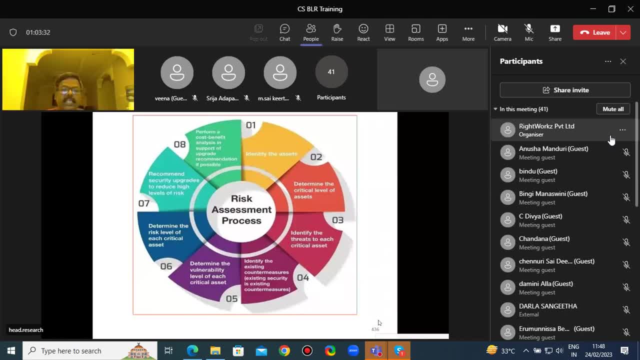 the vulnerability level of each critical asset. And sixth one is determine the risk level of each critical asset. And seventh one is recommended security upgrades to reduce high level of risk. And finally, perform a cost benefit analysis in support of upgrade recommendation and preservation if possible. These are the 8 risk assessment process steps or involved. 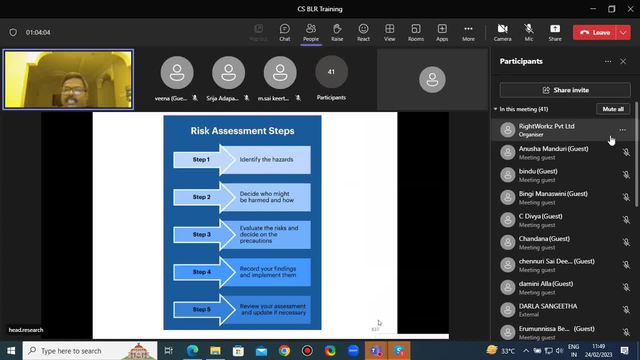 If you see risk assessment steps: step 1: identify the attacks needs: security incidents, cyber attacks, malicious attacks. step 2, decide who might be how and how that is comes another step 2, step 3: evaluate the risks. 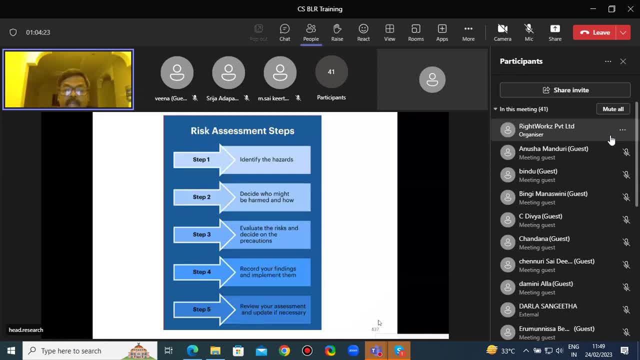 and decide who might be the risk target on the precautions from the organizations. Step 4, record your findings and implementation them. That is the fourth step of risk assessment. Then step 5, review your assessment and update if necessary. That is called risk assessment steps. Then 5 steps: approach in risk assessment. 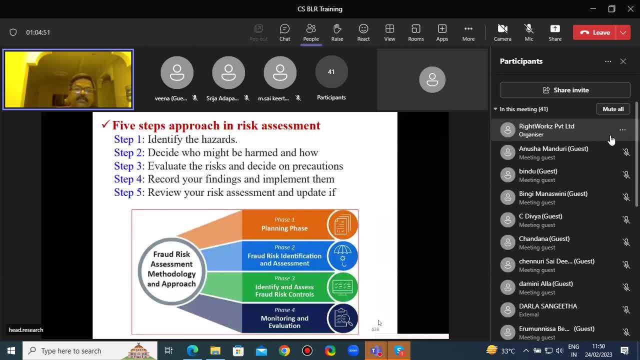 I have explained Once again. you can see: Step 1, identify the hazards. Step 2, decide who might be harmed and how. May be employees In employees- again, technical and non-technical- who might be harmed and how. Then step 3, evaluate the risks and decide on precautions. Step 4, record your findings and implement them as early as possible in the organization. Step 5, review your risk assessment and update if required. Then see the fraud risk assessment methodology and approach. So what is meant by fraud risk assessment methodology and approach? 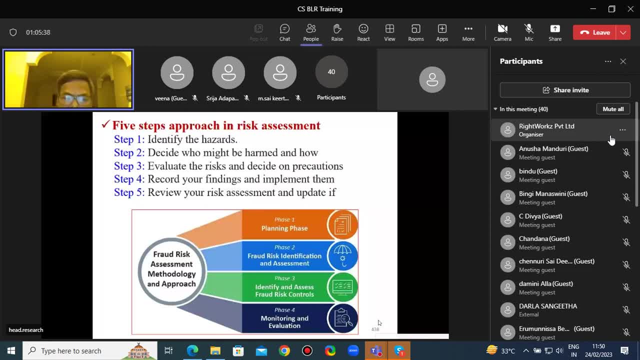 It happened during the last 6 months. So how do these phases are performing for fraud risk assessment methodology and approach? Phase 1, they are planning. Planning phase is called phase 1.. And phase 2, fraud risk identification and assessment. They are identifying what type of risk is happened. Phase 3, identify. 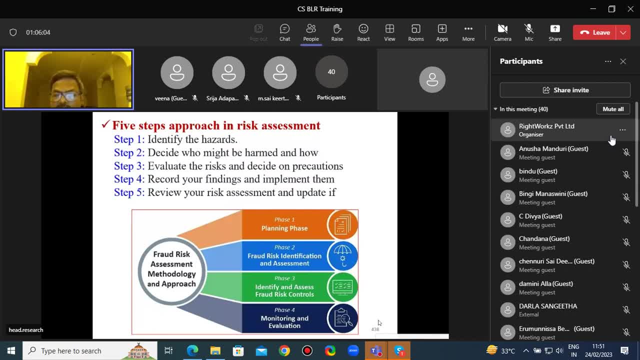 and assesses fraud risk controls, What type of control measures they are taking. Phase 4, monitoring and evaluation. Finally, they are checking through, online or offline, how many security incidents happened, How it happened, Which department the attack has happened. Everything we are monitoring and evaluation. 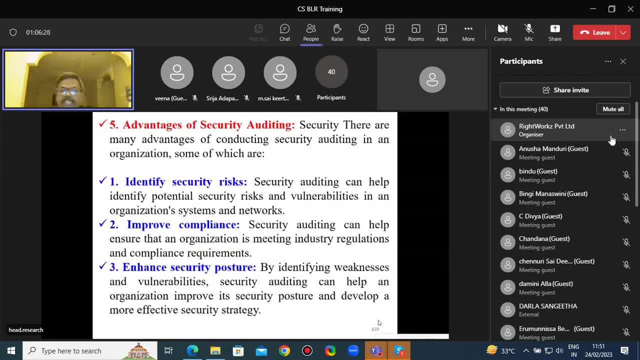 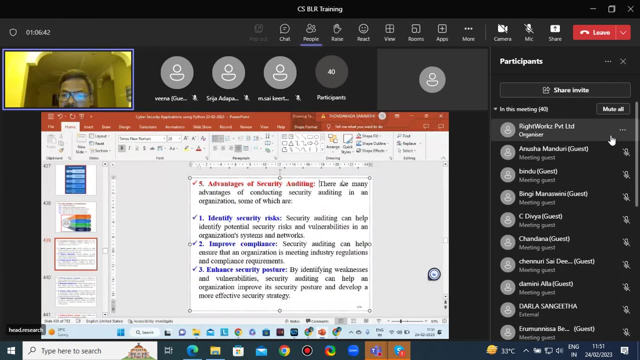 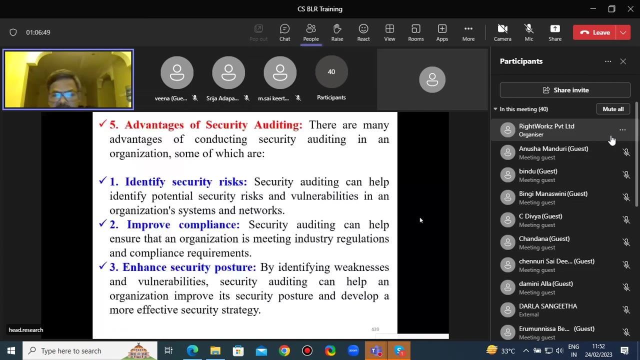 Then the fifth concept is advantages of security auditing. Security See. Advantages of security auditing is nothing, but there are advantages of conducting security auditing in an organization, some of which are identify security risks. that is one of the advantages. What they are going to do, Security auditing can help identify potential security risks and vulnerabilities or attacks or malicious attacks or any incidents or criminal breaches activities, criminal activities, vulnerabilities in an organization, systems and networks. 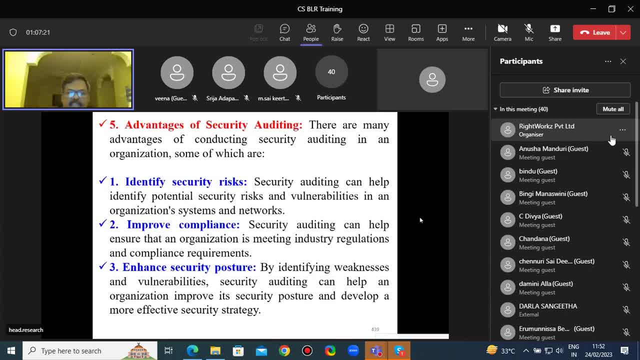 That is the first advantage. The second advantage is improve compliance. Security auditing can help ensure that an organization is meeting industry regulations and compliance requirements. It is based on the industry standard. you are getting salary or not, So that is one more. improve compliance of the employee of organization. 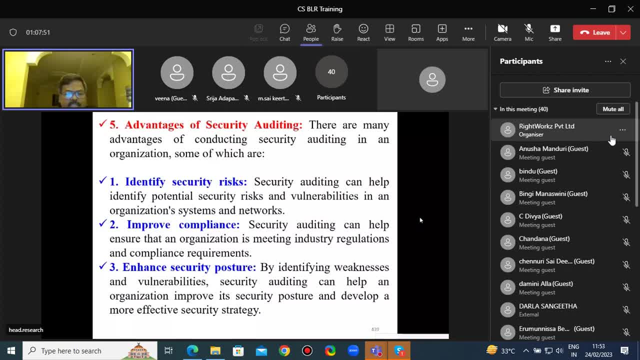 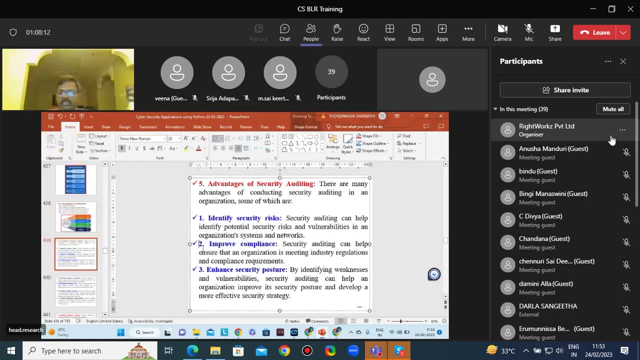 Then third one is enhance security portion. By identifying weaknesses and vulnerabilities, security auditing can help an organization improve its security portion, develop a more effective security strategy. That is called enhance security portion, So that is called. you can call it as advanced security portion. 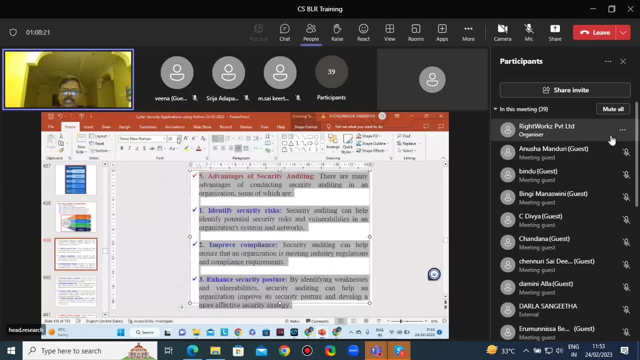 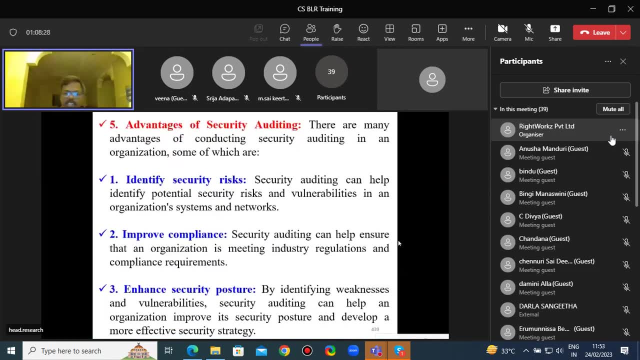 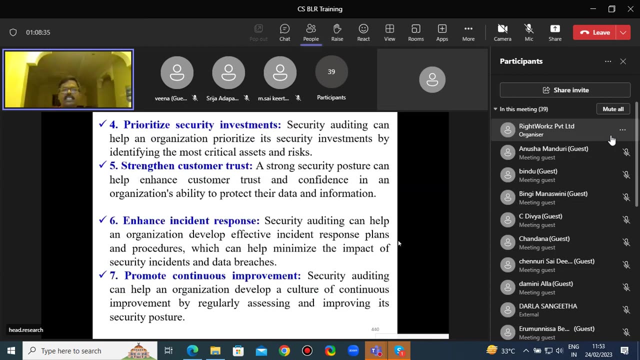 So that is the first advantage of enhancing security portion. okay, So these are the advantages. And fourth advantage is prioritize security investments. See security auditing can help an organization prioritize its security investments by identifying the most critical assets and risks- That is one more advantage. And strengthen customer trust. Strong security portion can help enhance customer trust and confidence in an organization's ability to protect their data and information. That is called strengthen customer trust. Then enhance incident response. 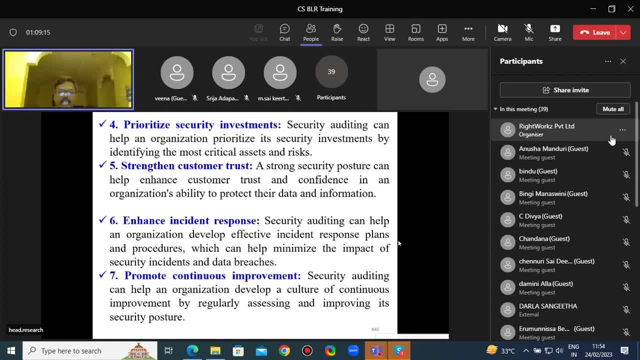 Next advantage: security auditing and organization. Effective incident response plans and procedures which can help minimize the impact of security incidents and data breaches. Promote continuous improvement. Security auditing can help an organization develop a culture of continuous improvement by regularly assessing and improving its security posture. 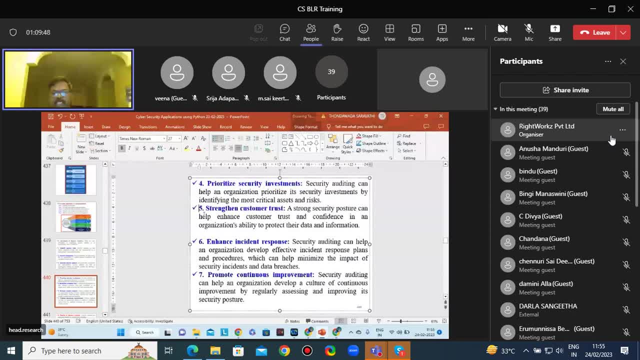 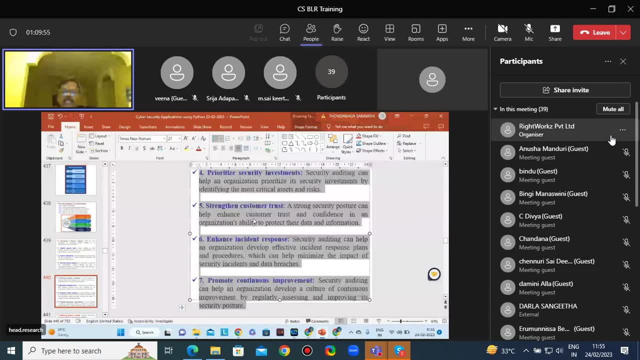 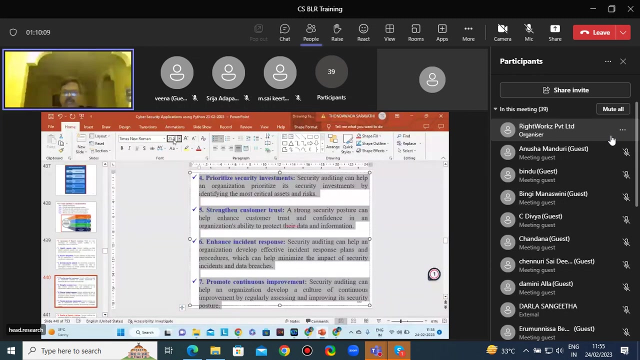 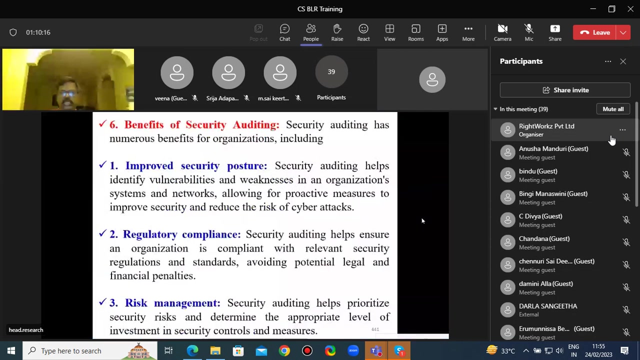 So that is called an advantage of security auditing. You can call it as security auditing advantage. There are seven types of advantages we are studying in this cell. Next one is benefits of security auditing. So security auditing has numerous benefits for organizations, including improved security posture. I have explained. 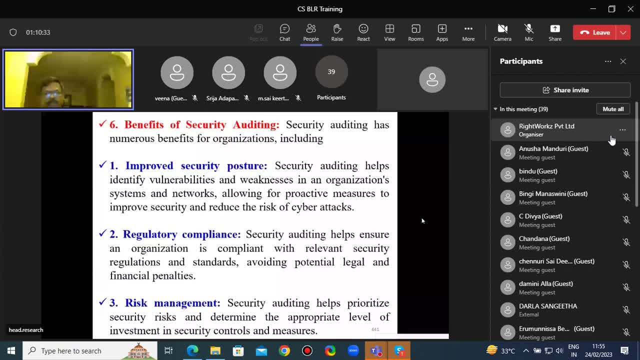 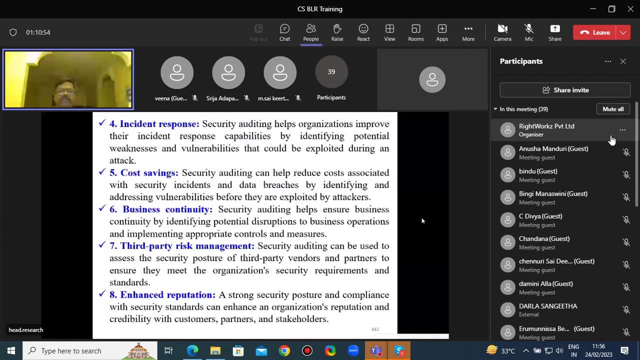 It helps ensure an organization is compliant with relevant security regulations and standards, avoiding potential legal and financial penalties and risk assessment. I know Incident response is nothing but security. auditing helps organizations improve their incident response capabilities by identifying potential weaknesses and vulnerabilities that could be exploited during an attack. 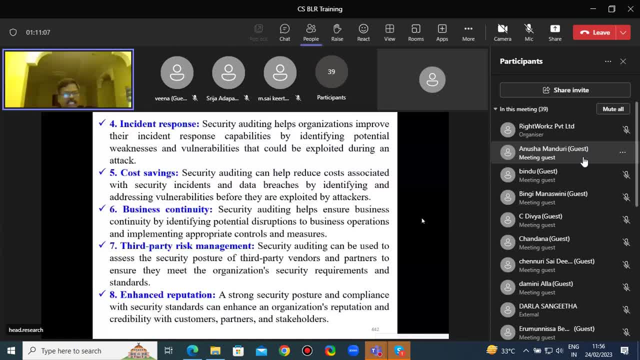 Then the fifth benefit is cost savings. Okay, It gets a little bit dry now. It is a little bit dry now. How do you save the cost of the services? All these are the benefits. cost of the organization. Security auditing can help reduce cost associated with security. 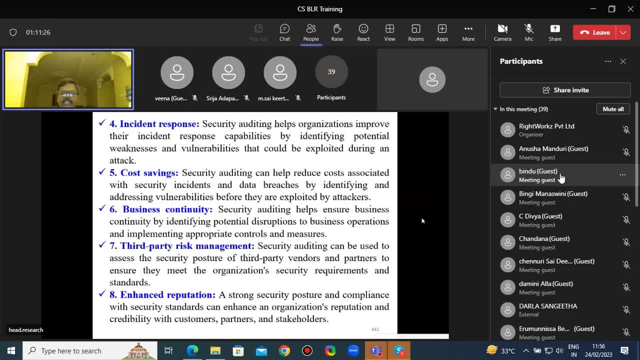 incidents and data breaches by identifying and addressing vulnerabilities before they are exploited by hackers. See if anything happened for organization people. they are getting insurance- Suppose car accident, car bomb, anything happened- So in that case the benefit of cyber security, they are getting reimbursement of the incident. Then business. 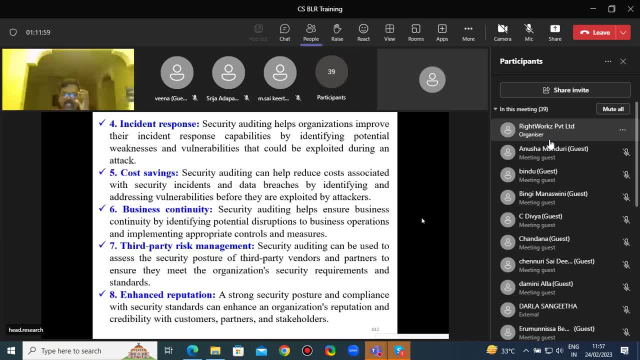 continuity. Ensure business continuity by identifying potential disruptions to business operations And implementing appropriate controls and measures. Third party risk assessment: Security auditing can be used to assess the security portion of third party vendors and partners to ensure they meet the organization security requirements and standards. That is called 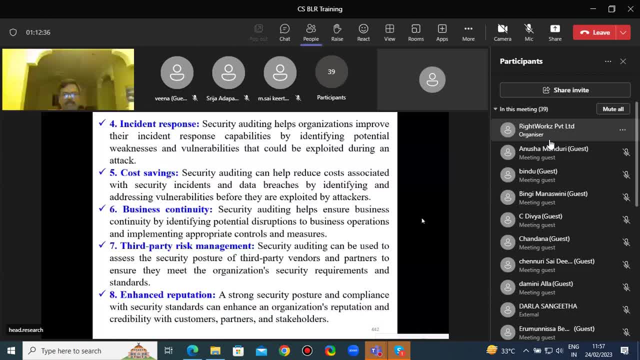 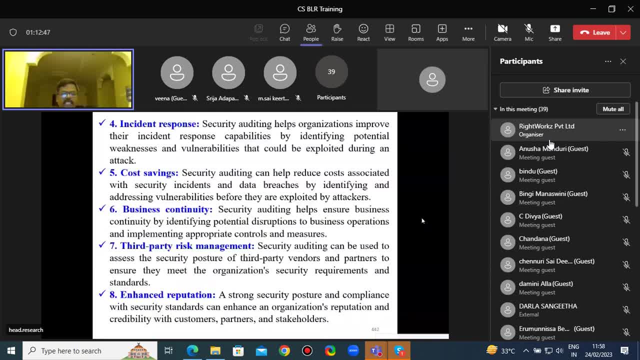 gap moments: Third party risk management. date is 11 July. Science projections for the upcoming deux 2016. and in the coming 30 days, development of the school cycle will be Initiative log基. Masterwho ofください's hypnosis舊. 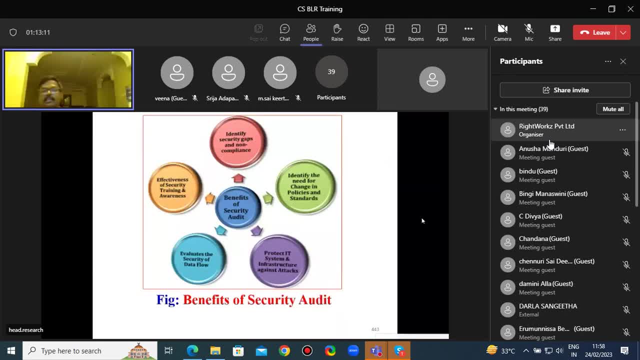 and non-compliance. That is one more benefit of security audit. Security: identify the need for change in policies and standards. Then protect information technology system and infrastructure against attacks. Evaluate the security of data flow, Effectiveness of security, training and awareness. These are the benefits of security audit. Then security: 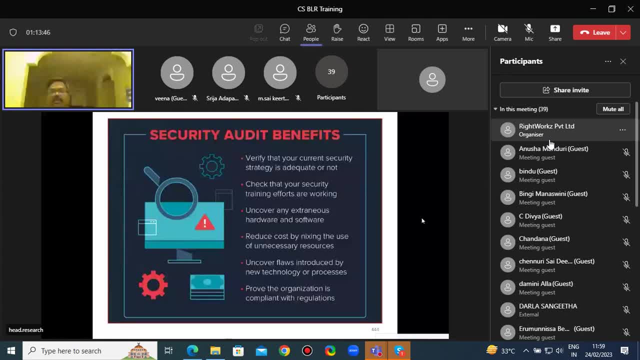 audit benefits are: verify that your current security strategy is adequate or not. Check that your security training efforts are working or not. Uncover any extraneous hardware and software. Reduce cost by X, Fixing the use of unnecessary resources. Uncover flaws introduced by new technology. 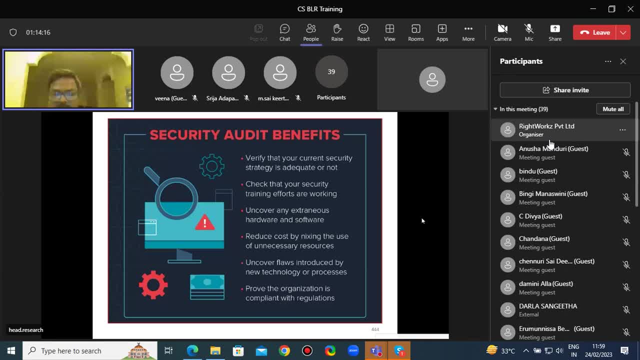 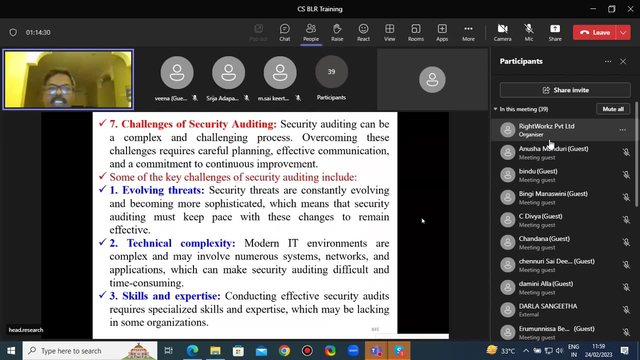 or processes through the organization is compliant with regulations. These are called security audit benefits. Then, seventh one, challenges of security auditing. Security auditing can be a complex and challenging process. Overcoming the challenges of security auditing can be a complex and challenging process. Overcoming the challenges of security auditing can be. 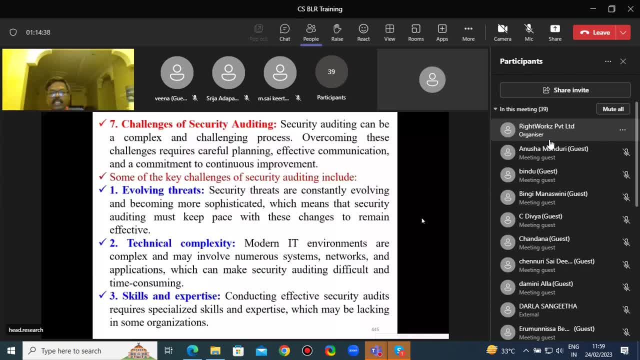 One of these challenges requires careful planning, Effective communication, community feedback and a commitment to continuous improvement. Dutch Kalufan. Some of the key challenges of security auditing includes evolving threats. This is a major challenge of security audit. Security threats are constantly evolving and becoming more. 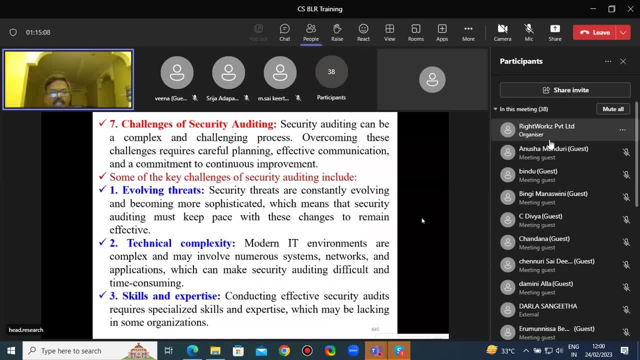 sophisticated, which means that security auditing must keep face with these changes to remain effective. technical complexity is a challenge of security auditing in this modern information technology environments are complex and may involve numerous systems, networks and data centers and applications, which can make security auditing difficult and time consuming. then, third, 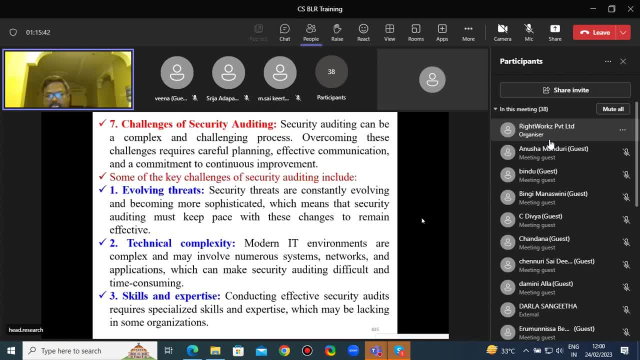 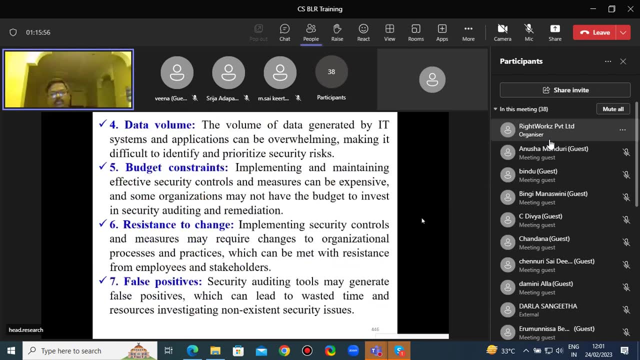 one is skill center enterprise. conducting effective security audits requires specialized skills and expertise which may be lacking in some organizations. then the data volume. data volume is a challenge of security. the volume of data generated by information technology systems and applications can be overwhelming, making it difficult to identify and prioritize security risks. 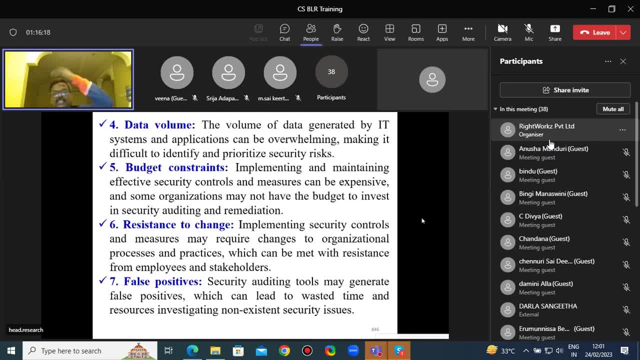 so that is one more challenge: budget constraints. implementing and maintaining effective security controls and measures can be expensive and some organizations may not have the budget to invest in security auditing under remediation. that is one more challenge of security audit: budget constraints. resistance to change: it is a one more challenge. 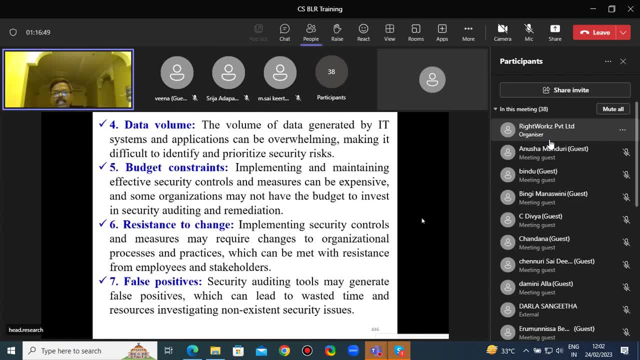 of security auditing. that implies implementing security controls and measures, many required changes, with resistance from employees and stakeholders. then the seventh research challenge is false positives. security auditing tools may generate false positives, which can lead to wasted time resources investigating non-existent security issues. so false positive also one of the security. 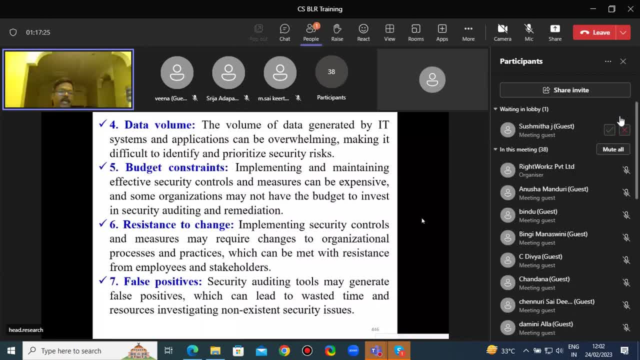 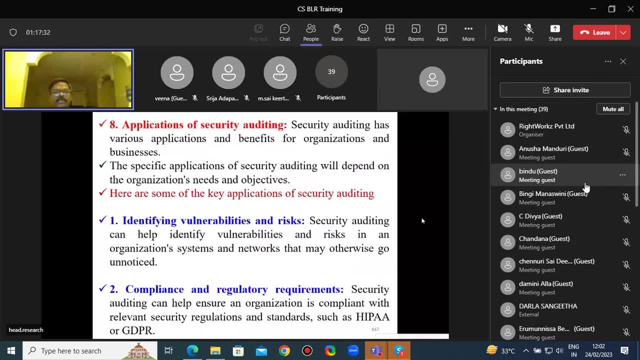 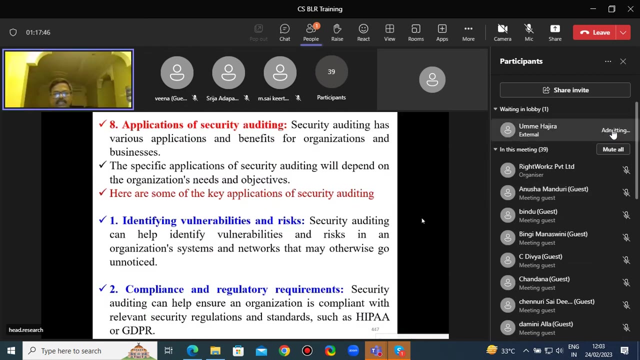 challenges. this is a very important factor in order to ensure that we provide a secure of security auditing. Then the eighth one: applications of security auditing. So security auditing has various applications and benefits for organizations and businesses. The specific applications of security auditing will depend on the organization's needs and objectives. 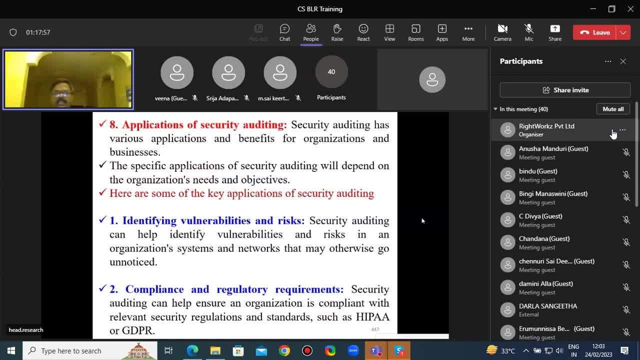 Here are some of the key applications of security auditing. First one is identifying vulnerabilities and risks. So security auditing can help identifying vulnerabilities, attacks, criminal activities, breaches and risks in an organization's systems and networks that may otherwise go unnoticed. That is called identifying vulnerabilities and risks, Compliance and regulatory requirements. 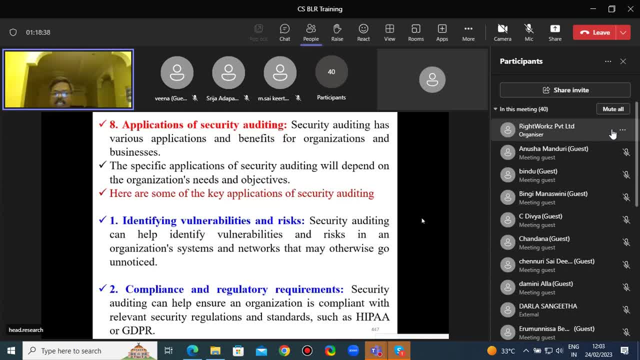 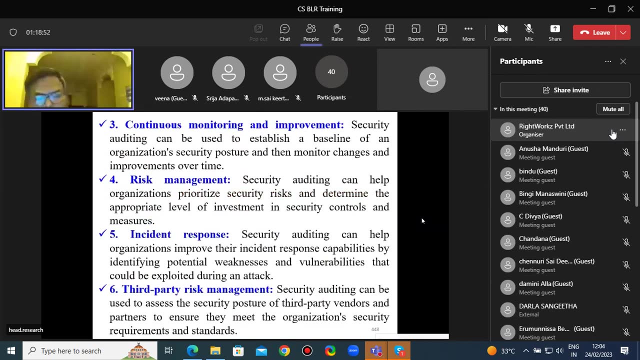 Security auditing can help ensure an organization is compliant with relevant security regulations and standards, such as HIPAA or GDPR. So these are the applications of cybersecurity auditing. Thank you. Continuous monitoring and improvement: Security auditing can be used to establish a baseline of an organization's security portion and then monitor changes and improvements over. 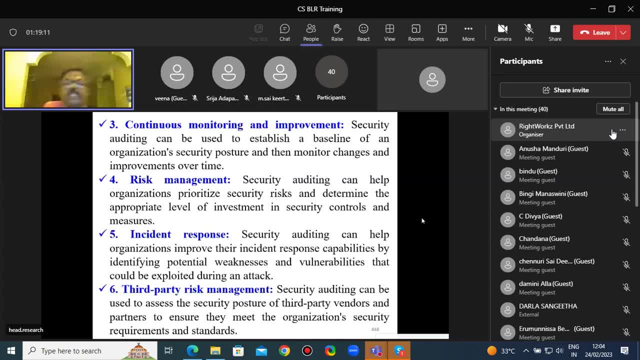 time Risk management. Risk security auditing can help organizations prioritize security risks and determine the appropriate level of investment in security controls and networks That is under risk management. Incident response is one of the applications of security auditing. Security auditing can help organizations improve their incident response capabilities by identifying 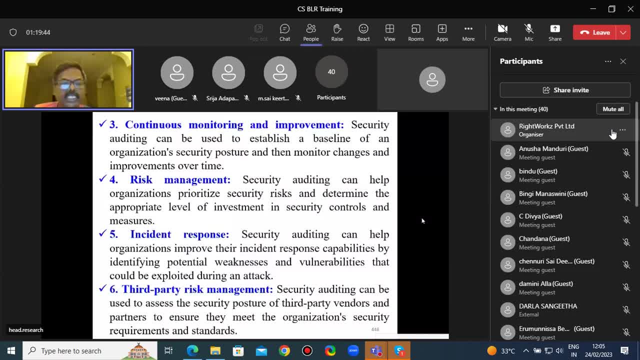 potential weaknesses and vulnerabilities that could be exploited during an attack. The sixth one is third party risk management. Security auditing can help organizations identify potential biases and vulnerabilities that could be exploited during an attack. The sixth management Security auditing can be used to assess the security portion of third party 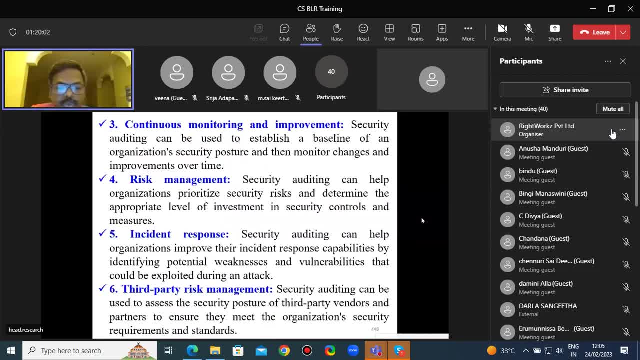 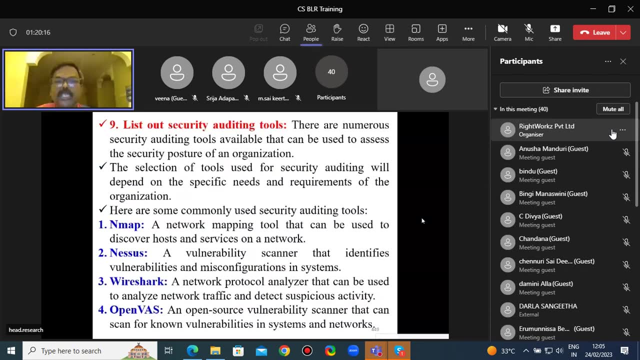 vendors and partners to ensure they meet the organization's security requirements and standards. That is called third party management. So last but one, list out security auditing tools, How many tools we are using for security auditing. There are numerous security auditing tools available that can be used to assess the security portion of an organization. The 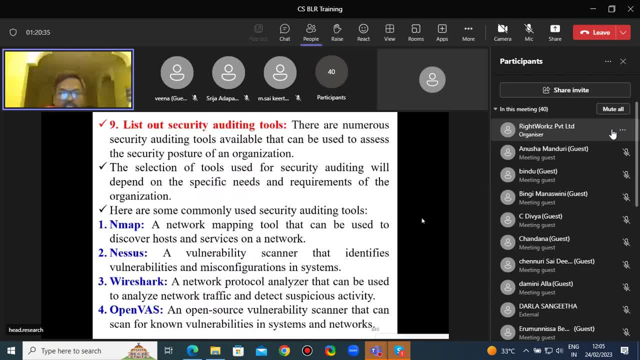 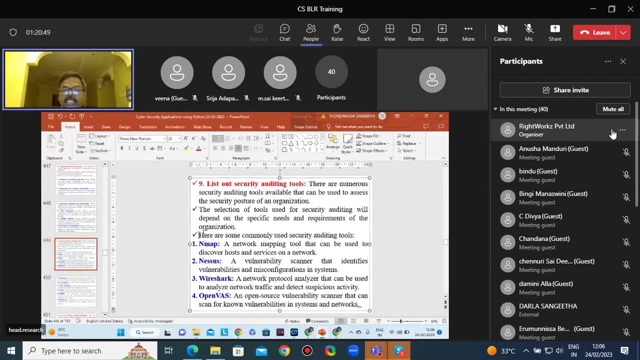 selection of tools used for security auditing will depend on the specific needs and requirements of the organization. Here are some commonly used security auditing tools. I think you, everybody, knows these security auditing tools. Those are Nmap. So what is meant by Nmap? Nmap- 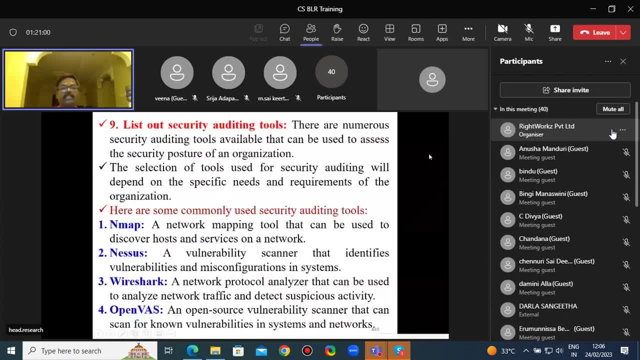 is a security auditing tool, a network mapping tool that can be used to discover hosts and services on a network. Nessus is a security auditing tool, a vulnerability scanner that identifies vulnerabilities and services on a network. Nessus is a security auditing tool that detects the misconfigurations in a system. Then Wireshark: Wireshark is a security auditing. 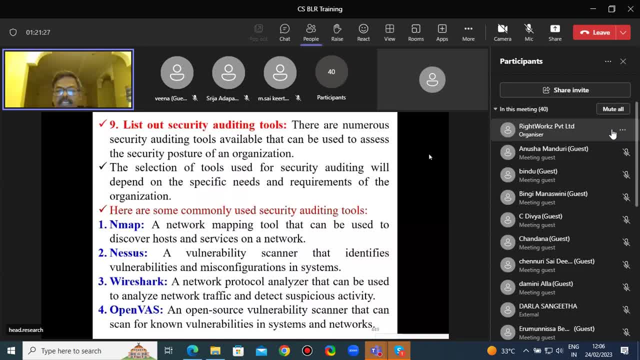 tool, a network protocol analyzer that can be used to analyze network traffic and detect suspicious activity. Then OpenVAS. So OpenVAS is a security auditing tool, an open source vulnerability scanner that can scan for no vulnerability. So OpenVAS is a security auditing. 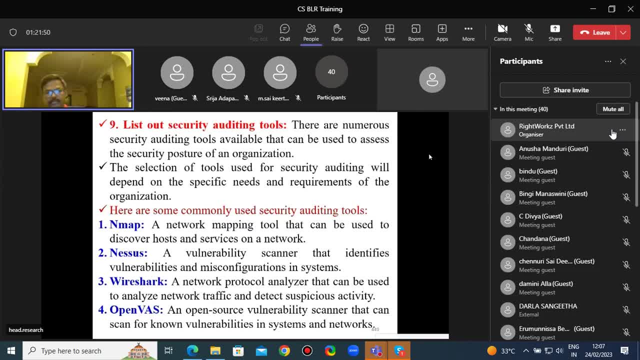 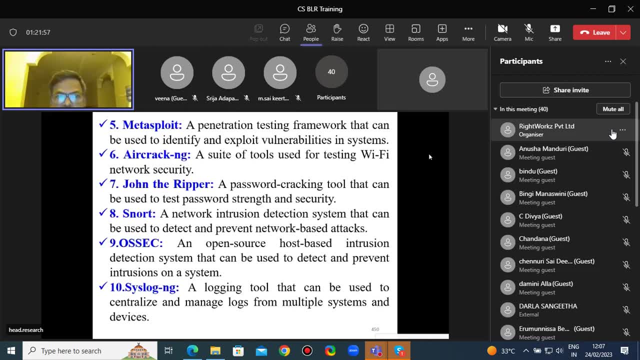 tool, a network mapping tool that can track vulnerability in systems and networks. Then see. the fifth security auditing tool is Metasploit, A penetration testing framework that can be used to identify and exploit vulnerabilities in systems. Sixth tool is 8 Crack Engine. It is a security auditing tool, a suite of tools used for testing. 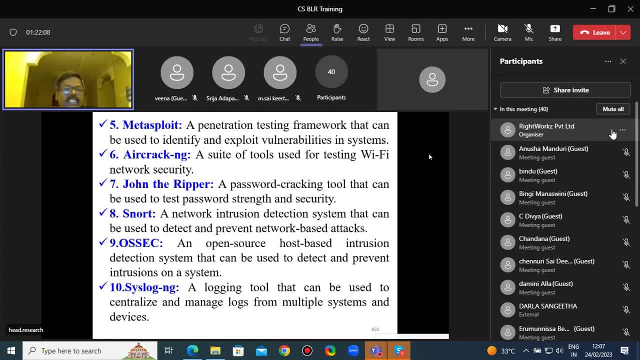 Wi-Fi and quasi-systems, You can define, identify and exploit vulnerabilities in systems. Sixth tool is 8 Crack Engine, which is a security auditing tool, a suite of tools used for testing Wi-Fi and quasi-systems network security, Wireless fidelity. network security auditing tool. John the Ripper: it is a security auditing tool, a password cracking tool that can be used to test password strength and security. 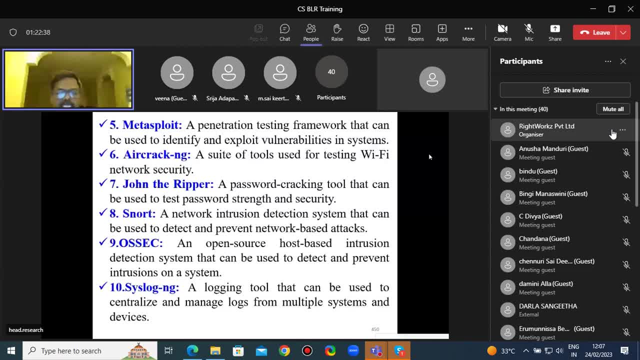 Snort. Snort is a security auditing tool, a network inclusion detection system that can be used to detect and prevent network based attacks. OSEC, an open source host based inclusion detection system that can be used to detect and prevent inclusion services. Syslog and NG, a logging tool that can be used to 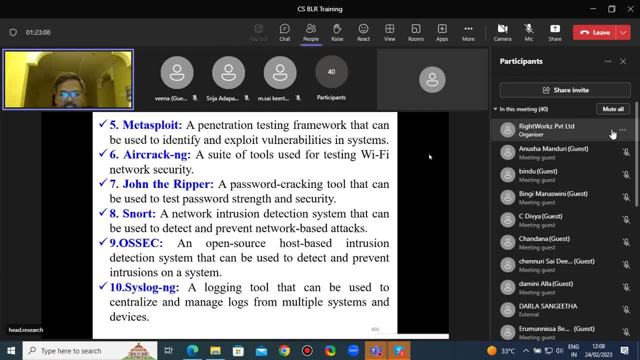 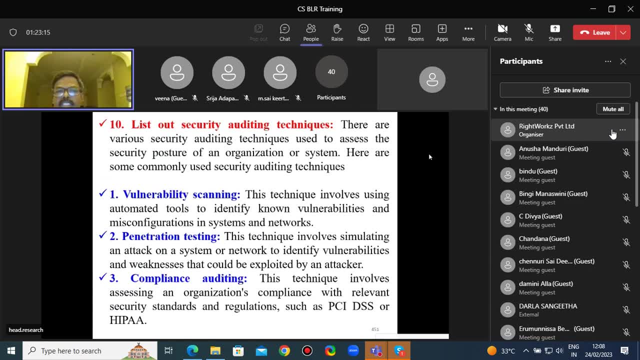 centralize and manage logs from multiple systems and devices. Then the last topic in security auditing: list out security auditing techniques. There are various security auditing techniques used to assess the security portion of an organization or system. Here are some commonly used security auditing techniques like vulnerability scanning. 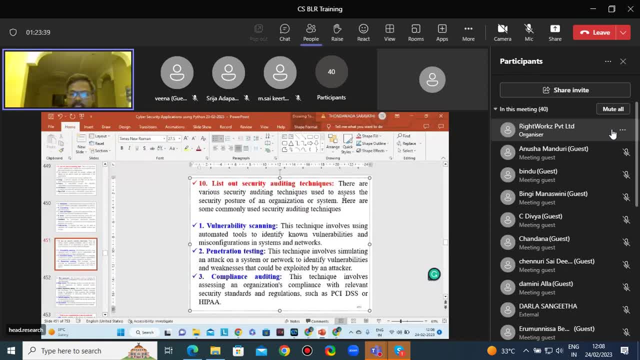 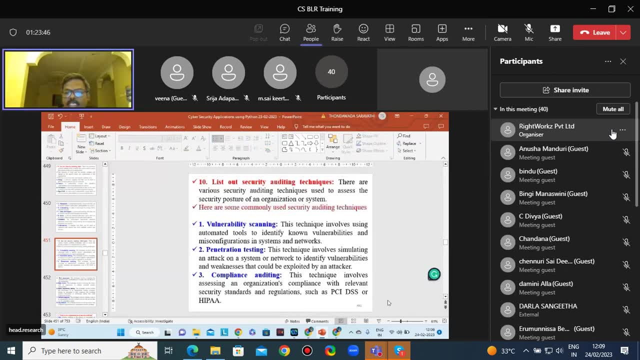 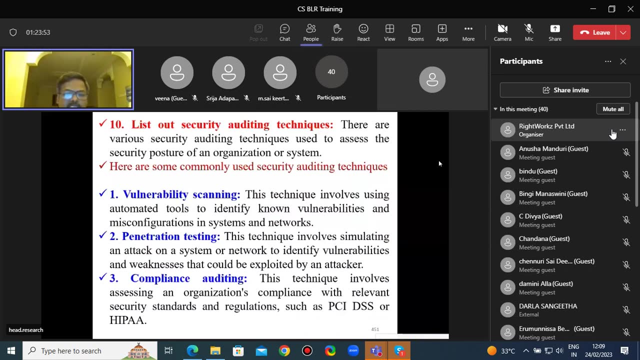 Vulnerability scanning is a security auditing technique. It is a security auditing technique: Vulnerability scanning, Then penetration testing. So vulnerability testing is nothing but this. technique involves using automated tools to identify known vulnerabilities and misconfigurations in systems and networks. Penetration testing is nothing but this. 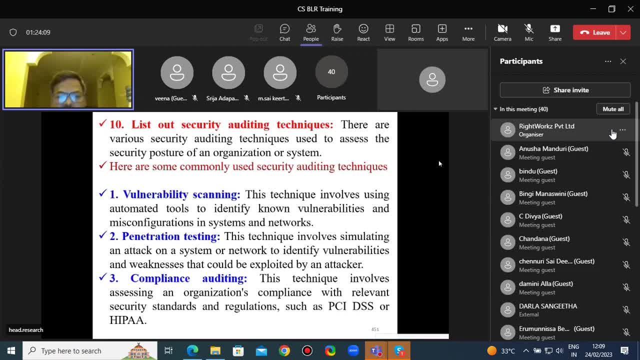 This technique involves simulating an attack on a system or network to identify vulnerabilities and weaknesses that could be exploited by an attacker. Compliance auditing: It is one of the security auditing techniques. This technique involves assessing an organization's compliance with relevant security standards and regulations, such as PCI, TSS and HIPAA. 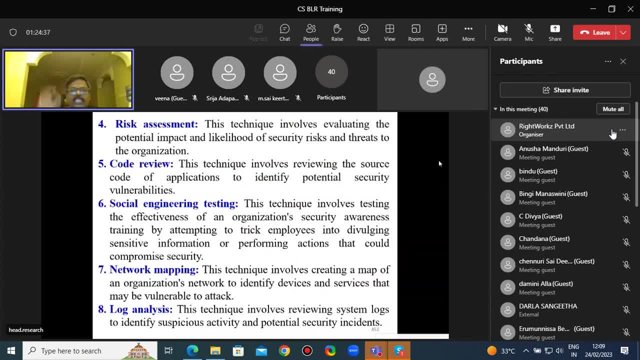 Then, risk assessment: This technique involves evaluating the potential impact and likelihood of security risks and threats to the organization. Code review: This technique involves reviewing the source code of applications to identify potential security vulnerabilities. Social engineering test: This technique involves test the effectiveness of an organization's security awareness. 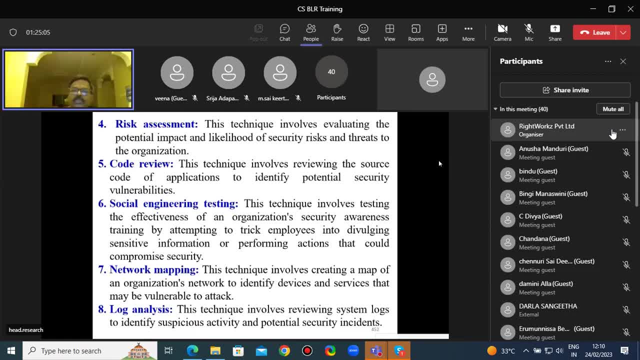 training by attempting to trick employees into rivalizing sensitive information or performing actions that could compromise security. Network mapping: This technique involves creating a map of an organization's network to identify devices and services that may be vulnerable to attack. Log analysis: This technique involves reviewing system logs to identify suspicious activity or potential security incidents. 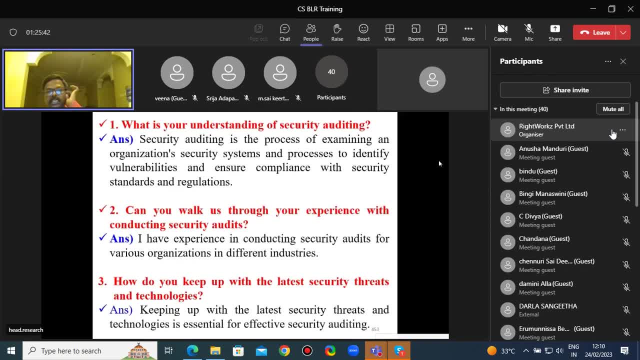 So with this, one theory part is completed. Now the interview questions. What is your understanding of security auditing? Security auditing is the process of examining an organization's security systems processes to identify vulnerabilities and ensure compliance with the security standards and regulations. Can you walk us through your experience with conducting security audits? 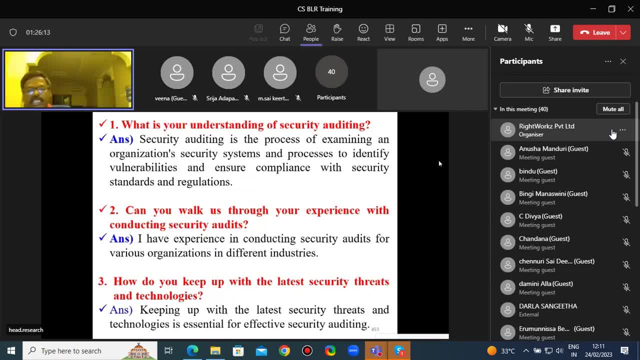 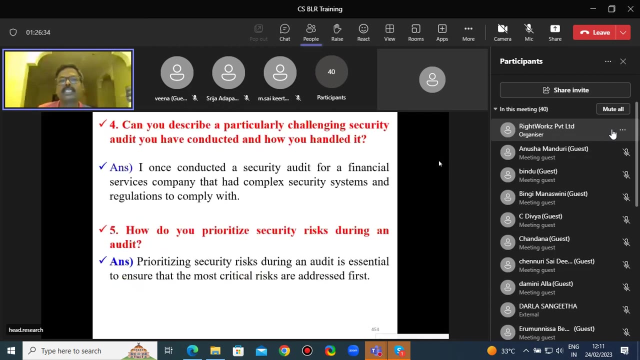 Yes, sir, I have experience in conducting security audits for various organizations in different industries. How do you keep up with the latest security threats and technologies? Keeping up with the latest security threats and technologies is essential for effective security audit. Then can you describe a particularly challenging security audit you have conducted and how you have handled it? 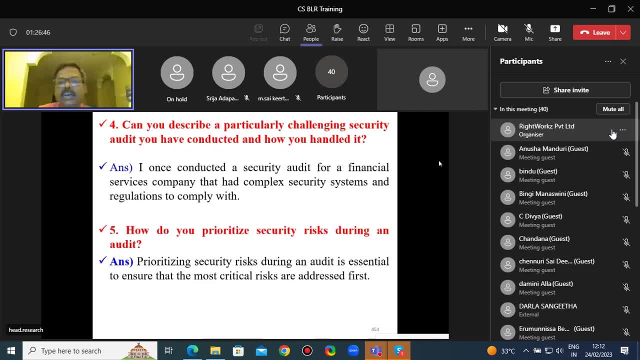 Yes, I have experience. conducted a security audit for a financial services company that had complex security systems And regulations to comply. How do you prioritize security risks during an audit? Prioritizing security risks during an audit is essential to ensure that the most critical risks are addressed first. 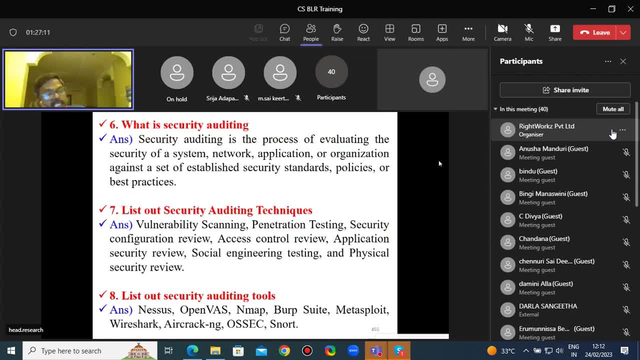 Then what is security auditing? Security auditing is a process of evaluating security of a system, network applications, data center. Our organization again has a set of established security standards, policies, rules and regulations or best practices. List out security auditing techniques. 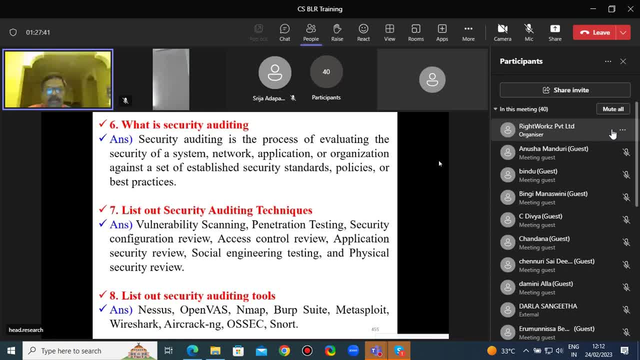 Vulnerability scanning technique. Vulnerability scanning is a security auditing technique, Monitoring testing, Security configuration review, Access control review, Complication security review, Social engineering testing And physical security review. List out security auditing methods: Nessus, OpenVAS. 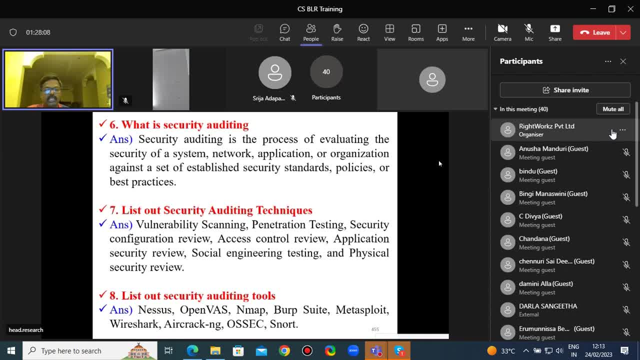 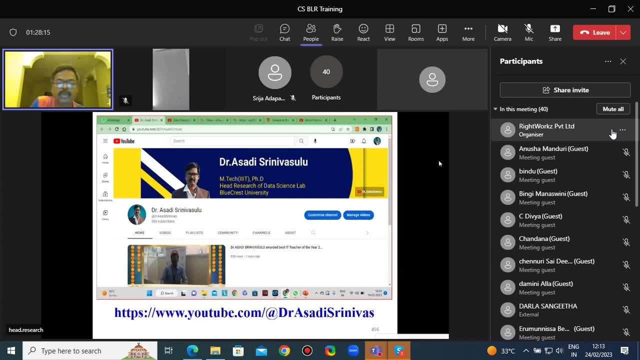 Nmap, Herb Suite, Metasploit, Wireshark, Aircrack, Osec, When security auditing Yesterday, Ethil sir might even homework or assessment already in the afternoon meeting, afternoon training. So now I have updated the information security auditing. 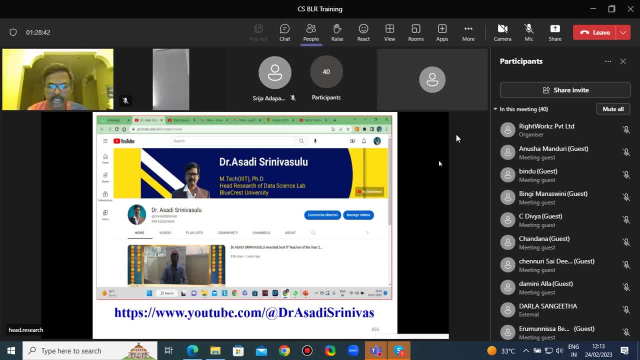 This information I will share with you. So, my dear students, I'm going to stop here stock. here we will see project implementations of individual projects. i have given, i think, three batches code how to execute. you need to take a excel sheet of your input data. 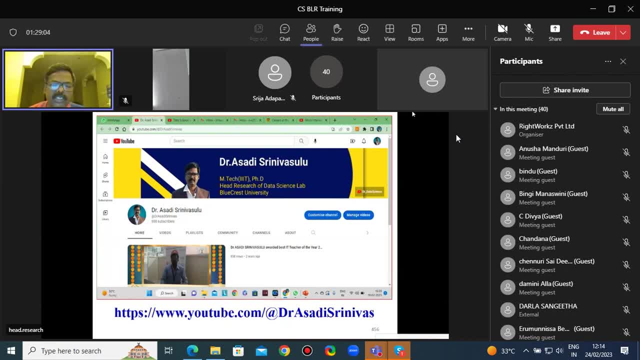 or csv file format. once you have excel sheet we can convert into comma separated variable dot csv file. okay, if you see veca input file, yeah, attribute relation file format. like any type of file, it has to take input and process our execution. my dear students, if any student has not done, 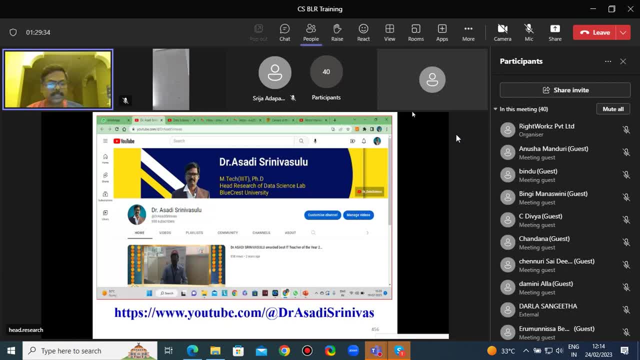 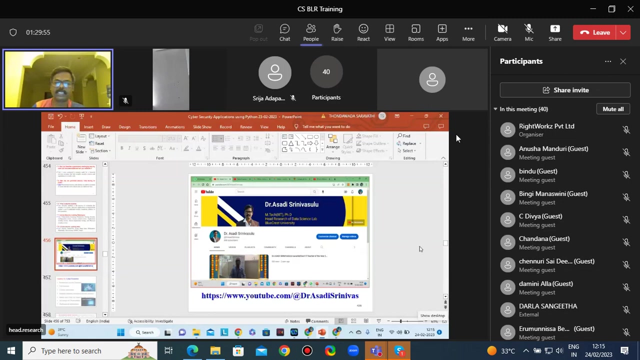 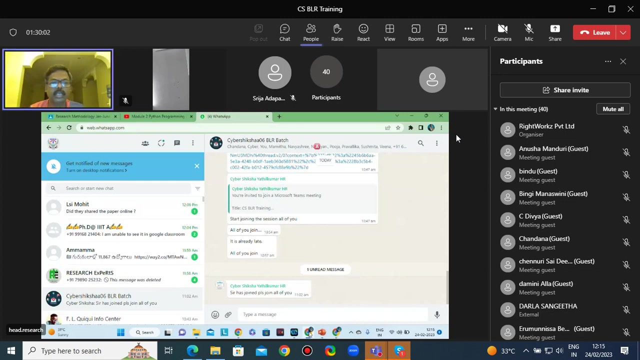 this subscription. please do subscribe my channel. i'm uploading each and every video of cyber security in my channel, so with this one i'm closing the theory session. now i am going to explain and demonstrate project implementation. so how many batches got code and right? hello, my dear students. 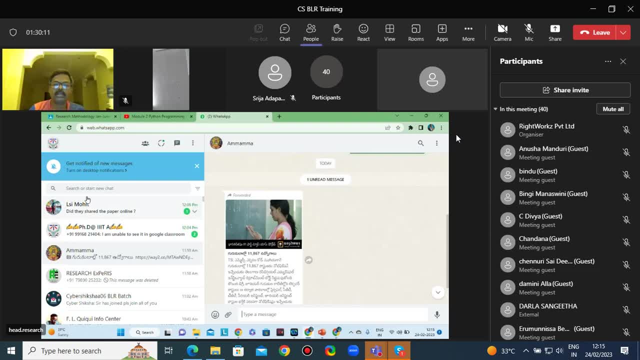 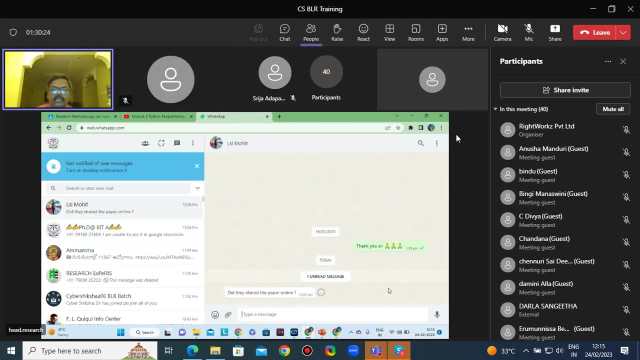 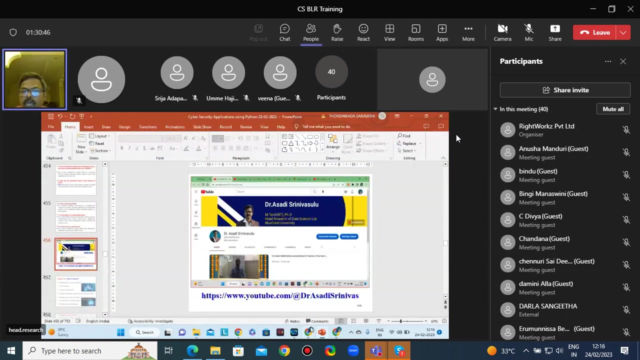 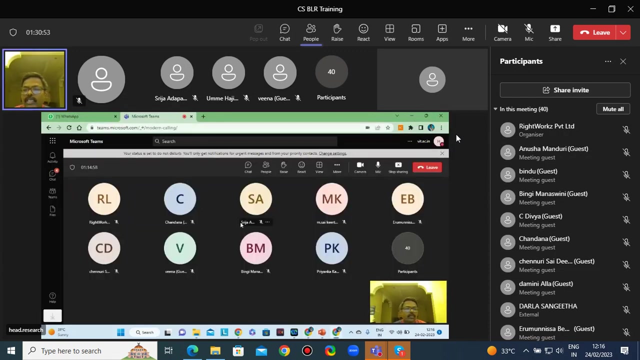 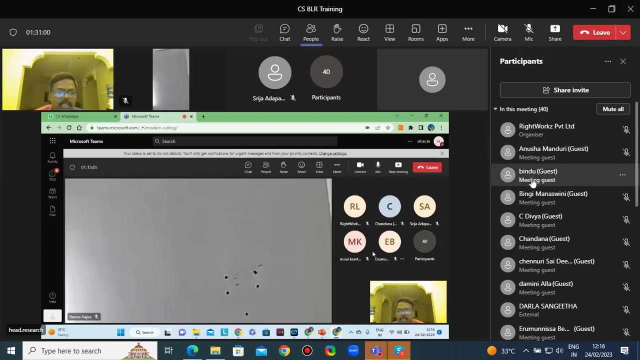 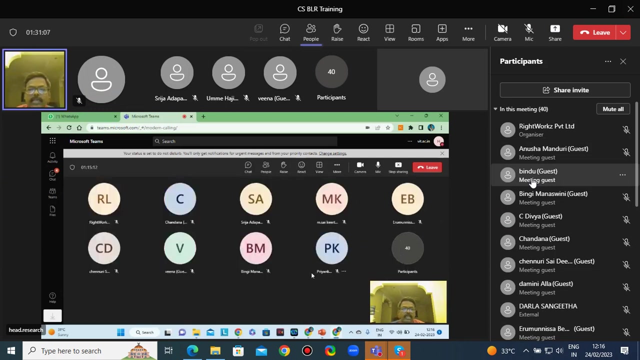 our how many batches you got it? yes, um, um, any idea of many patches you got it? Hello, 5 students are not responding. 40 students are there. my voice is audible. yes, sir, ok, ok, that's good. and anyone implemented project: see, there is a procedure for implementation of your project. 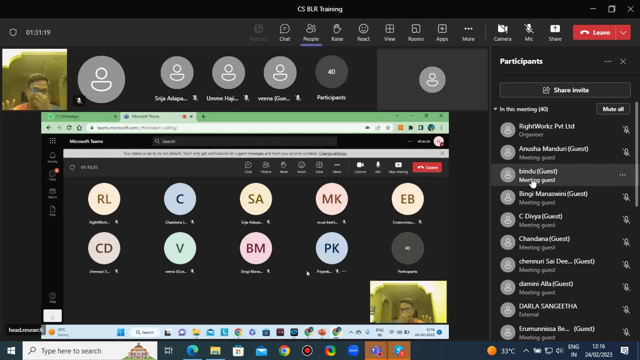 first you need to collect the data set. data set may be excel sheet or csv file format. data set: yeah, so I think 1 hour 2 batches sent data sets. I am evaluating, I am checking and I have given 1 data set. 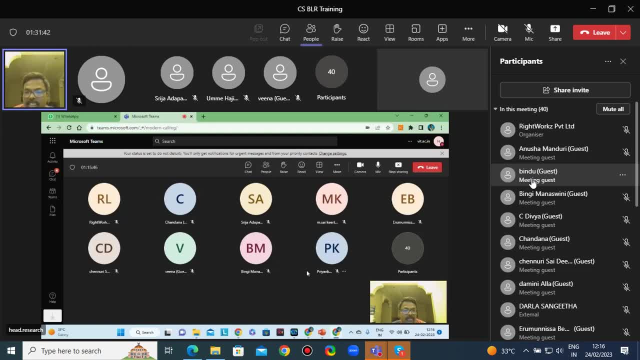 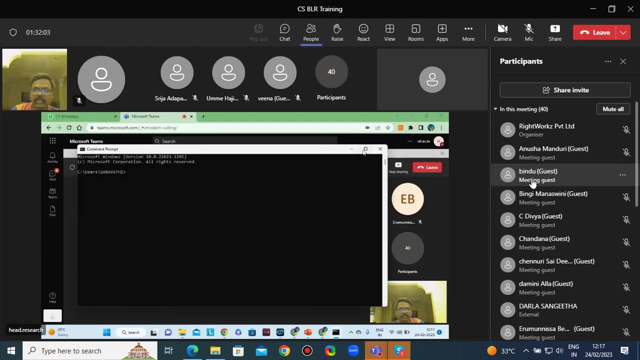 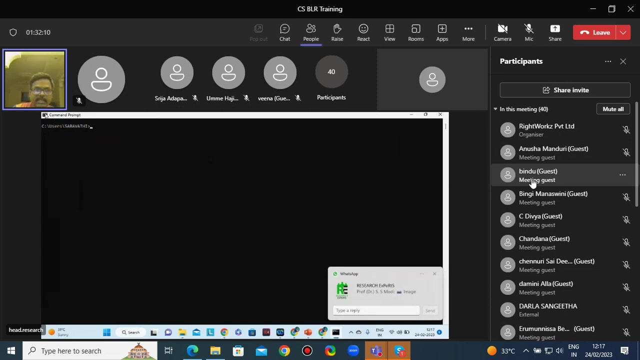 that is called power quality data set. so in that power quality data set I have included number of instance or threads and malware. then it is going to verify our data. see now I am going to execute that one. how to execute how to execute that main project. likewise, see, my screen is visible. hello, please. yes, sir. 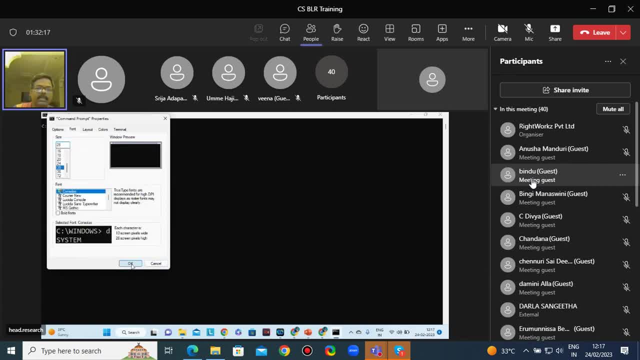 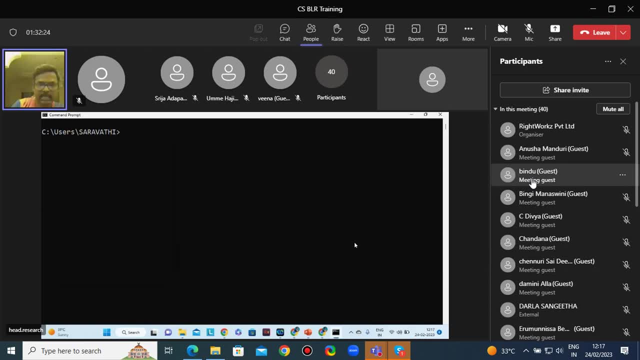 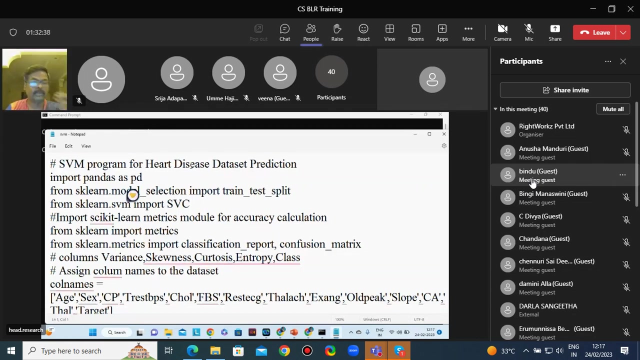 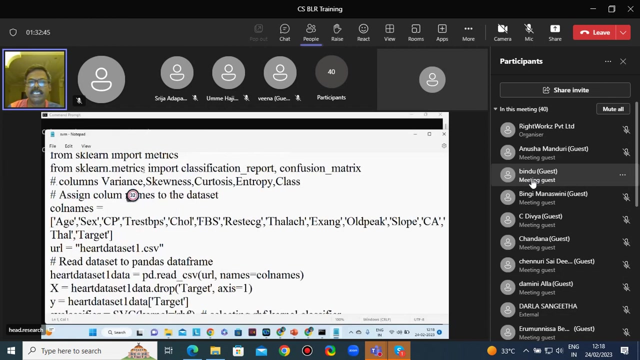 my screen is visible. ok, now, see. so I have implemented support vector machine once again. I am opening first that file, notepad space, svmpy. this code: ok, at least you can try this, this one I have developed and I have sent to for ok in the online. I have sent. see, this is the code I have tested for csv data. csv means comma separated variable for heart disease. 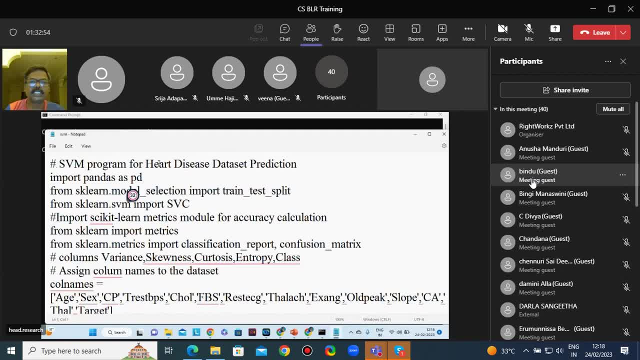 prediction. you can remove this heart disease data set prediction. you can include malware detection or packet sniffing data set or cyber security data set or cyber forensics data set or any kind of mobile security data set or web security data set. you can download from the internet excel file or csv file. if you get excel file, we can. 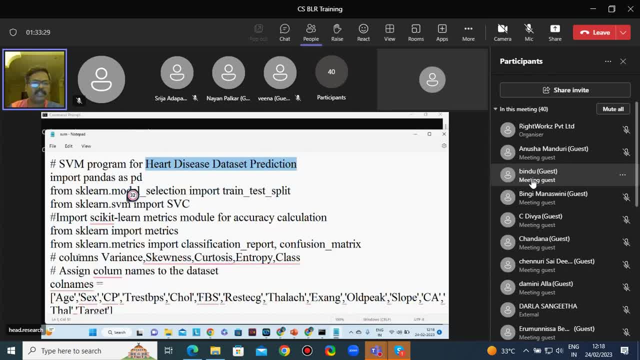 we can convert it to csv file. you need to check the columns. only you need to change the aim of the program like a write a python program to perform packet sniffing detection using support vector machine. you need to change like that. then this code, as it is, you can use here. you need to change column variance like variance, skewness, kurtosis, entropy and class. 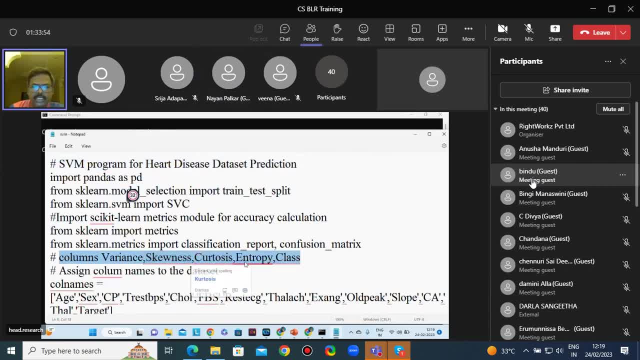 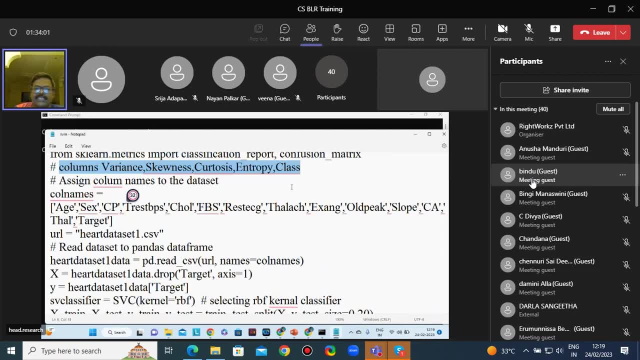 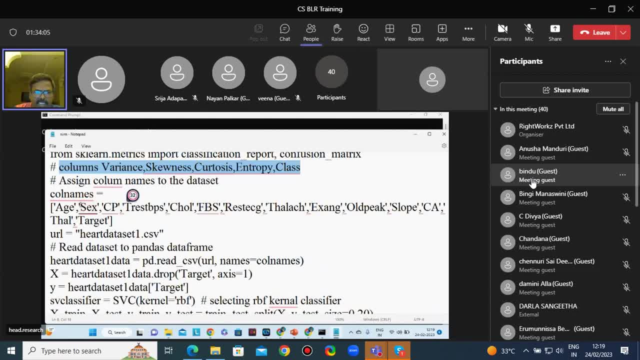 thing then column names in the data set, like this age you can change here. so there you need to use your data set columns. how many columns are there? so you need to change age, gender, cholesterol, like for related to heart disease, then this is the data set you need to give here. 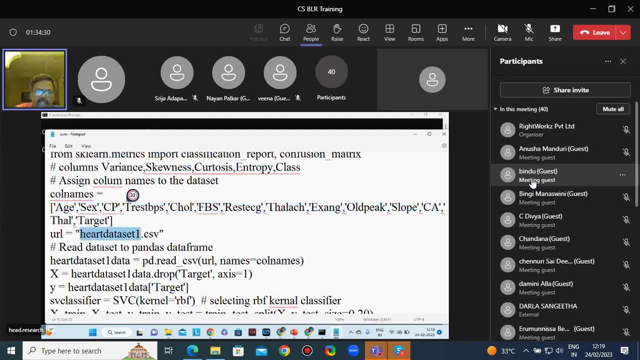 malware detection data set- dot csv. or malware cyber forensics data set- dot csv. here you need to change. that's all the data set name you need to give and the column names you need to change. that's all your program will execute now see, and what is the data set i have taken. 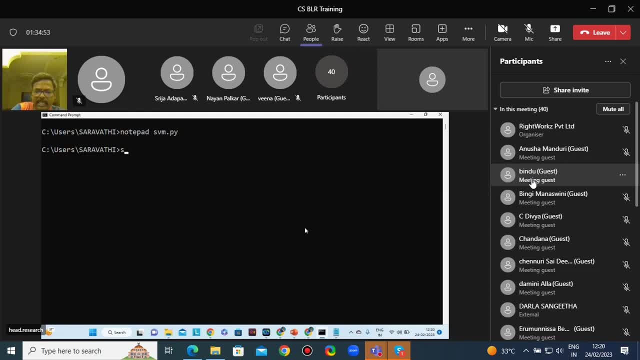 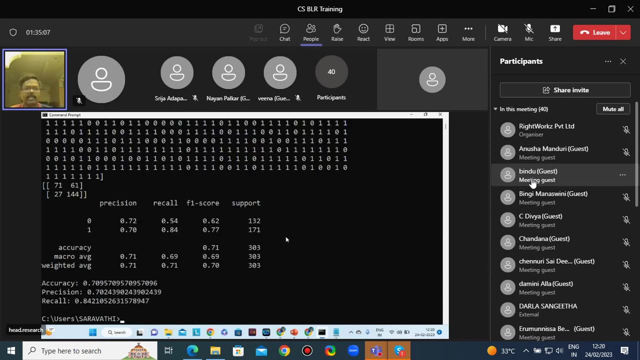 so i am opening first, i am executing, then i will see what type of data set i have. uh, i have used for my my implementation, see now. now python is executing 303 records. i have taken and i got 17.95 percentage accuracy. now what is the data set can you see in this one? 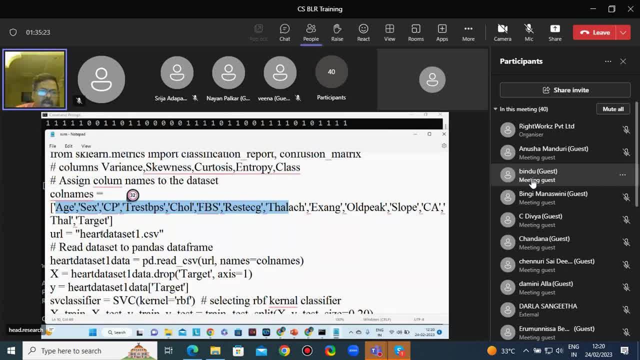 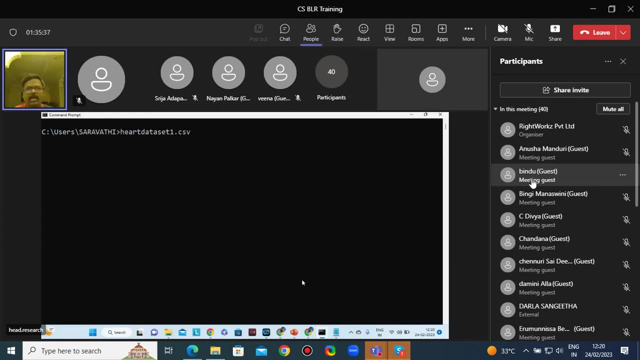 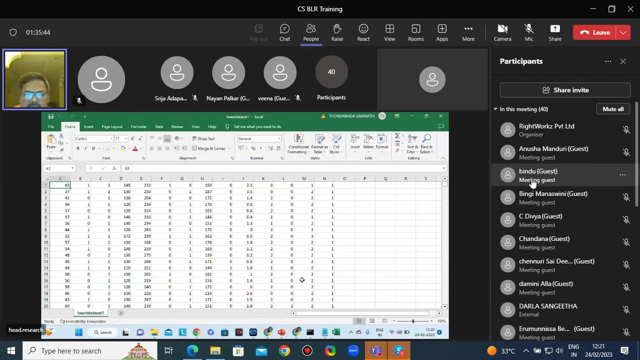 hot data. just i'm giving example: hot data set one. so this is the data set. i will change here. malware detection data set. so now, see here. i would like to open for the data set one dot csv. you can open. see, now my system is opened. excel sheet. my screen is visible. 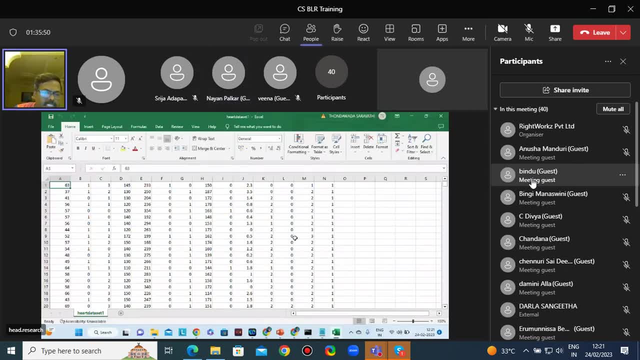 please. so this is first. column means age of the person. age. then cholesterol is there or not, bp is there or not? any kind of testing? finally, target class one means whether that patient having a heart disease or not. so zero means there is no heart disease. one means: 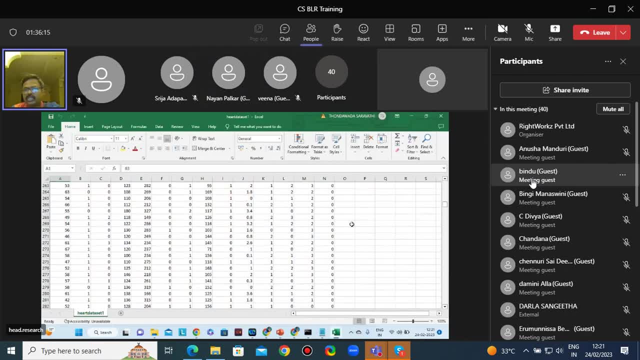 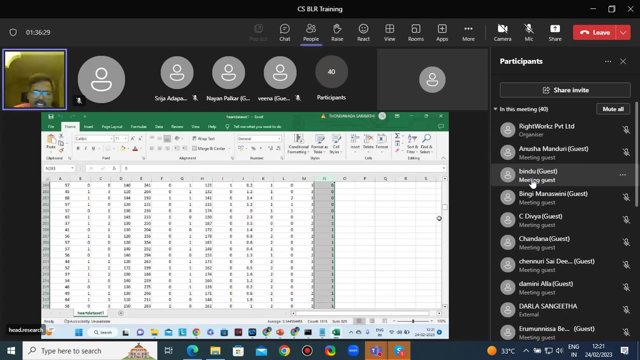 there is a disease like that. see zeros are also presented. last column is target class. means classification is a supervised learning. it uses target class. we are. we are calculating whether that person having disease or not. or we are calculating malware detection: whether the malware detection, how many threats it is identified through, how many threats are happened. 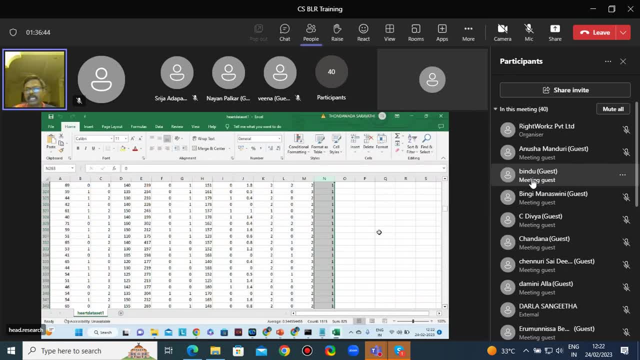 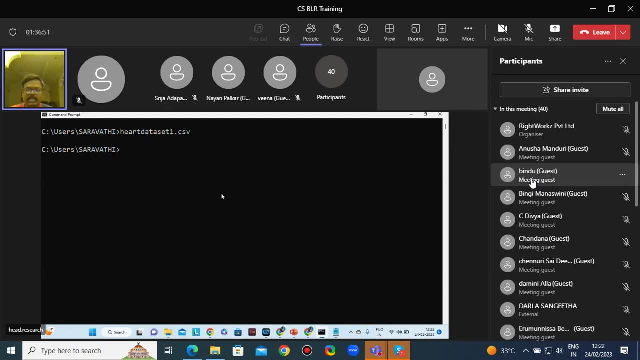 no threats are. that is called a zero, like that. this is the data set, this is csv5 and like this you can execute your project. and who are expecting code from my site i am going to share with you right now? tell me yeah, tell me so for geolocation extraction. okay, now i am giving geolocation. 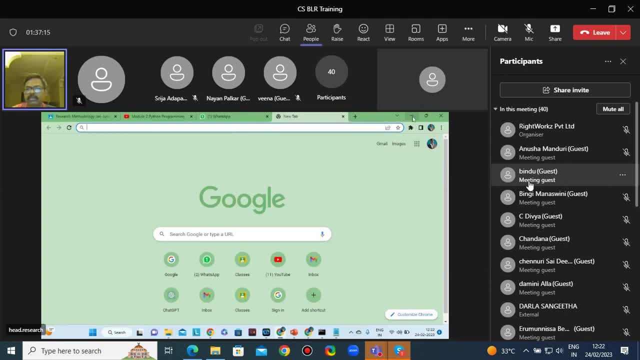 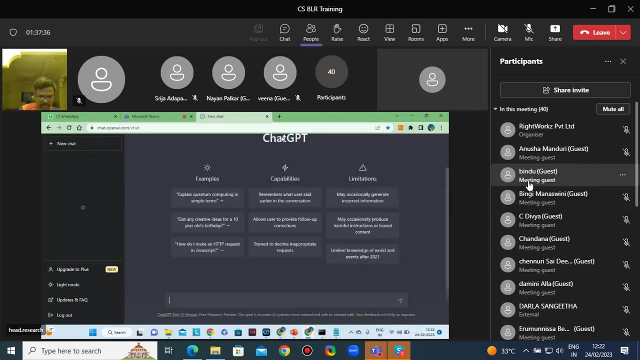 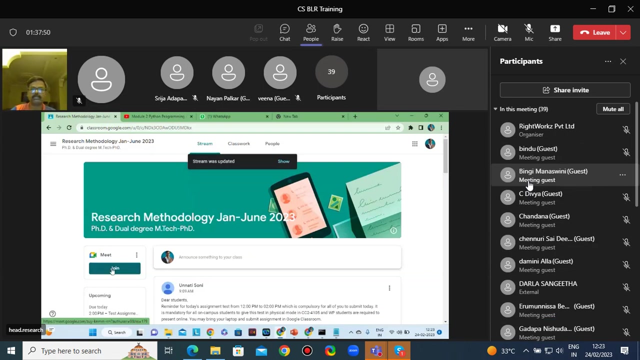 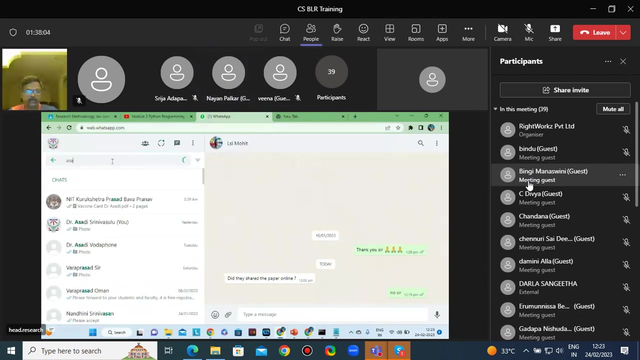 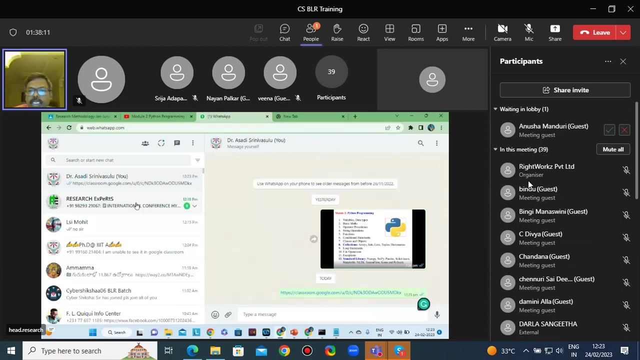 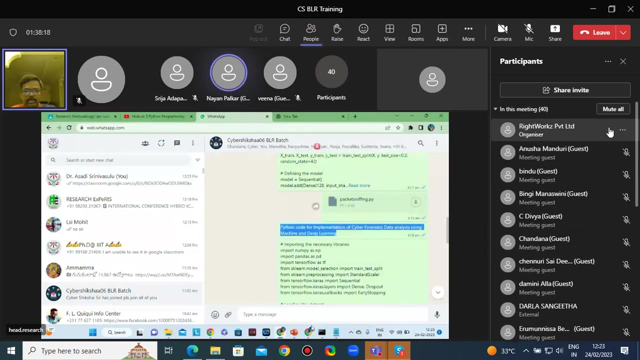 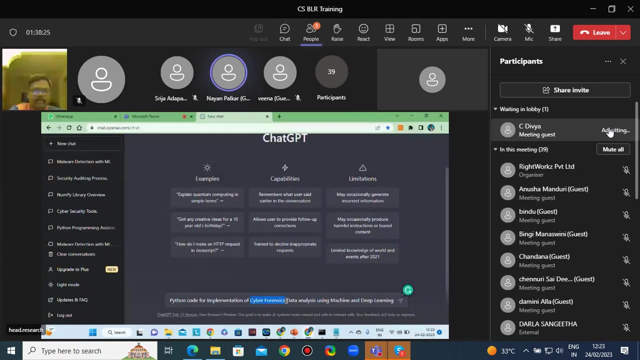 one second geolocation. so i am giving geolocation data set. please check i am sharing, so you need to do. yesterday i have- i have given So very several bats yesterday night- have seen like this: you can search: what is that bat, what is your problem mouse, what is your problem cell. ok, that's it for geolocation. 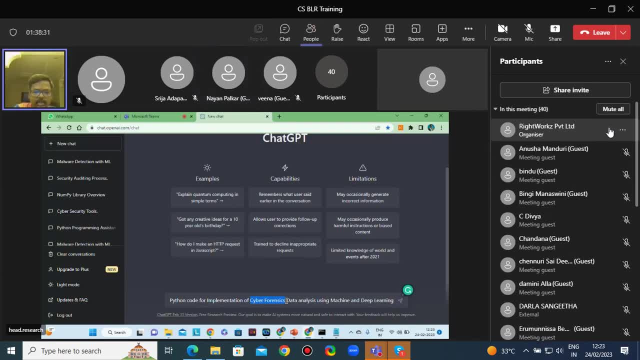 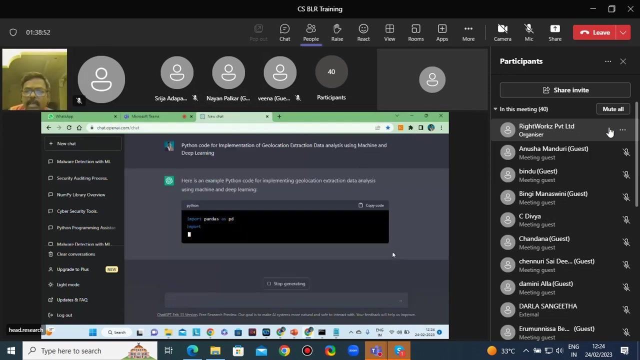 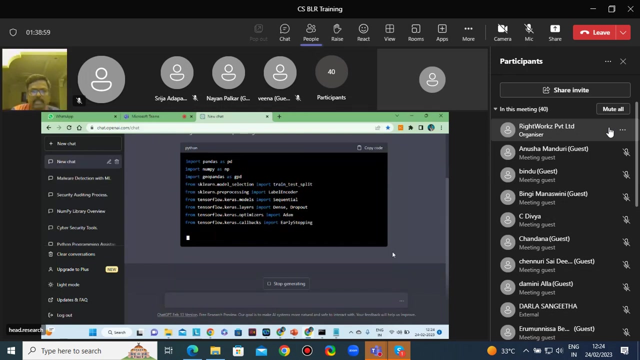 extraction: ok, geolocation, geolocation, that's all. extraction: ok, geolocation extraction: data analysis using machine and deep learning code. now, see so my chart GPT is generating a code for implementation of geolocation extraction. ok, so data set. 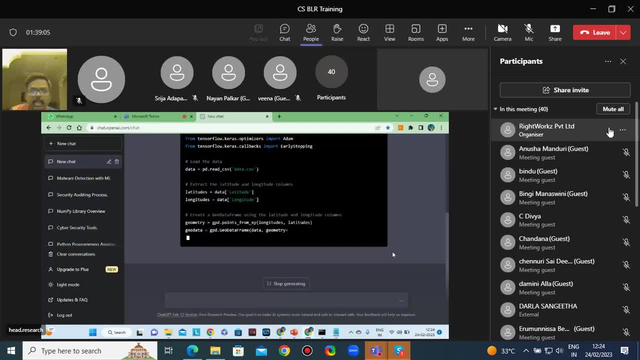 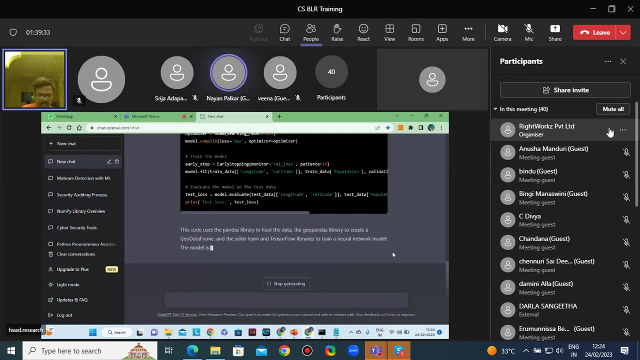 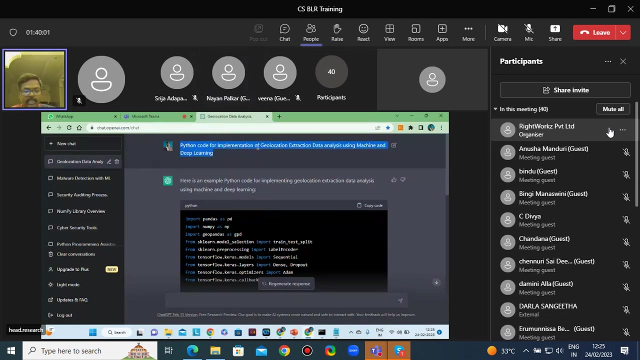 you are taking data: dot CSV, comma separated variable. ok, now see the. and. please open all of you. try to execute now, please. please open your system. Please open all of you. Yeah, now I am sharing the code. please see the geolocation extraction. please go to your. 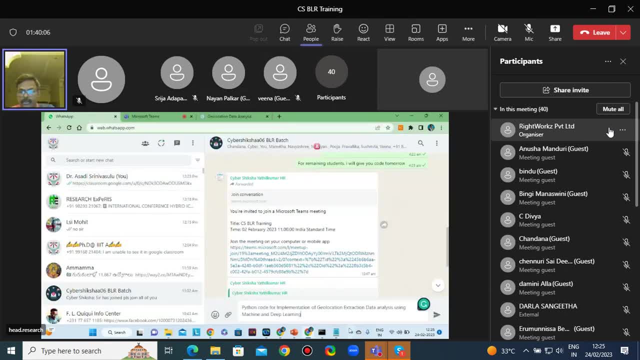 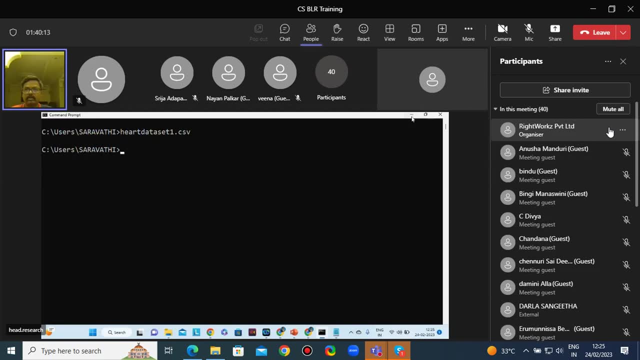 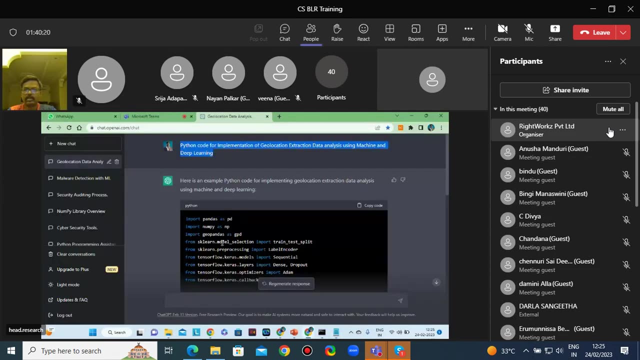 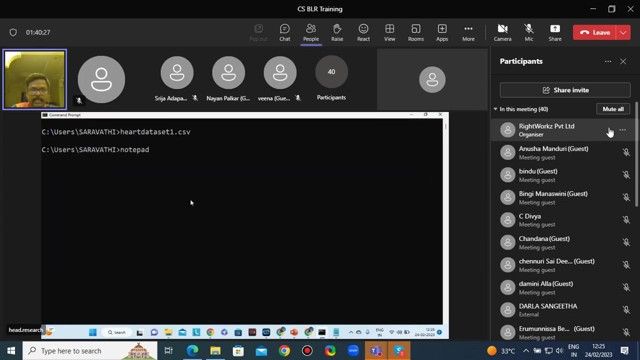 WhatsApp. the aim of the program is this one and code I am sharing with you code. see, here I am sharing the code. Ok, now you can create. see, just I am creating notepad space: geolocation, geolocation dot. 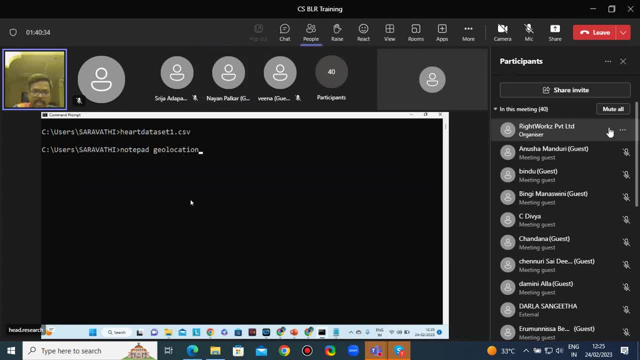 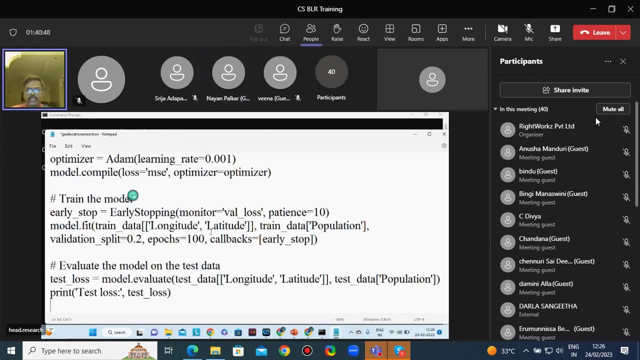 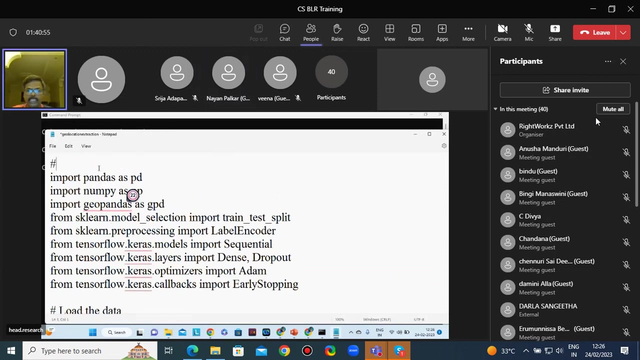 or extraction, geolocation, extraction dot py. Ok, I am creating the file. so this is the. so aim of the program is exactly to create ok. Ok, the hash. I am writing game of the program. python code here. please write down. 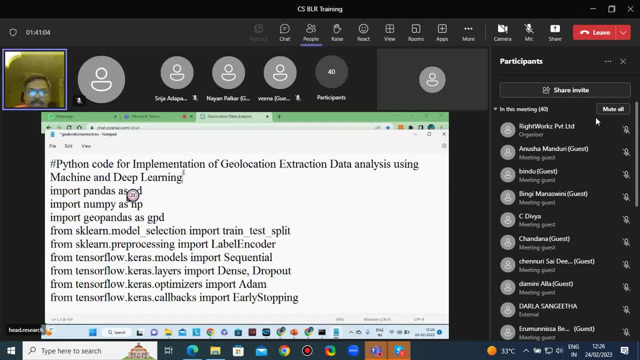 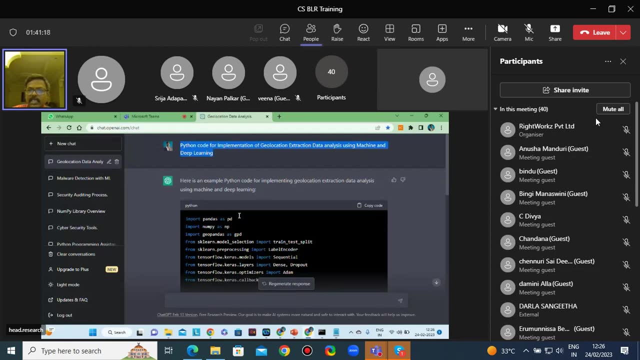 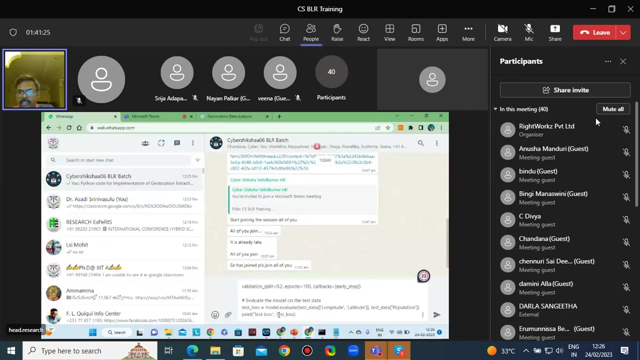 python code. python code for implementation of geolocation extraction data analysis using machine and deep learning techniques. ok, so now I am closing this one. save, yes, and you can check this code in the whatsapp. you can also create this file and try to execute if any data set is available. 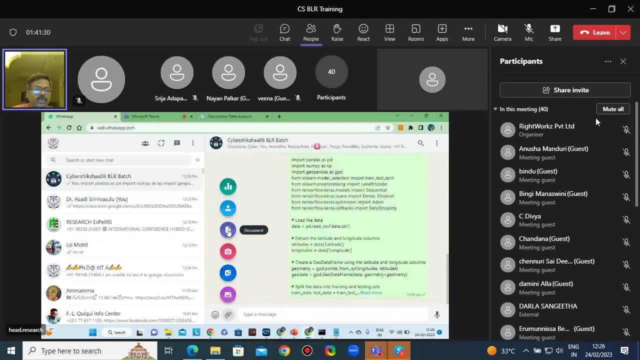 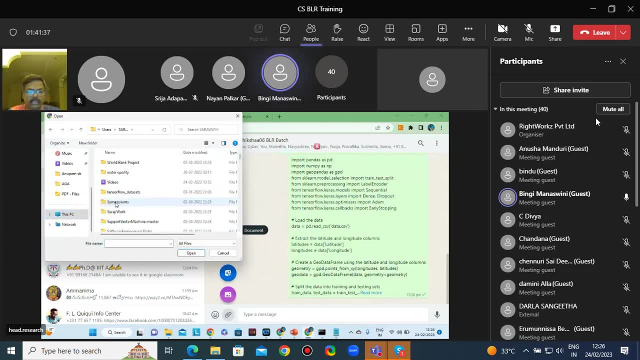 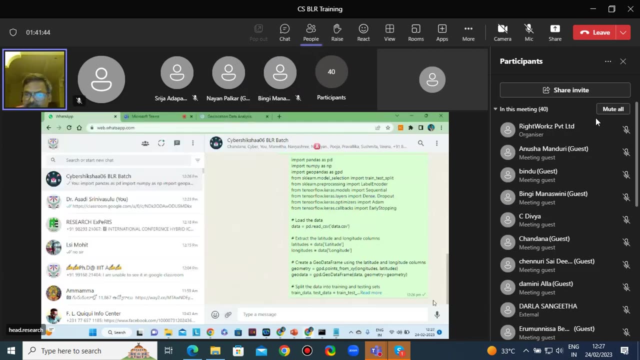 next: next, who's code? whom do you want? next code: geolocation, geolocation. I am sending the data set and I am sending the file also. please download and try to execute now any small data set you can take and execute later. we will take excellent data set. 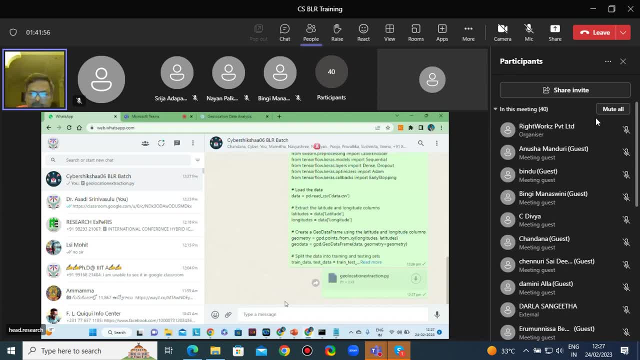 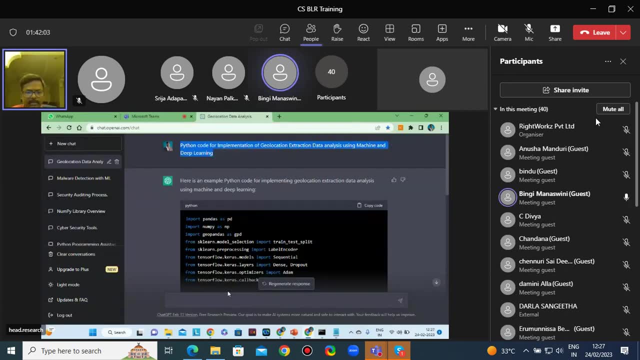 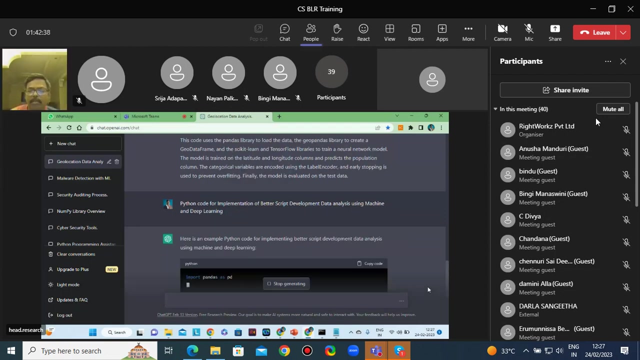 first two, three columns you can take and perform your own data set. next, who's next project? tell me better, better, please speak. better script using MLM. better script, better script develop development data analysis using machine and techniques. it will generate automatically our code, but in this code you need to do: 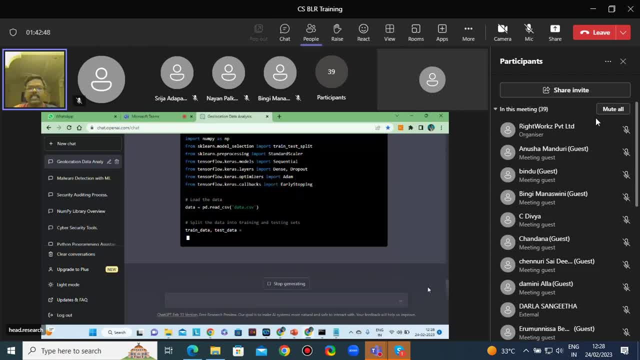 our analysis and our information. we can keep it. ok, so we can keep the code in this code and we will keep our code in it. ok, so we can keep the code in it. ok, so we can keep the code in it. ok, so we can keep the code in it. 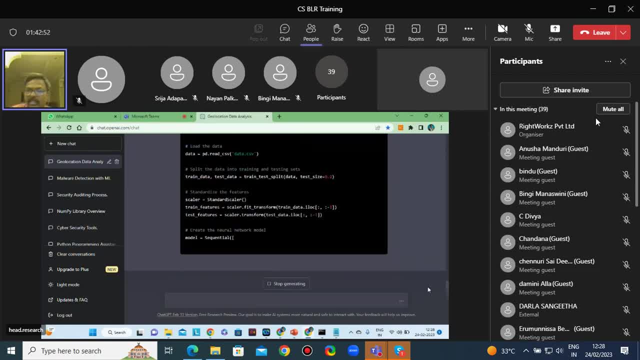 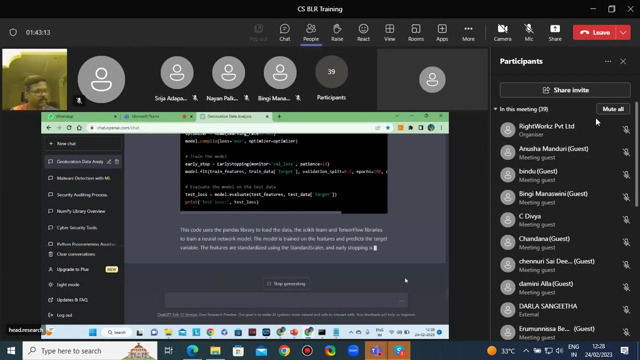 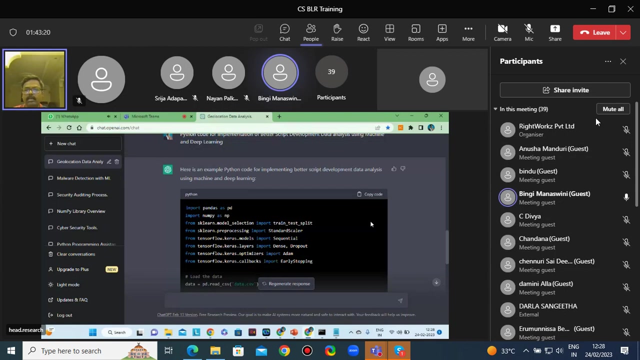 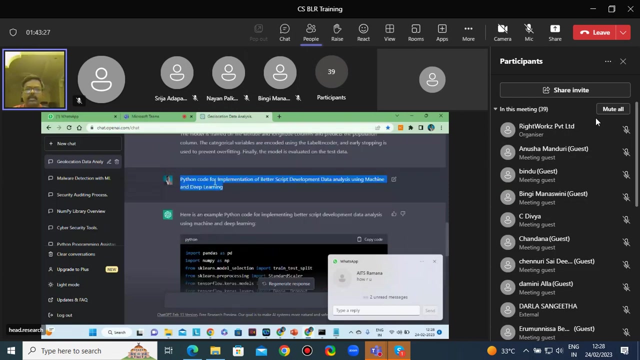 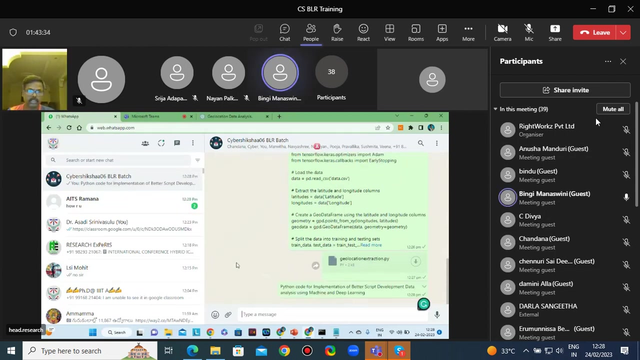 We need to take the data set. that's all remaining things. it is performed Now, so I am generating the code for geolocation extraction. so now I am giving ok, please do all of you. who is this python code for? ok, who is this Manashwini or no? who is this? yeah? 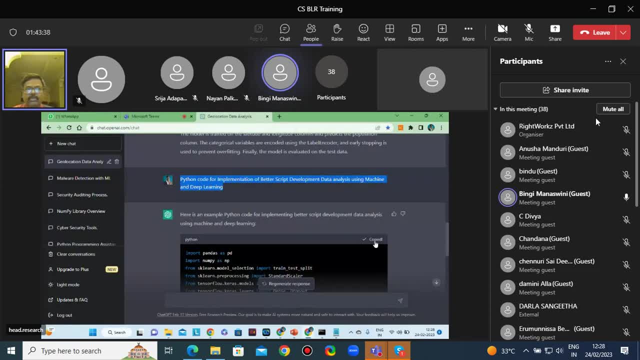 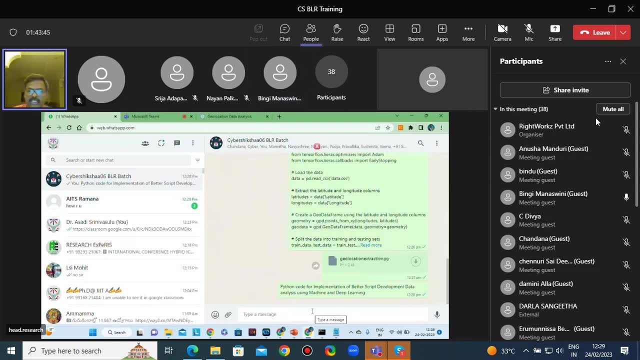 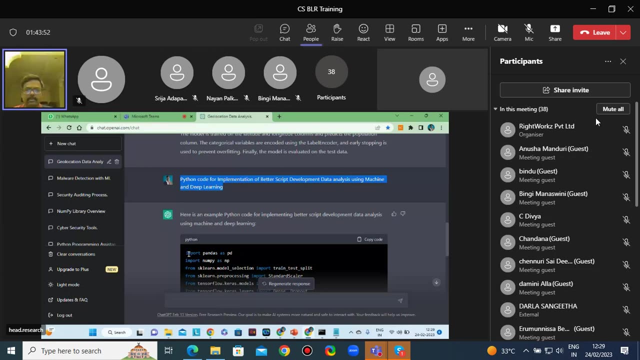 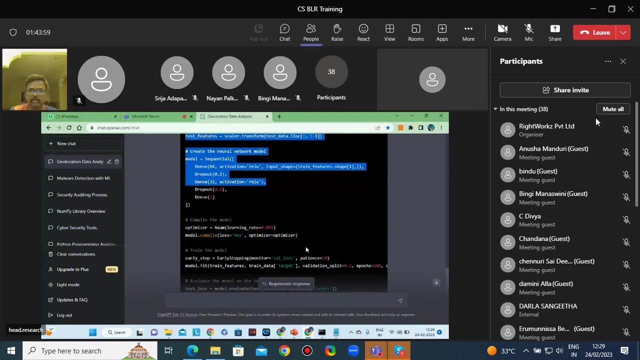 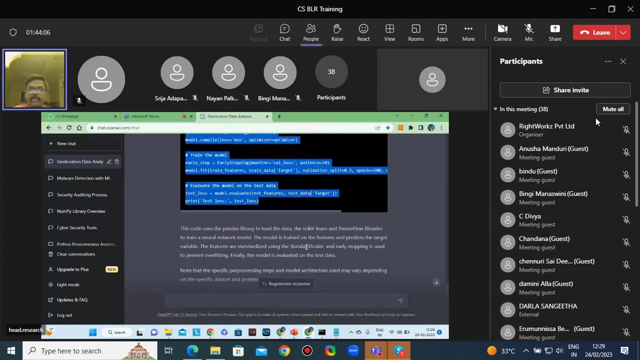 Manashwini, I am sharing your code in the group chat. please take and create. I am creating a notepad file also. please check now and I am copying this one. I am copying this code evaluation, so try to understand every, each and every comment is presented here, so notepad. 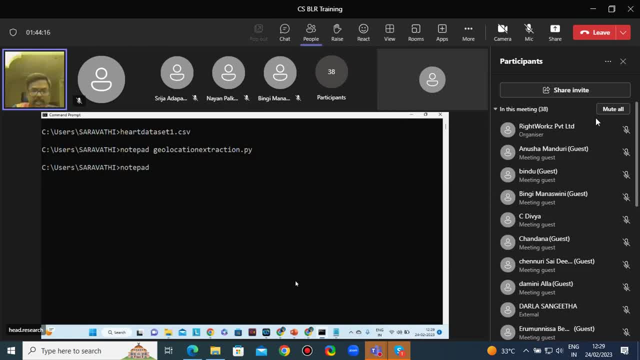 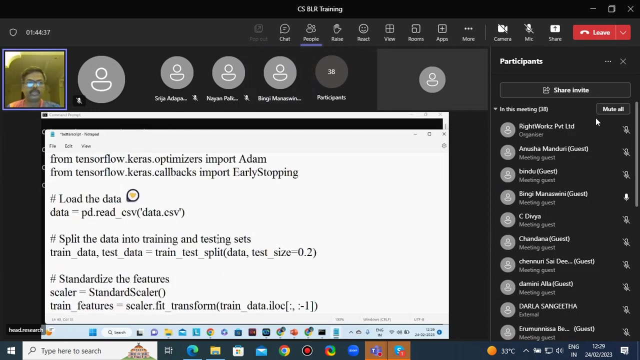 space. What is that you are copying me? better script, better script, better script level of 9? yeah, better script dot py. I am creating the file better script dot py now. so this file I am setting to you. ok, so now try to execute and find out. any errors are there you need to. 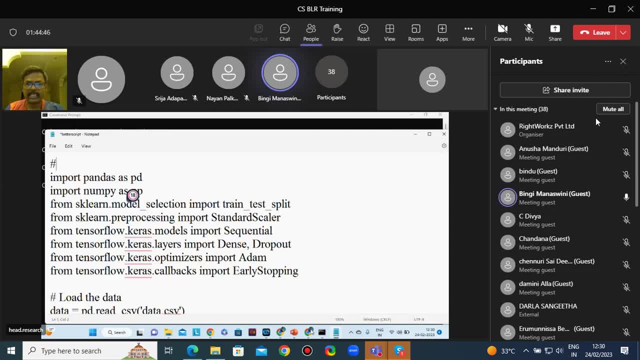 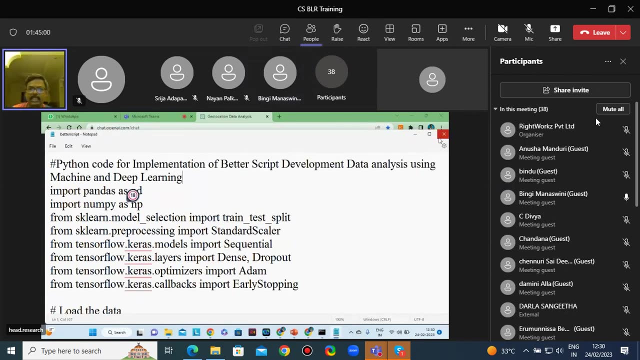 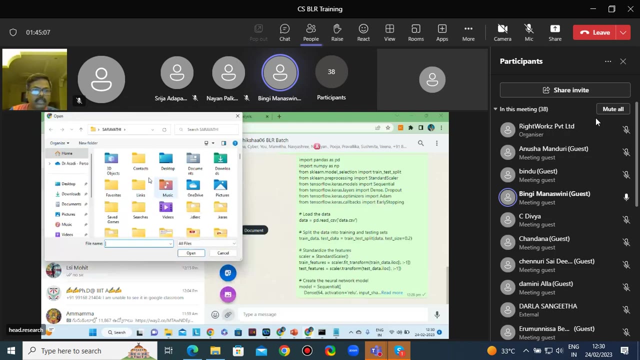 find this. so please be completely. you need to tomorrow and day after tomorrow you need to execute the complete project implementation. please try to execute. ok, so I am sending the file. also, don't worry, Yeah, any doubt, please ask me. Ok, Yeah, yeah, I will give you data. better script, better script, python file I am giving, so you 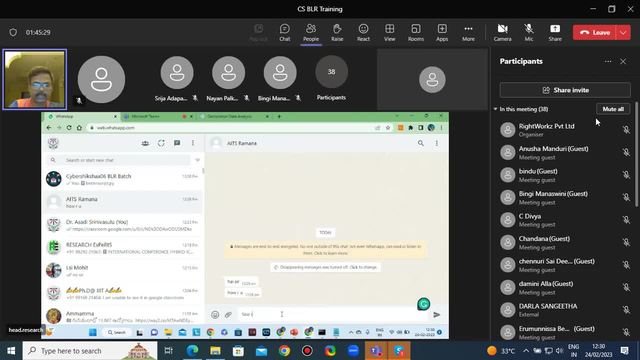 download from the next one. who is next one? next project, Sir. can you give me a project with jupiter book, sir, is that ok? Huh, Jupiter notebook, sir, can I use jupiter notebook? Yeah, yeah, yeah, yeah, yeah, jupiter notebook also fantastic. 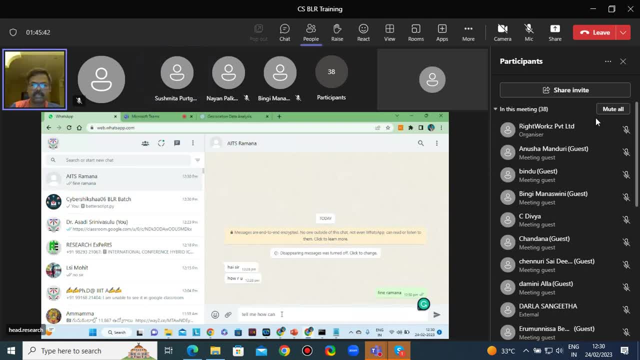 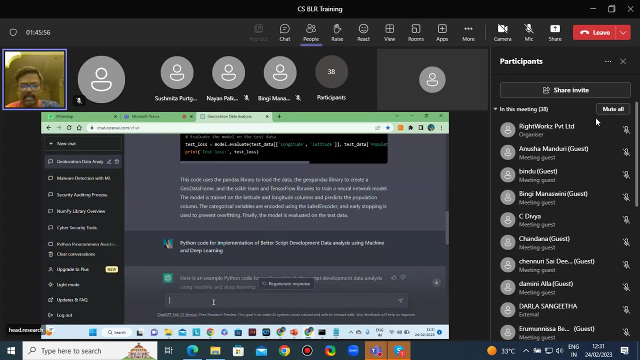 Ok, Yeah, Jupiter Notebook is also fantastic. OK, thank you, Anything, Those are the next project of mine. Whose next project? I think? night I have shared whose mobile security data? Hello, Mobile security data. Whose See? nobody is responding. 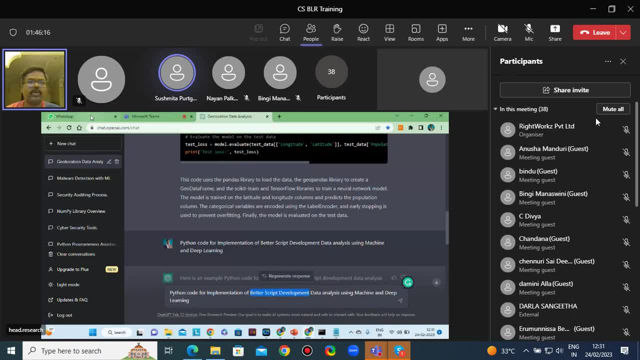 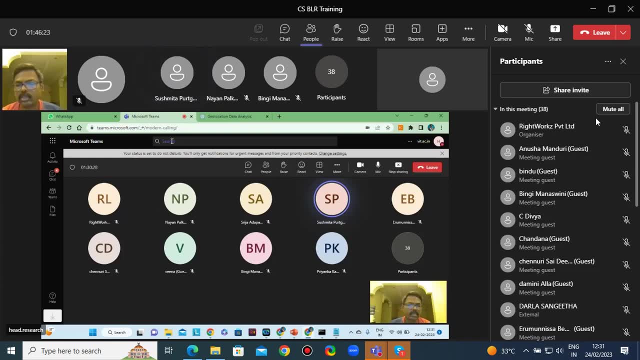 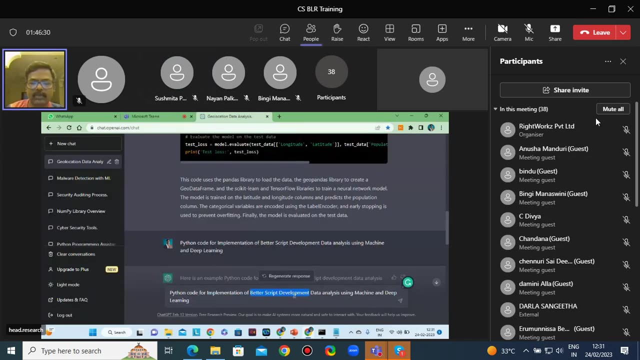 Hello, Mobile security data. I want ethical hacking, sir, Ethical hacking, and You want ethical hacking data. OK, See now Python code for implementation of ethical hacking And data. Yeah, Ethical hacking: data analysis using machine learning. 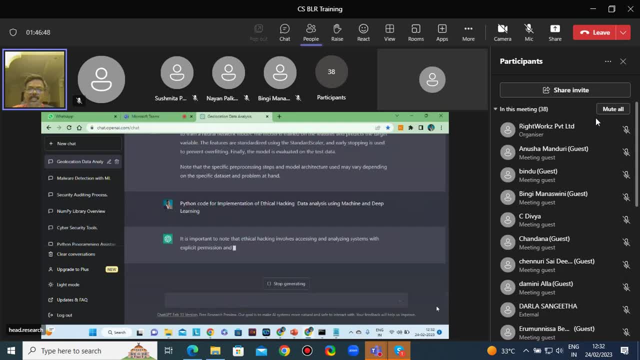 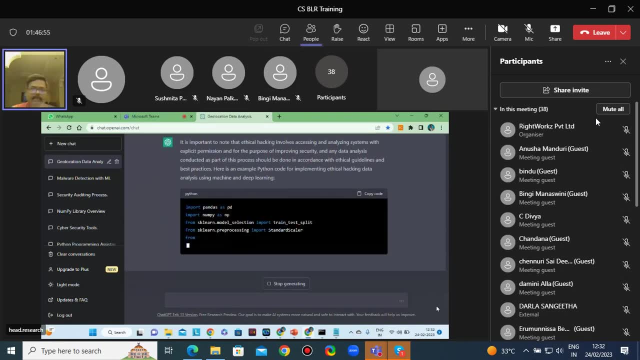 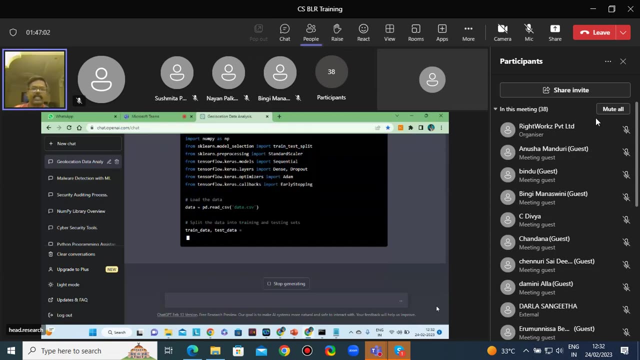 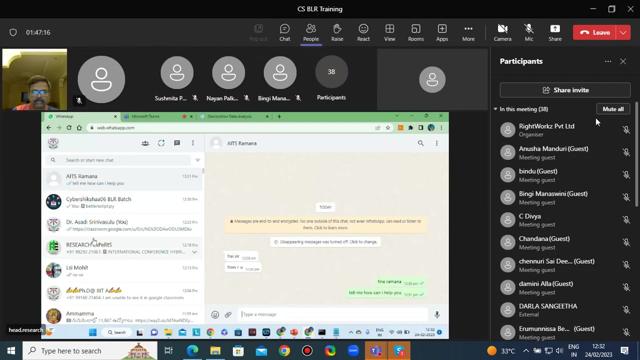 OK, Now see Python code for implementation of ethical hacking data analysis using machine learning and data learning. So now I am giving ethical hacking data set, So data set. I am giving Load the data, Very simple data. So who is this? 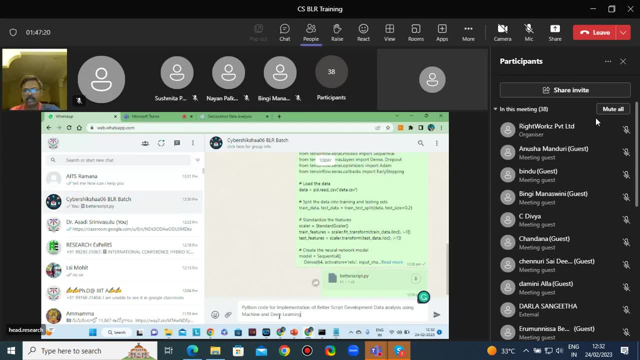 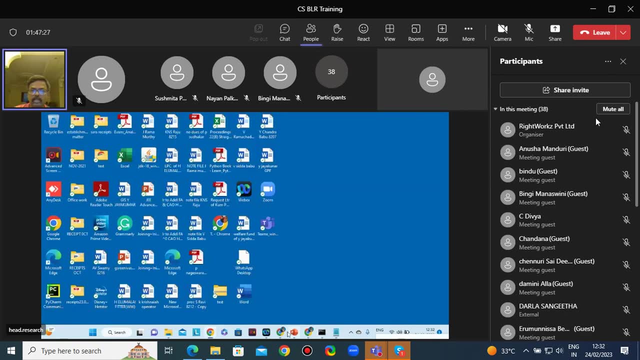 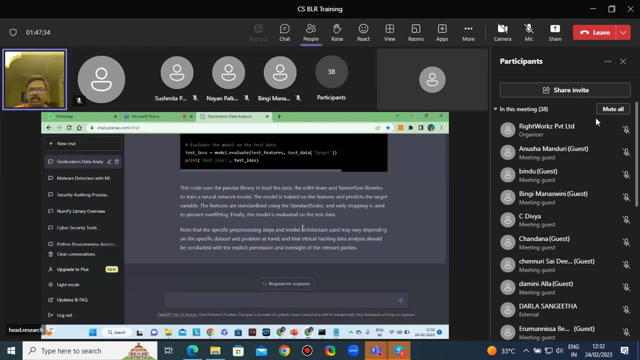 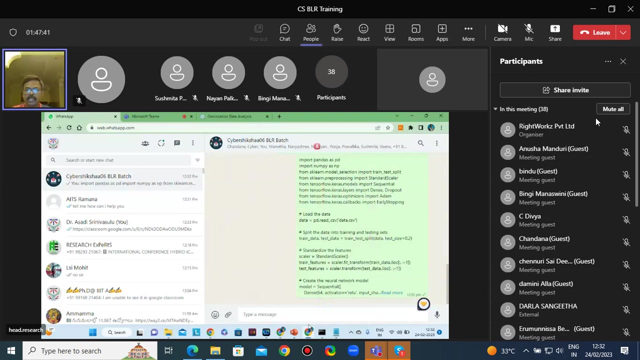 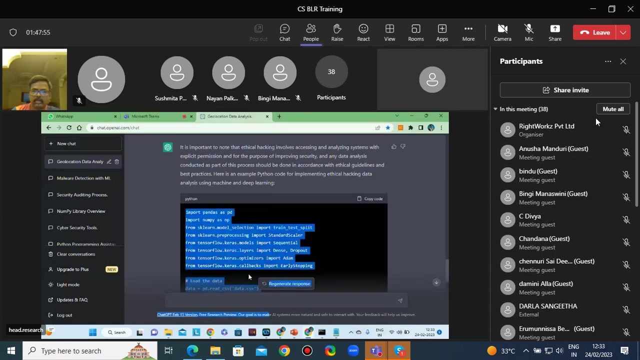 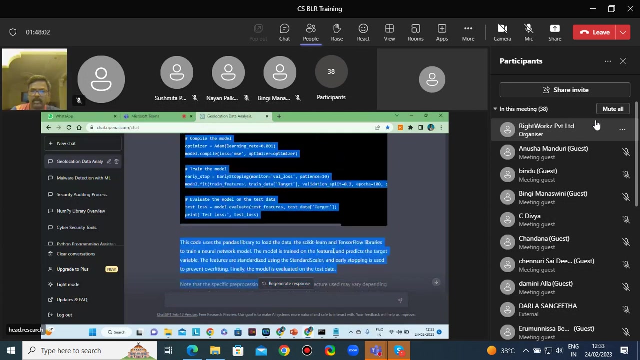 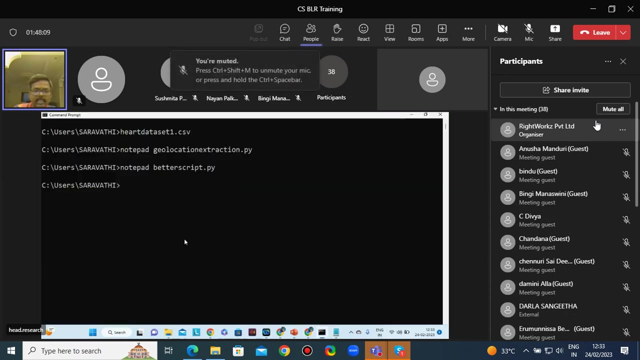 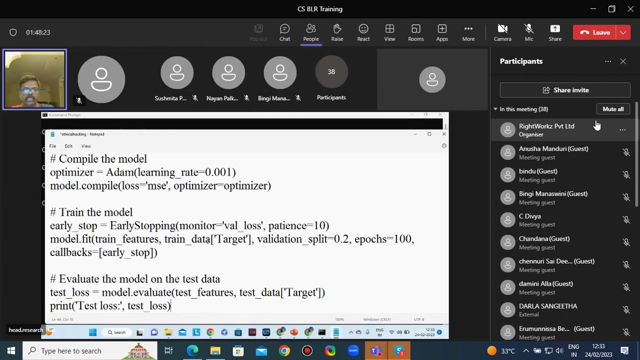 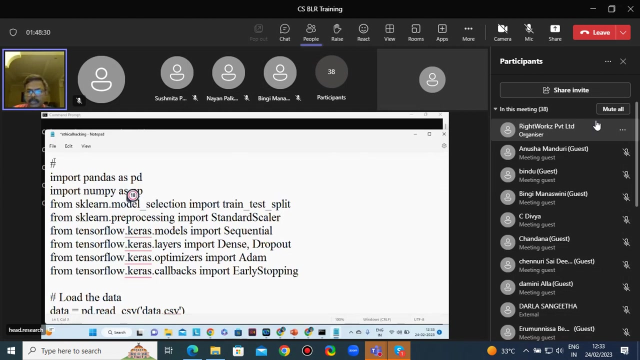 So next batch, Please download. Please check Code I am giving for this batch code. Please try. So I am sharing the code. This is the code. Ethical Hacking- Please see here. Not bad, Not bad space. Ethical Hacking dot V1.. Ethical Hacking dot V1.. So this is the data center. Now see the aim of the program. 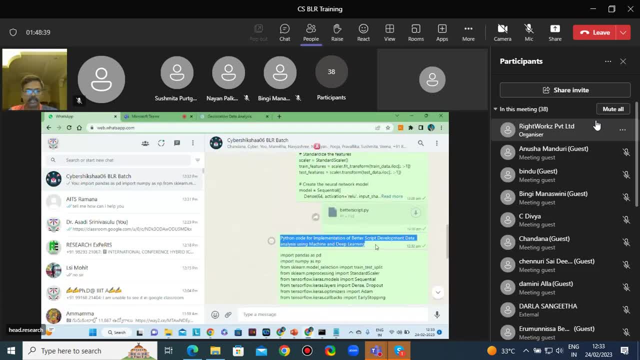 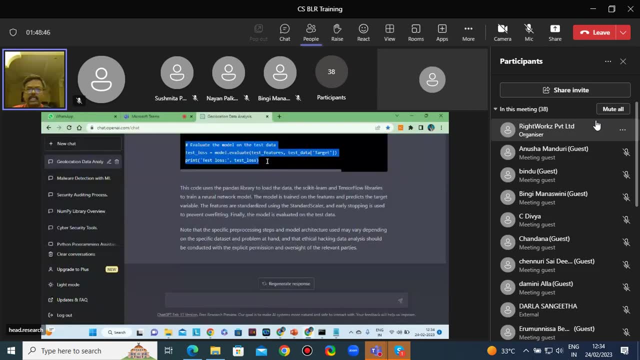 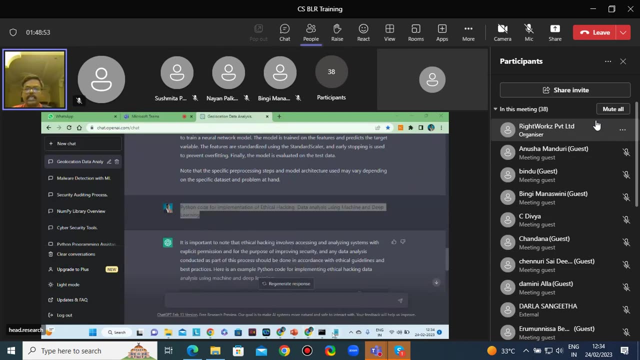 Who is this project? So group 11 project: Group 11.. One second, I am taking this. Okay, This is group 11 project: Ethical Hacking. Perfect, So now I am writing the aim of the program, Okay. 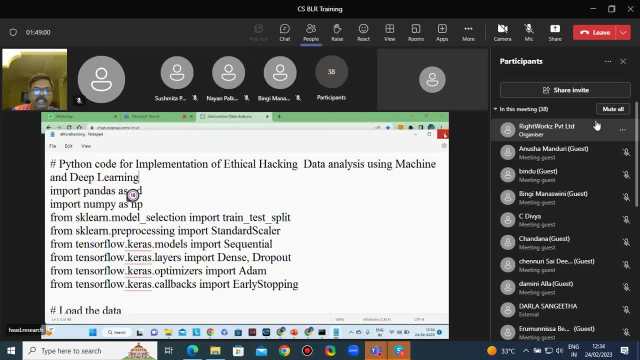 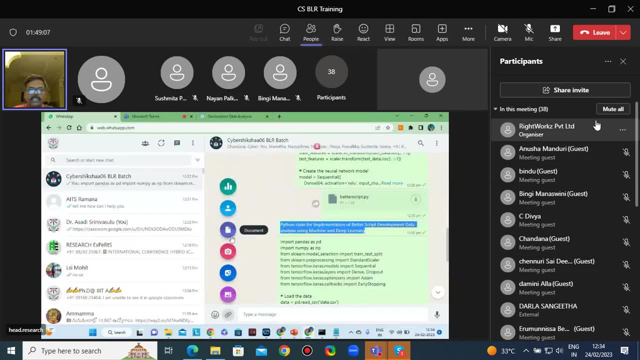 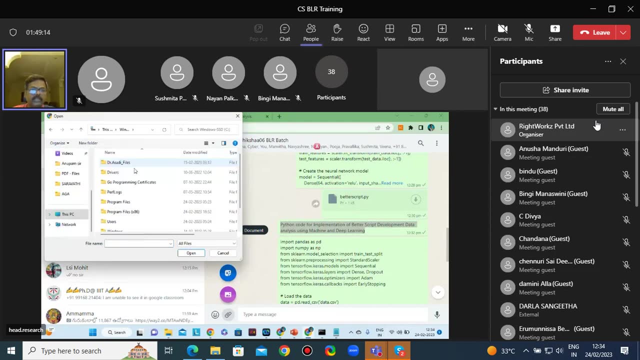 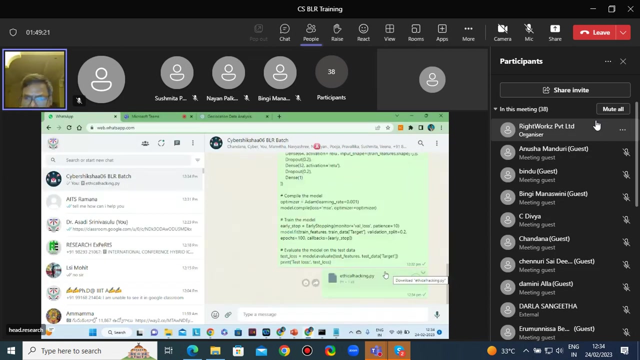 Okay Now please download your data center from the WhatsApp I have sent. So this one C drive users: Ethical Hacking- E stands for Ethical Hacking. Okay Now download. Next any other. Next another project. 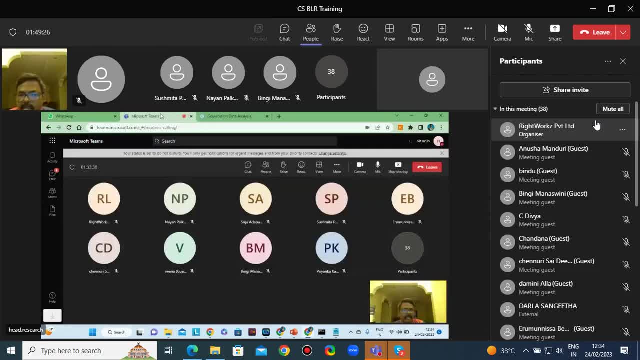 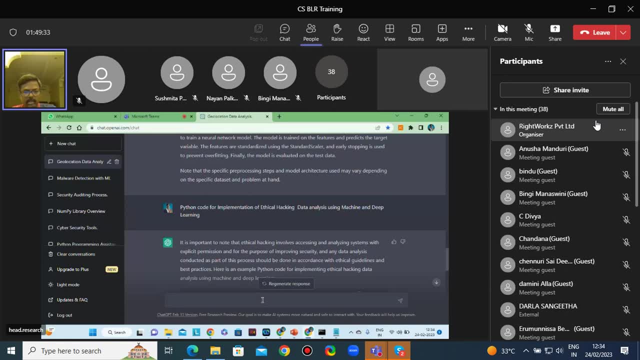 Sir, I think it is monitoring. Okay, Application monitoring Very good, So go to Python code. Okay, So remove this Ethical Hacking. User Application monitoring: Application monitoring- Data analysis. Application monitoring: data analysis using machine learning and deep learning techniques. 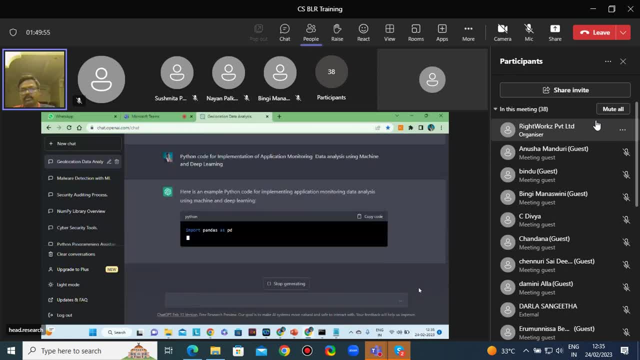 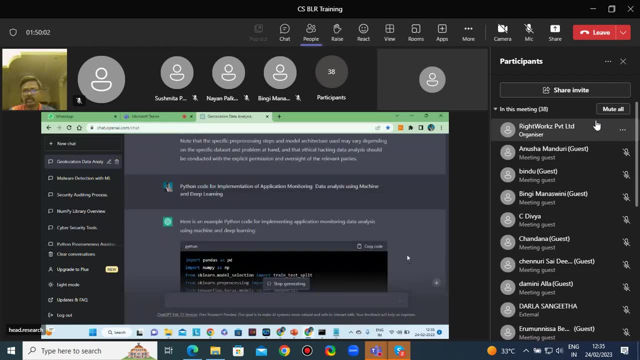 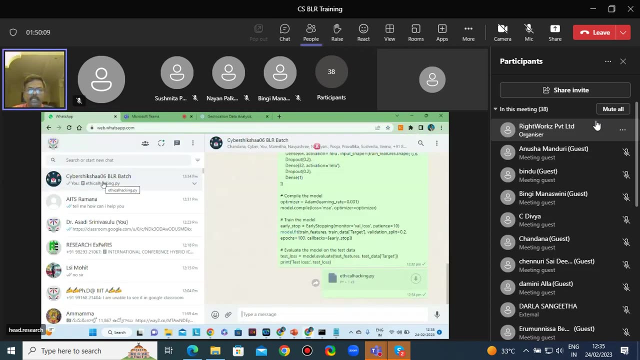 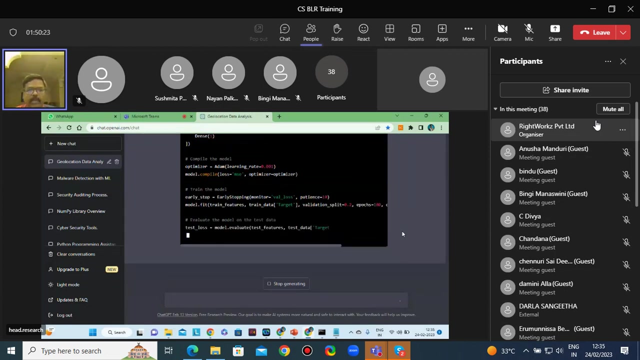 So now it is going to perform. So what is the aim of the program? Application Application monitoring. Batch number. Please download from the WhatsApp Batch number. Choose batch So compile the model. Yeah, Batch number 3.. Train the model: Evaluate the model on the test data. Yes, So this is it. 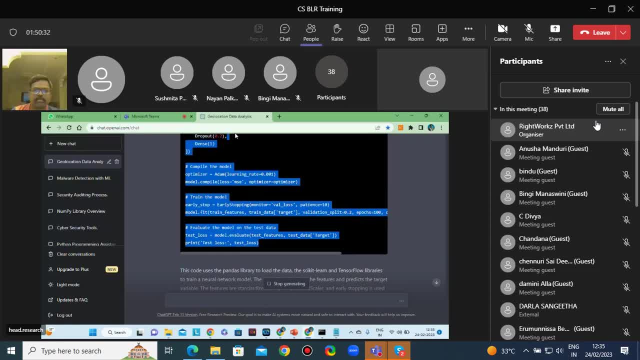 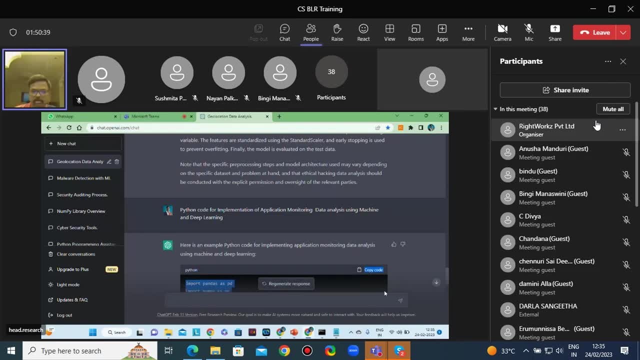 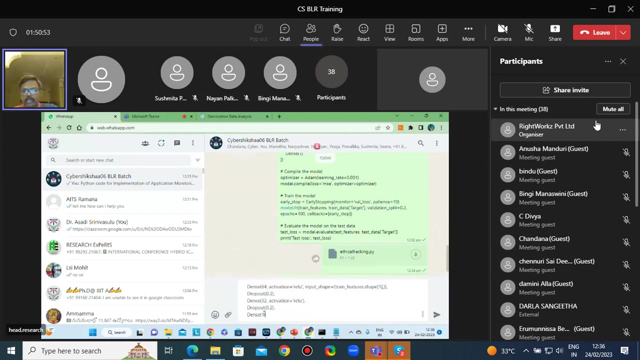 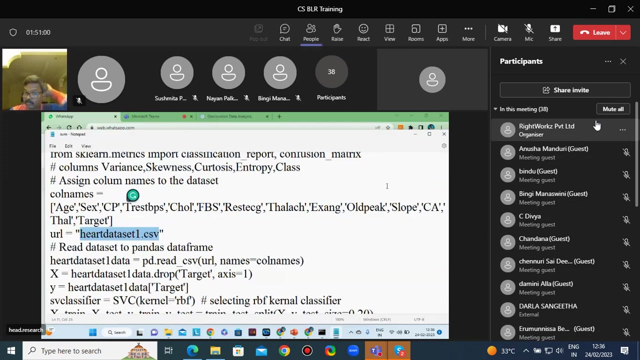 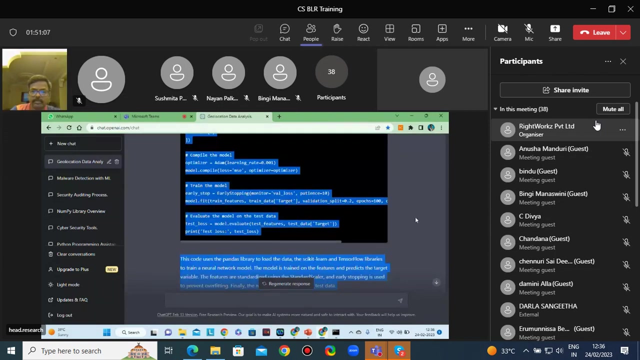 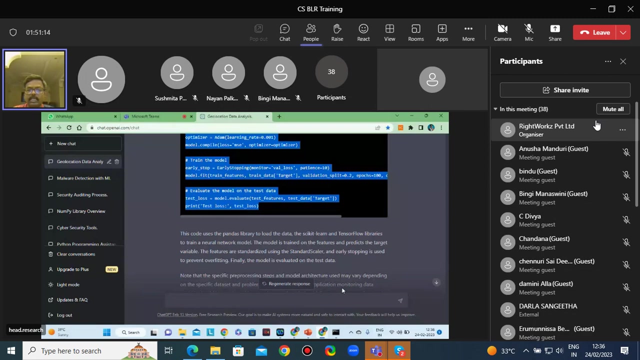 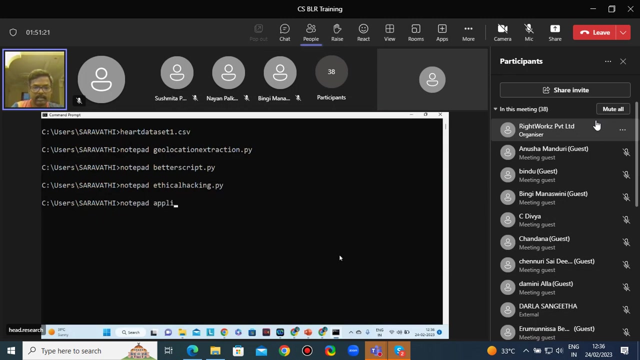 Yeah, Yeah, Yeah. So I am copying this code. I will simply: Okay, Now please download your code and try to execute. I am sending this file also One second. I am downloading. Okay, Yeah, Now, see, this is the code. What is application monitoring? My file name is notepad space application monitoring. 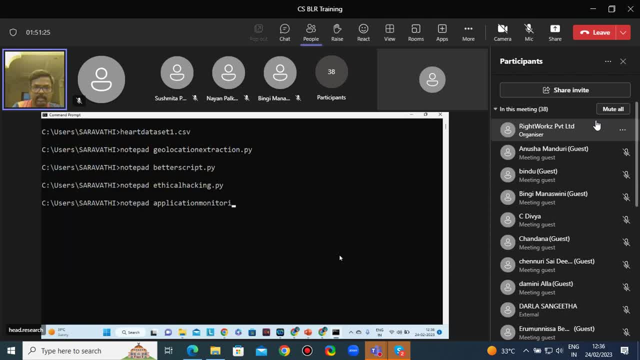 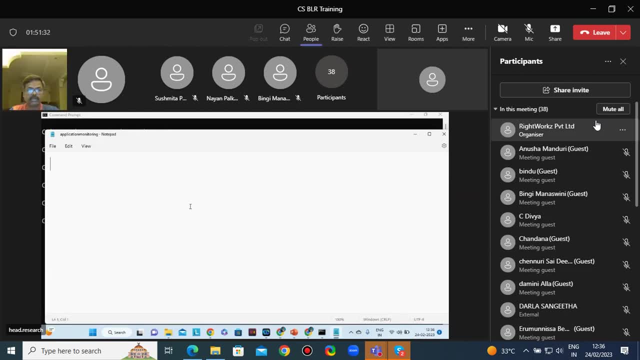 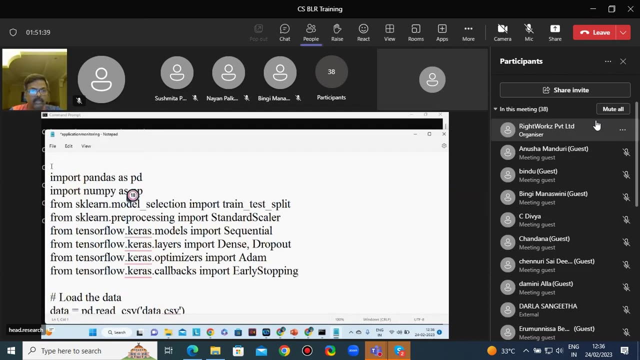 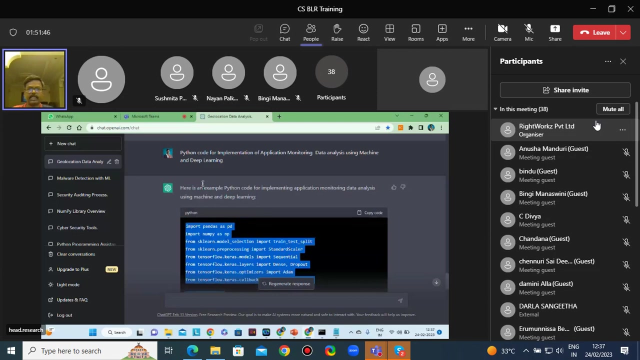 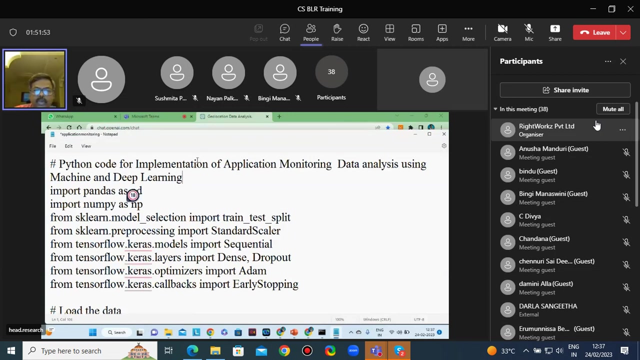 Monitoring, Monitoring The PY. Just I am giving the file for remembering easily: Application monitoring. Okay, So now. Now what I am going to do. So here, comment section, I am writing aim of the program. So write a Python program. Write a Python program to perform implementation of application monitoring data analysis using machine learning. 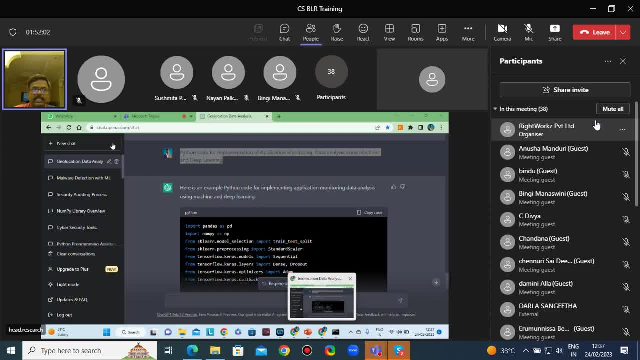 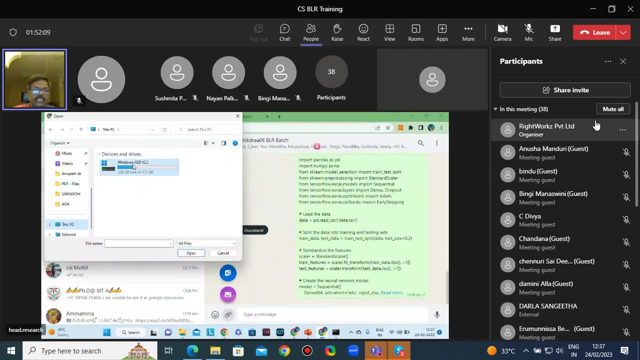 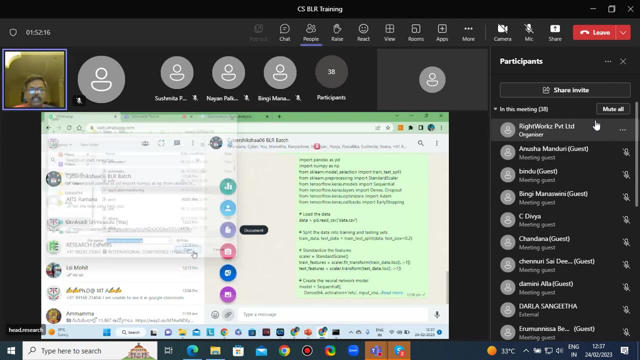 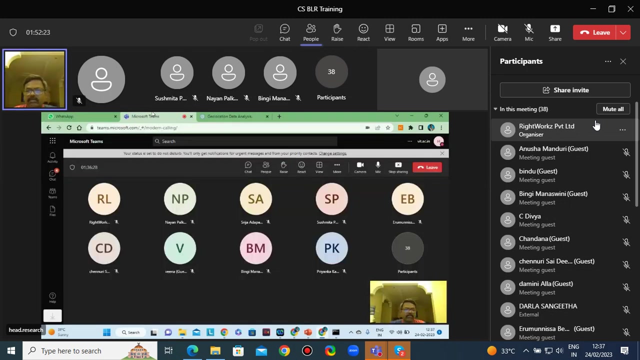 Okay, Application monitoring. Okay, Please download from the website Your file also, I am sending Next, Next, Next, Who's project? Hello, Please tell me. Application monitoring. Next pending: Next pending: Mobile security issues: data analysis. 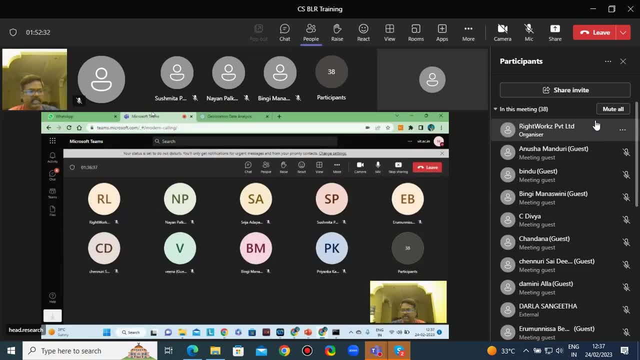 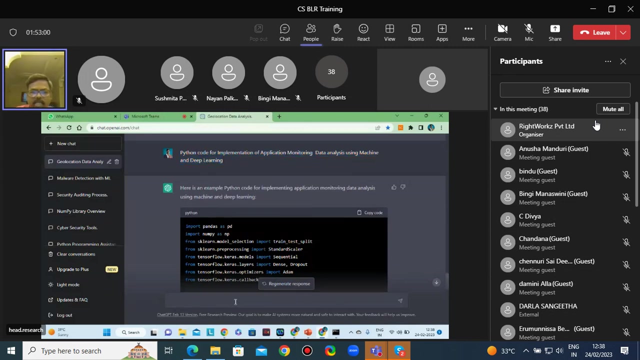 Who is that? mobile security issues? is there anyone? is there anyone with security issues, data analysis, web security issues? please respond. anyhow, i am giving the problem. i think they are not there in this chat room or application monitoring and removing mobile security. mobile security issues or risks. 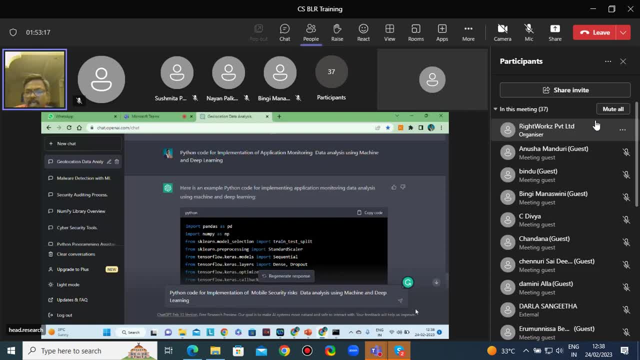 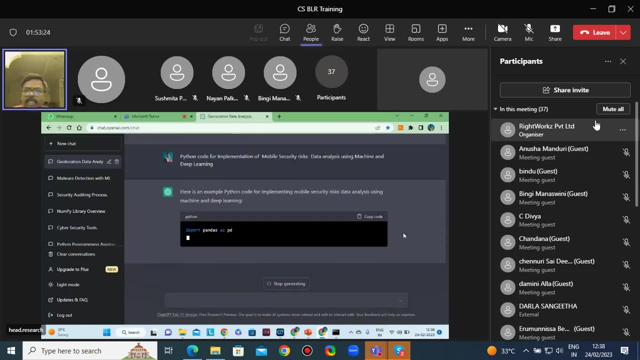 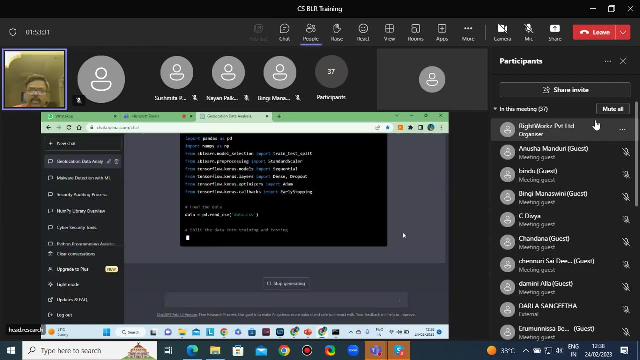 mobile security risks data analysis. python cover for implementation of mobile security risks data analysis. so i am reading datacsv: load the data- this is for mobile security- compile the model, train the model and evaluate the model. please keep in mind. these are the steps we are following in this. 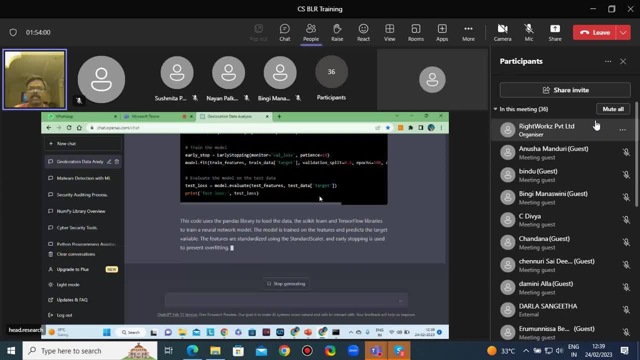 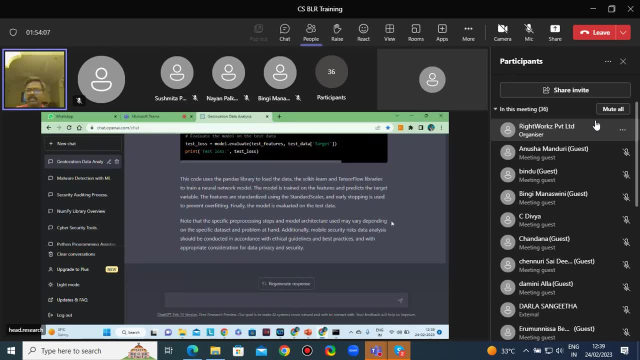 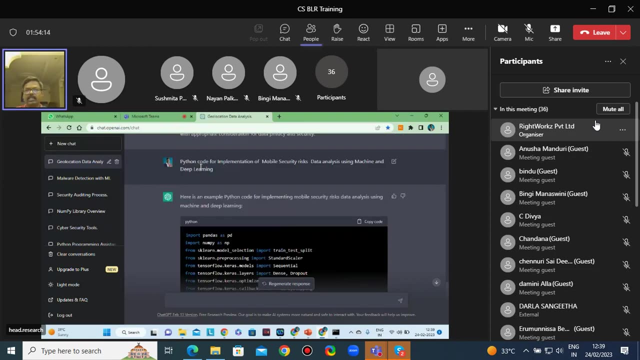 session. so this is the cnn model. this is the cnn model, at least under svm. i have given both algorithms. also, you can include in the code and as well as in the documentation, please. you need to complete within this week and you need to send me the document. 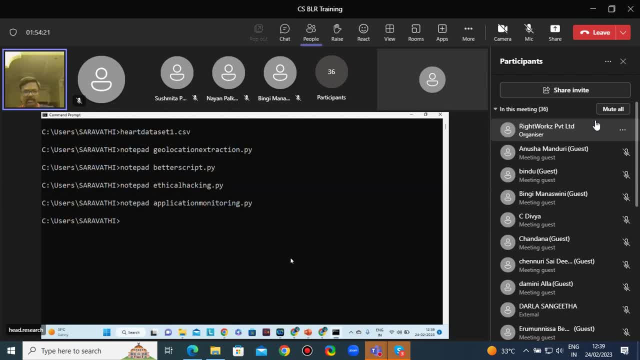 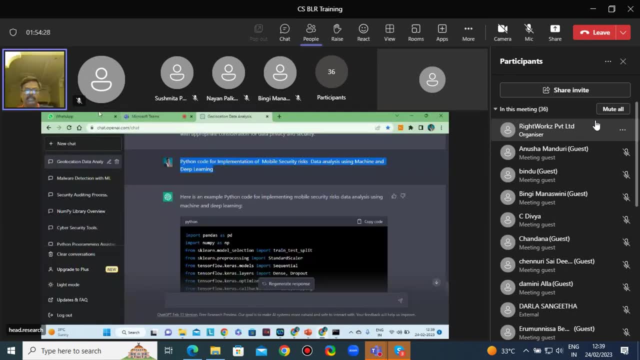 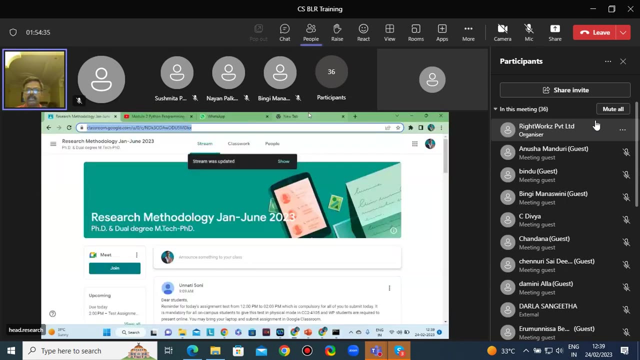 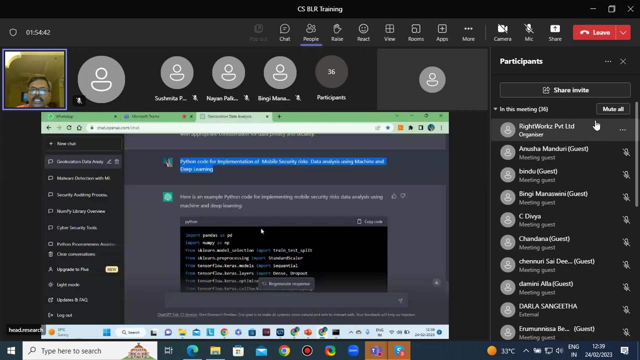 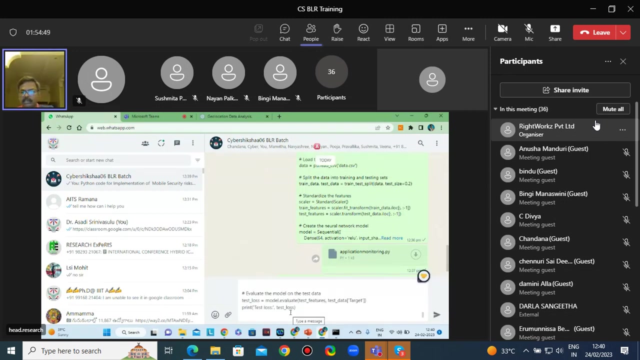 for correction. ok, so i am sending in the group. please see here. please see here: mobile security risks for them. i am sending the. i have sent three members. now i am sending remaining, remaining students, four. you need to create a file. ok, then see, i am creating this. 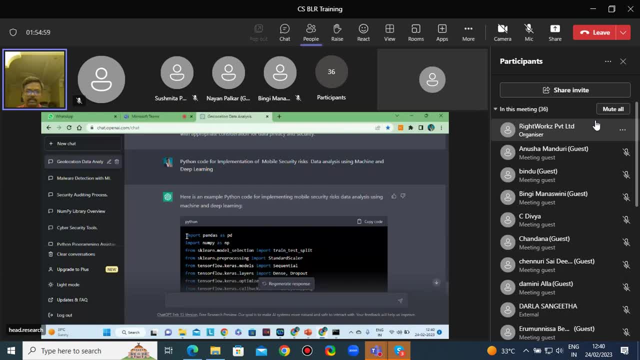 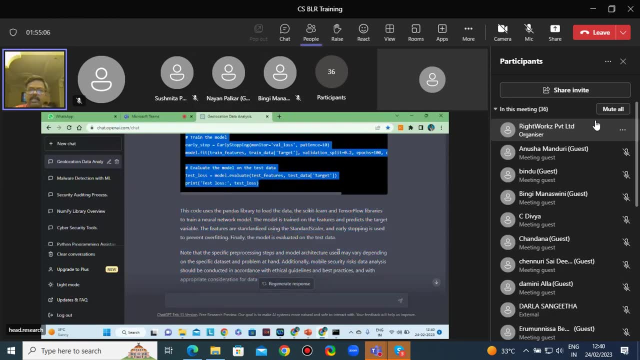 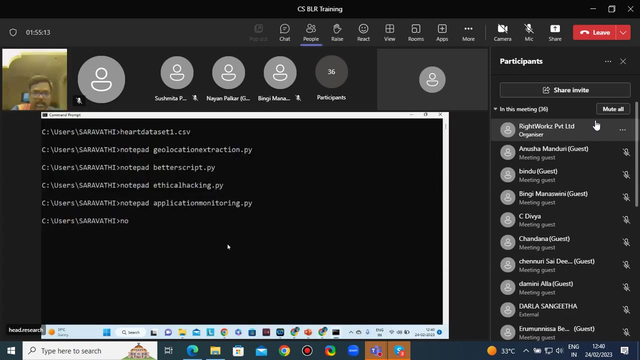 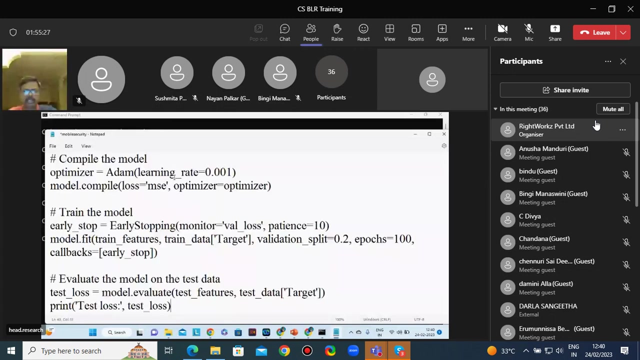 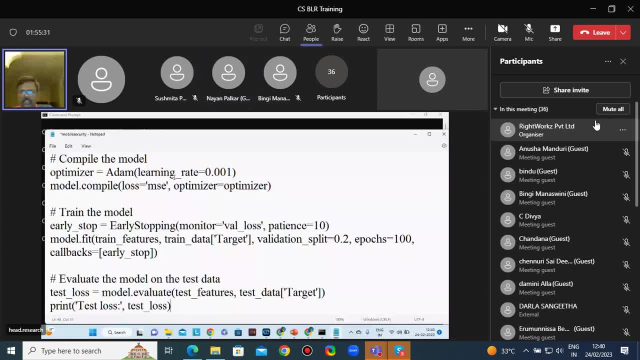 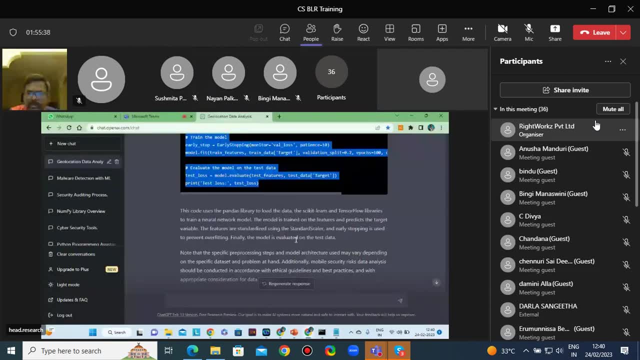 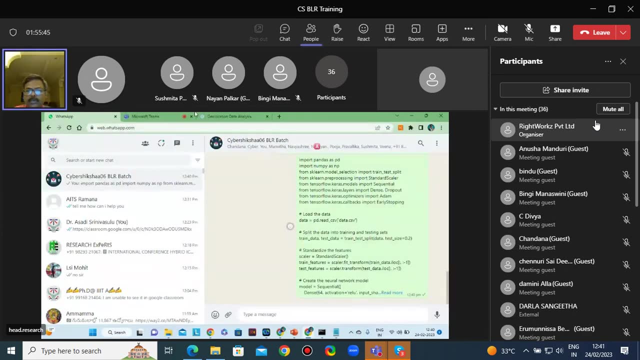 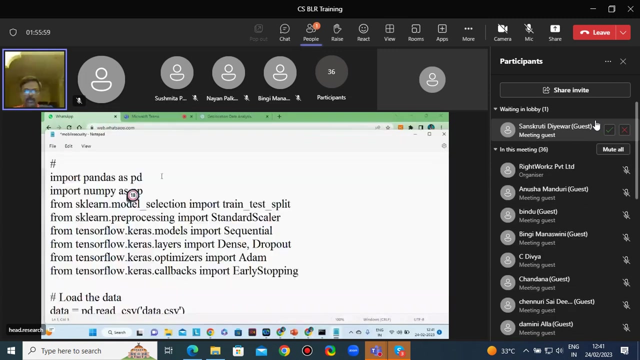 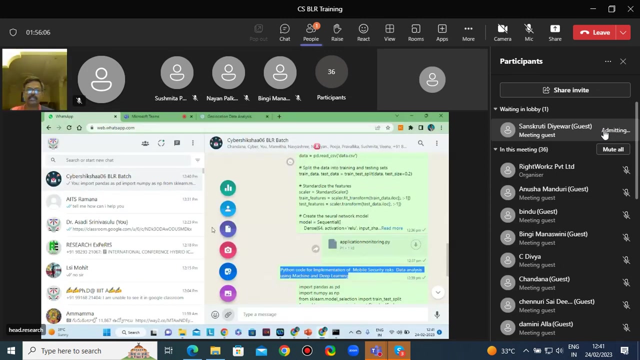 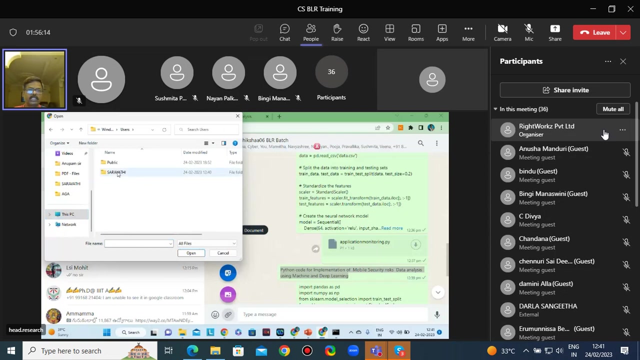 o, please tell me badge, why. why? the aim of the program is: yeah, aim of the program. one second name of the program: mobile security, mobile security risks. next i am sending in the group chart: see users: sarawati, mobile security. there is mobile security. this is the python file. okay, next, web security. 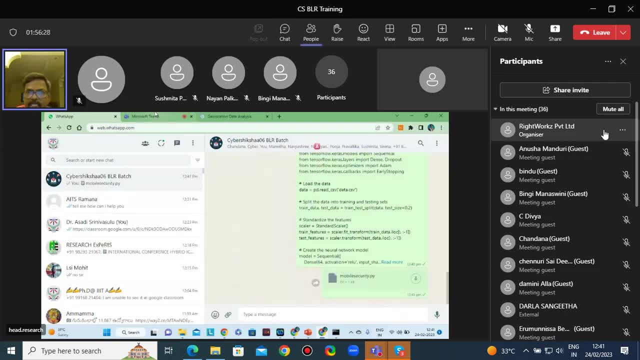 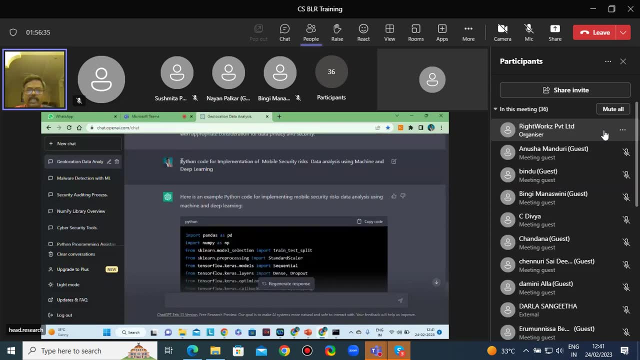 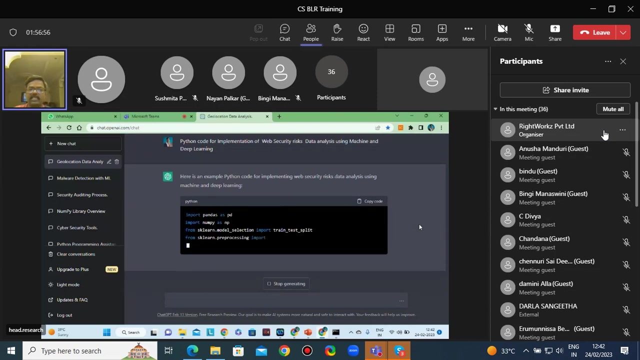 risks data analysis. who's web security? hello, please respond. web security risk analysis using machine learning and deep learning. nobody is responding. why so? excuse me, sir, so implementing at that time i'm getting errors. so, yeah, yeah, we'll see. we'll check. we'll check, don't worry. first you need to collect the data and analyze the columns. 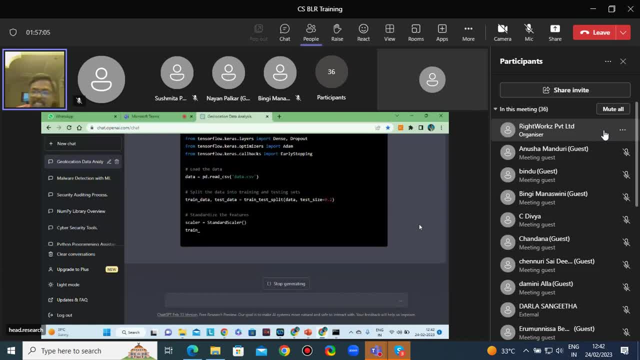 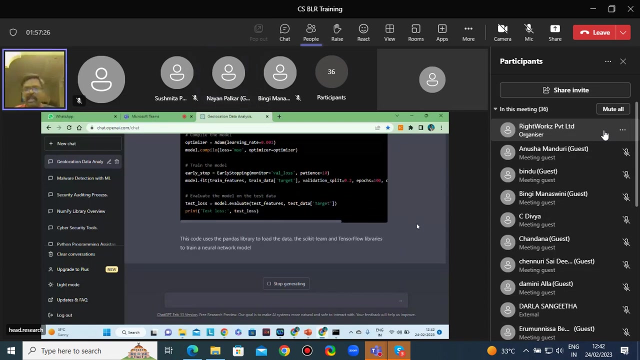 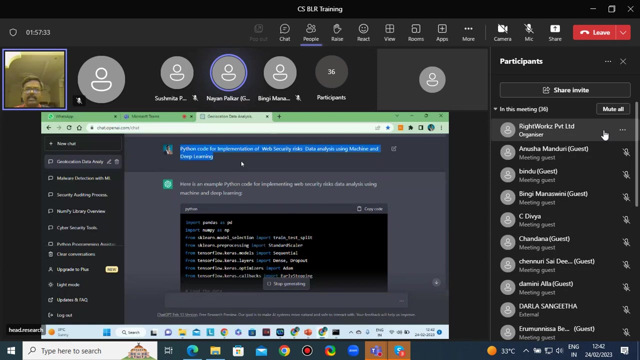 you need to analyze the comments, because your data set columns are different. yeah, definitely don't worry. no, sir, it is giving like a no model named pandas, like that, but pip install pandas, that's all. but still it is giving like that. okay, i will, i will do it first. try. first try to write: install pandas or pip install pd. 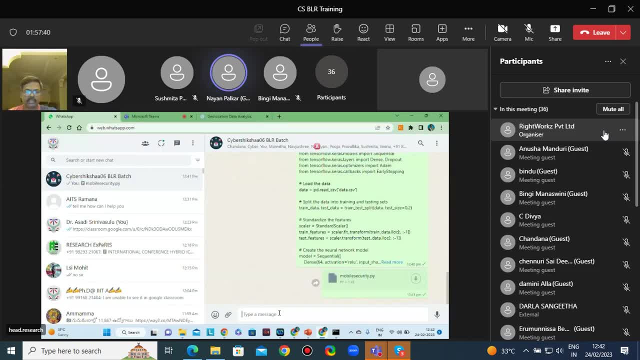 still it is giving same error. yeah, so we have to write pip: install pandas, goal of pd only first installation. i will, i will ask you to share your screen. please wait some time, i'll, i'll. i'll call you next. who's the security risks data analysis. 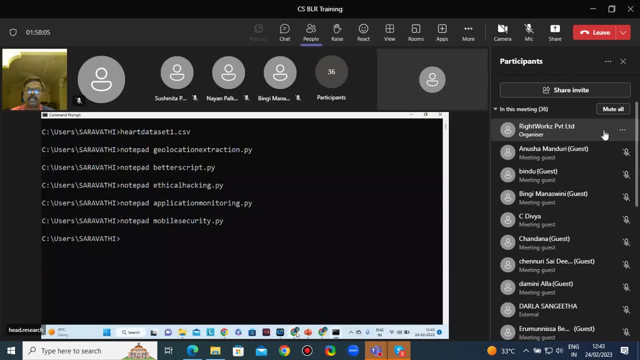 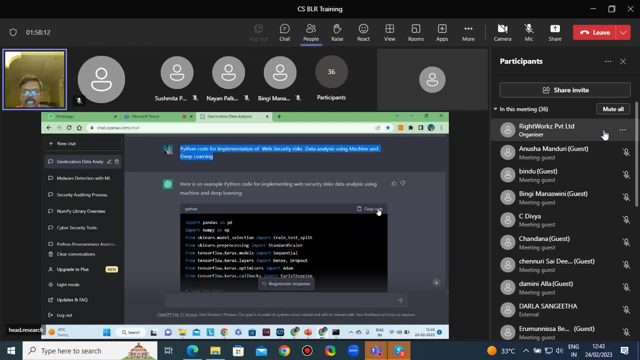 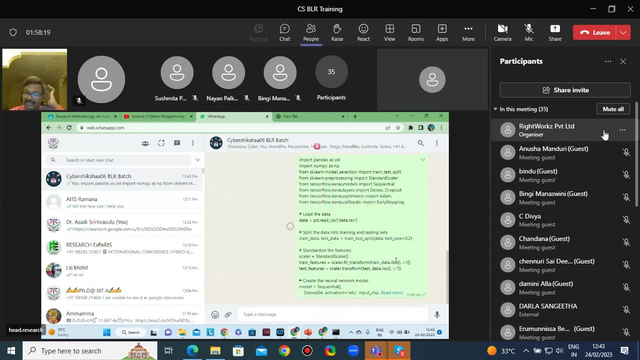 please see here i'm sending the code, please. i think this is the last project. can you check, uh, how many projects i have sent? please count so far how many projects code i have sent. okay, sir, say, wait, call you. check in the group chat. check in the group chat, uh, how many projects code i have sent. 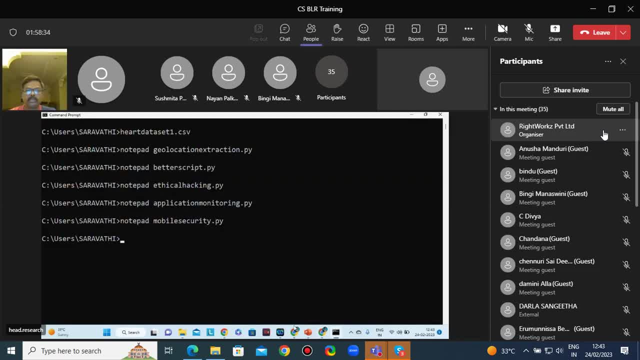 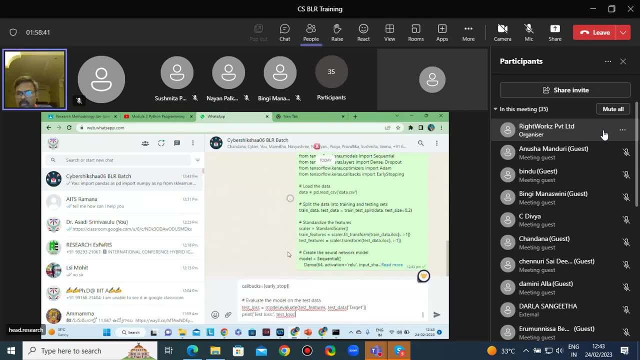 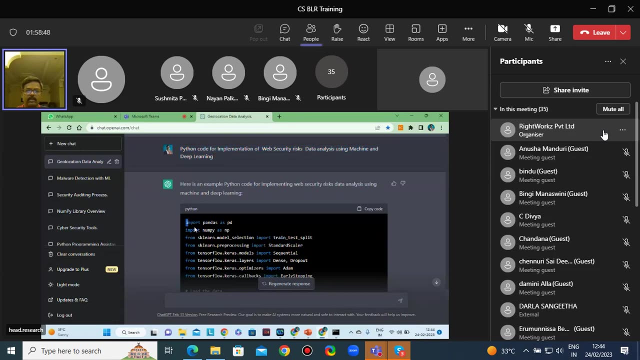 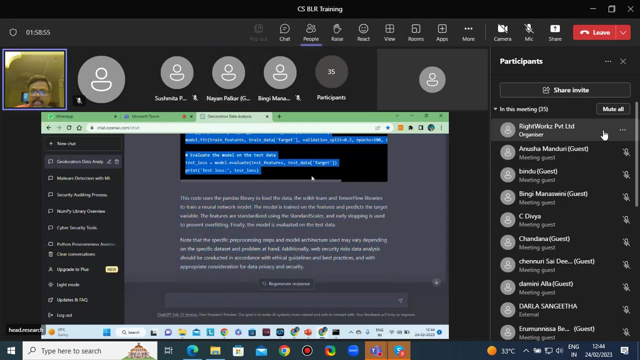 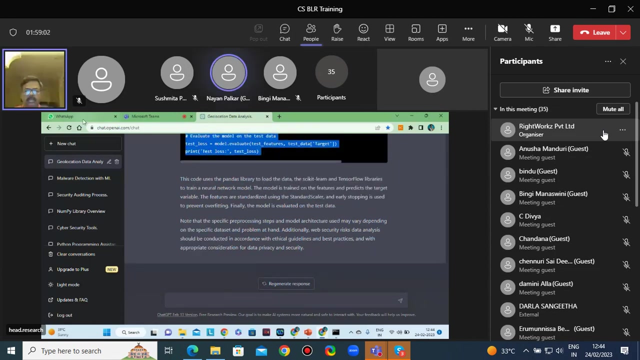 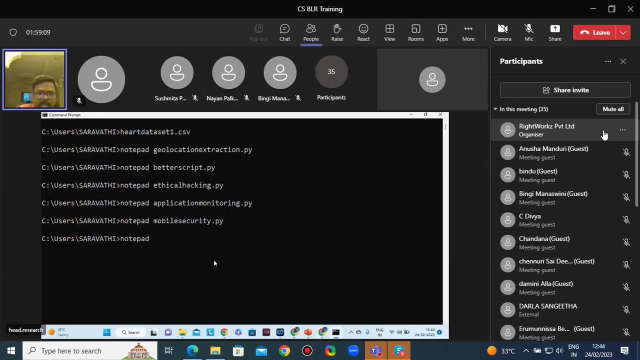 this is web security. yes, this is web security, sir. a codes are there, sir. eight codes are there. night, i have center three, including that one. yes, sir, including that eight. that means that means a few students not yet started their implementation mobile security. now at this three batches, please respond. this is a main project you need to implement. 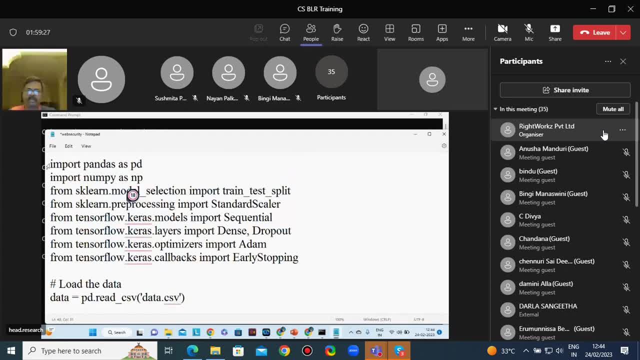 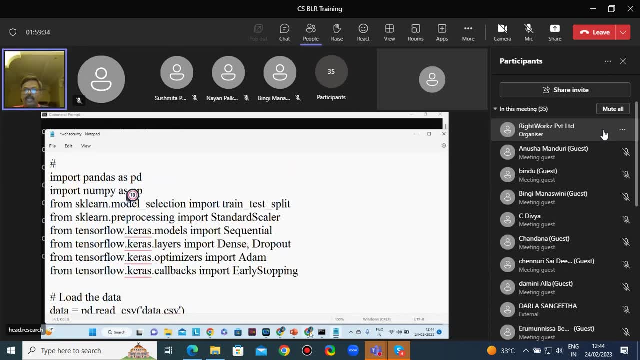 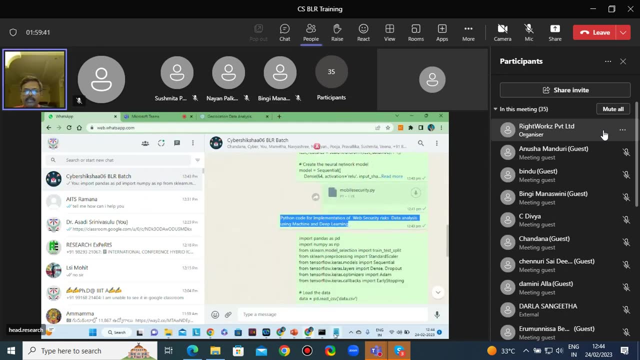 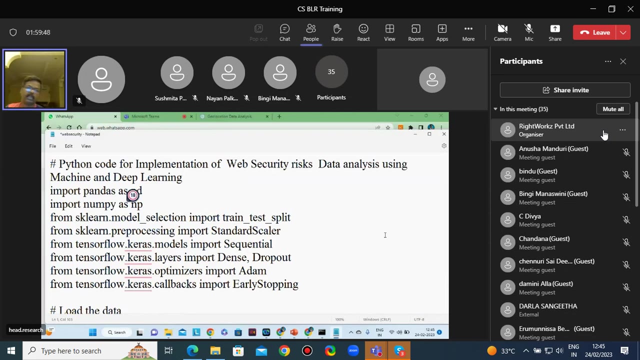 okay, eight batches. next batch: please tell me the problem statement. without problem statement, how i can help you. this is implementation. i think you have prepared, uh, you have prepared already um, what i can say, uh, powerpoint presentation and documentation. okay, this is web security related project. now i am sending a file. 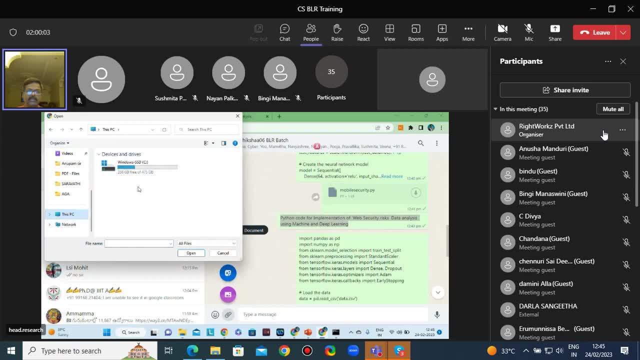 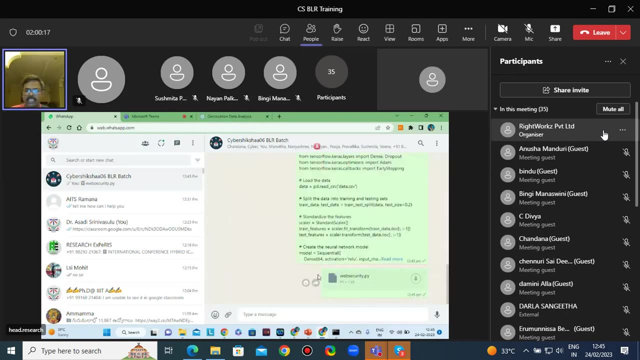 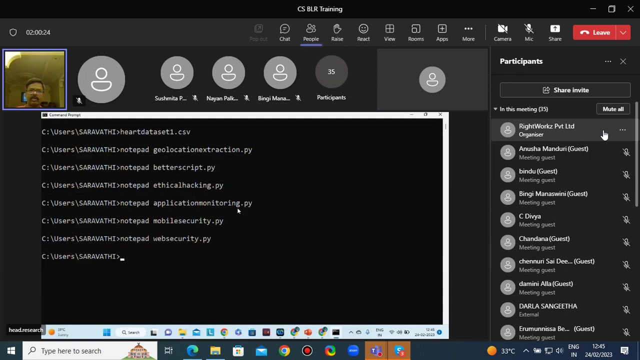 абсолют this pc web security users. web security. yeah now, who? what are the bad? what are the files are? uh, i think i need to check in working. any any batch is pending. any code: 1, 2,, 3,, 4, 5, 6, 6 plus 3, 3, ok, anyone Network code scanning can you explain? 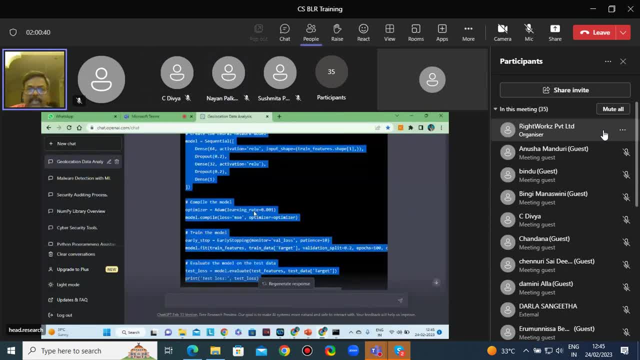 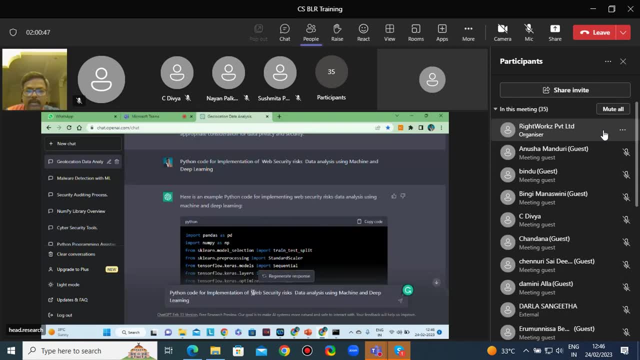 sir, Ah, very good, very good, very good. network code scanning- that problem. I need to give code. so network wait, wait, wait. network code scanning. network code scanning. network code scanning risks. network code scanning. 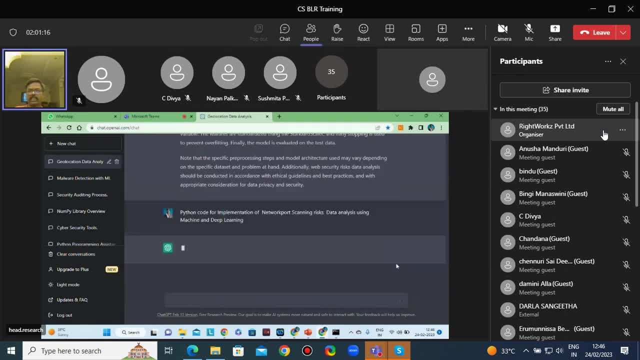 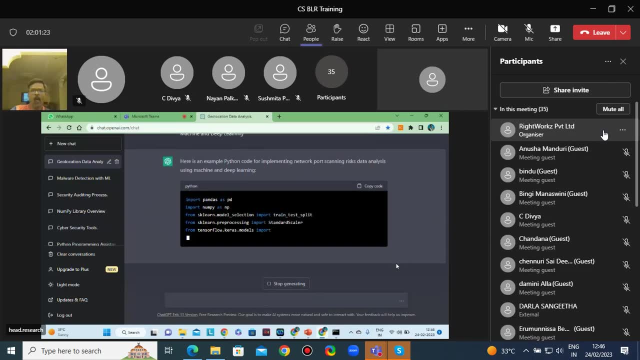 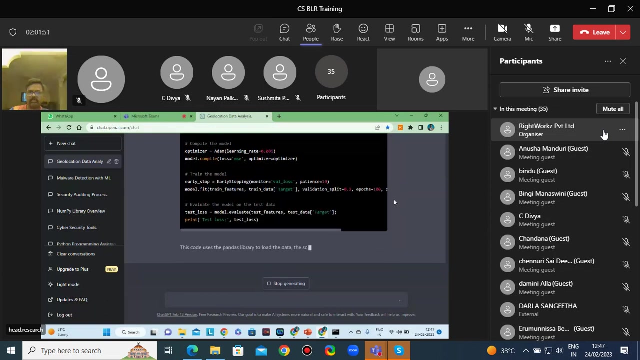 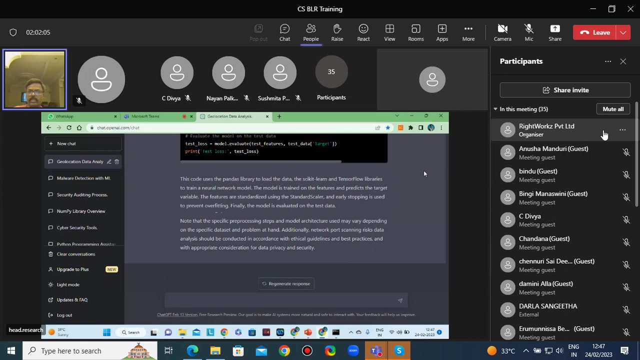 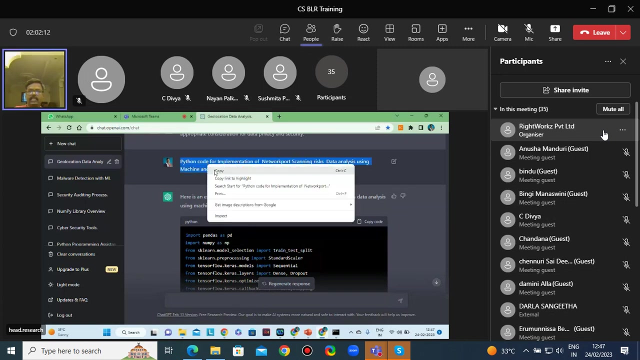 Ok, so now I am sending the python code for a. so pd is a shark pop of pandas. you need to install numpy. next let us see how many 35 members are there: 3,, 4,, 5,, 6,, 7,, 8,, 9,, 10,, 11,, 12,, 13,, 14,, 15,, 16,, 17,, 18,, 19,, 20,, 21,, 22,, 23,, 24,, 25,, 26,. 26,, 27,, 28,, 29,, 30,, 31,, 32,, 34,, 35,, 36,, 36,, 37,, 38,, 40,, 41,, 42,, 44,, 45,, 46 and 47,. 41,, 42,, 44,, 45 and 48,, 41,, 45 and 46,, 39 and 42,, 44,, 45, and 49 and 50, and thoseuf szczegól marks. 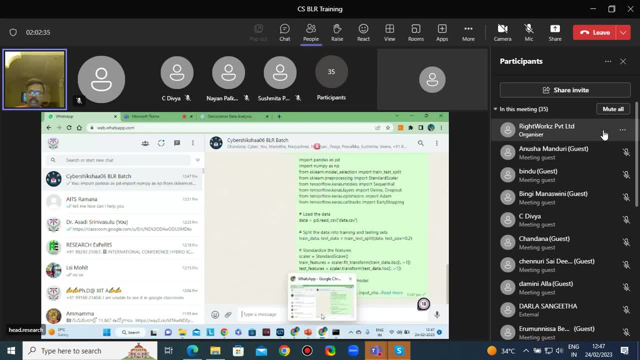 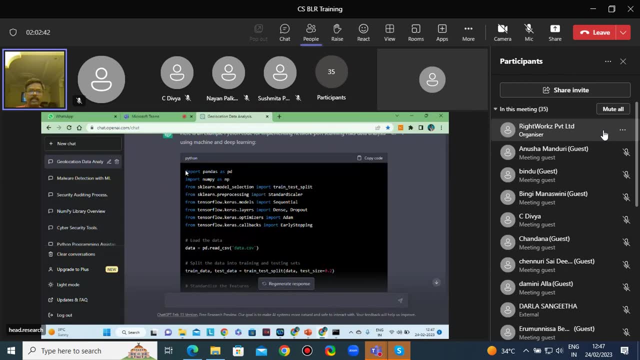 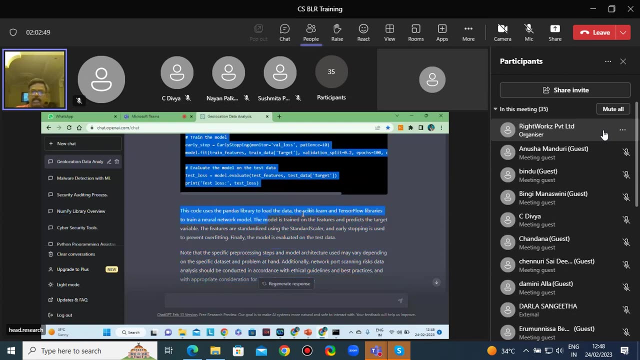 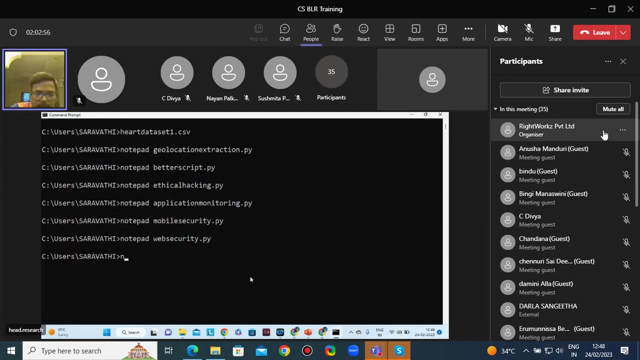 Ok, so the example for the p, p, p, ppto's. It is seen that it is known as a ppmrep. it will come out like this: p ripr for the. he is enough code. see, now i am giving network notepad: space network port scanning, tmi network port scanning. 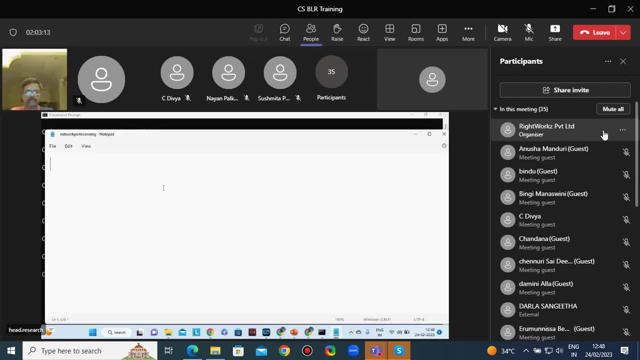 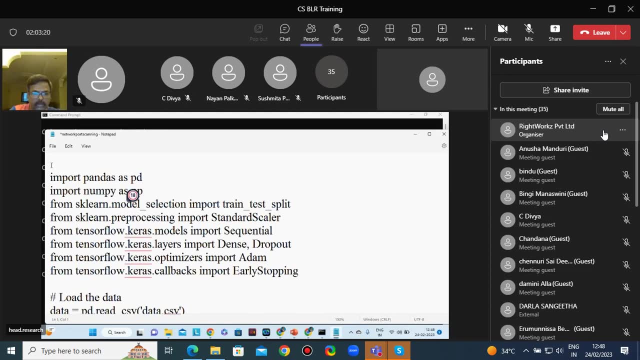 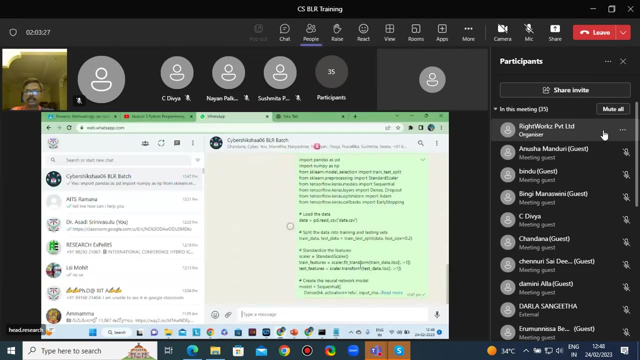 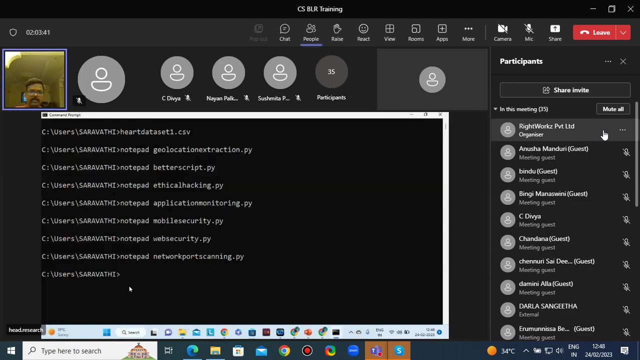 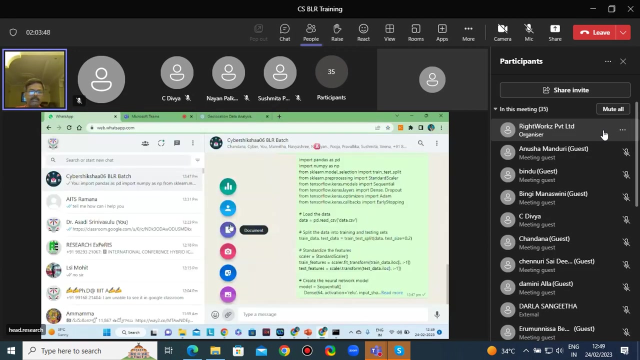 so i am creating one file. ok, i am giving the name of the program, python code for network tmi and say network port scanning: ег, eg, eg, eg. Please download from the internet whatsapp. I have given whatsapp network you need to. 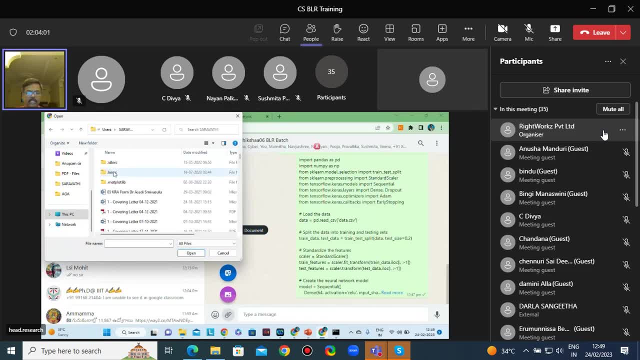 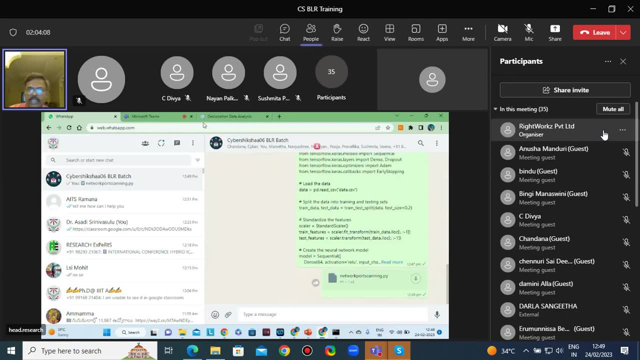 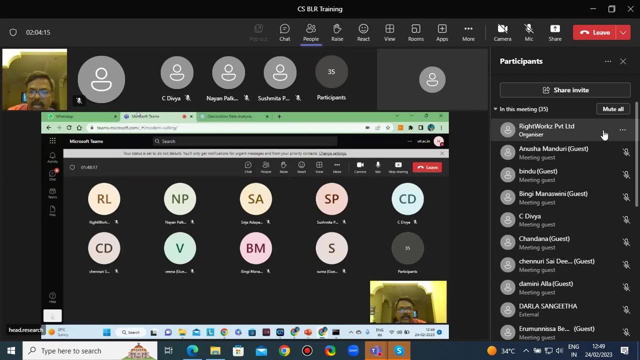 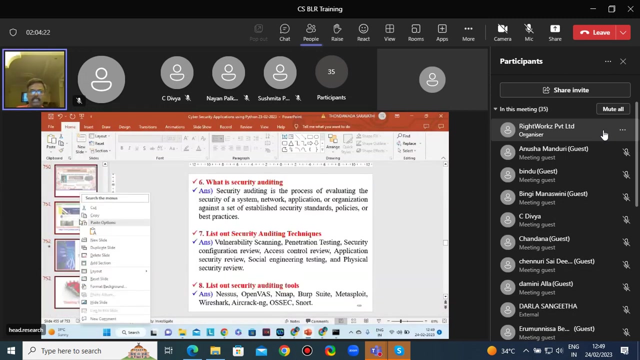 go to users network code scanning: see here. ok, Next one project. one more group is left. can anyone identify All all departed? now check all of them. I don't think one project is left remaining. I have given all for ten projects. I have given. let me check right now how many projects. 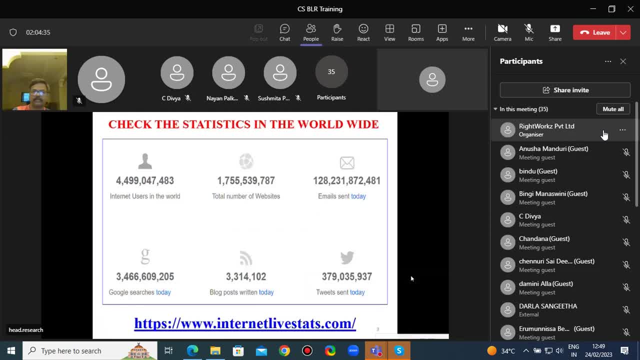 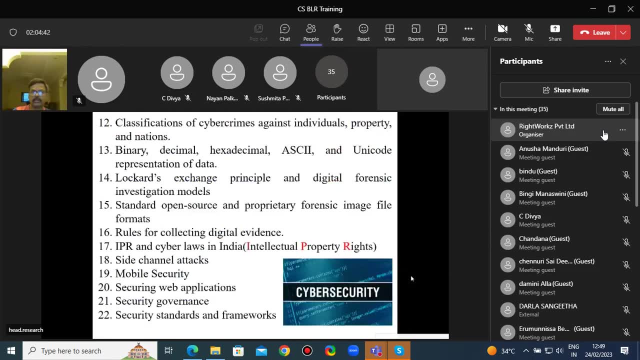 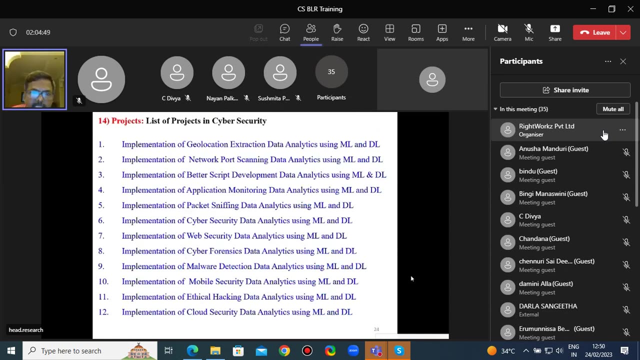 we have given. Yeah, these are the twelve projects. implementation of geolocation: whose batch this geolocation? implementation of geolocation extraction: Sir seven, sir Seven, batch number next: implementation of network code scanning data analysis, batch number One. 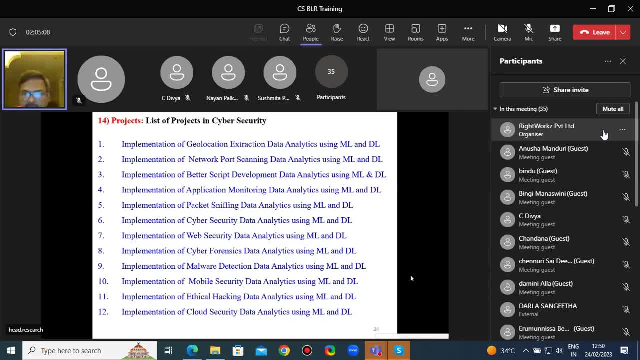 Yes, One batch number network code scanning. this one is completed. better script development: Yes, yes, sir, good. Next, application monitoring. I have given packet scripting data. I have given cyber security data analytics- ok, Cyber security data. I have given web security. I have given cyber forensics. I have given. 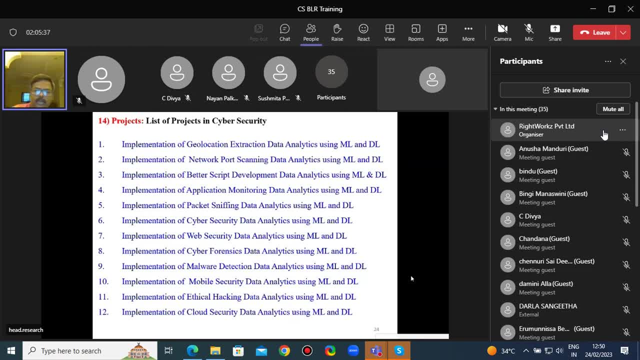 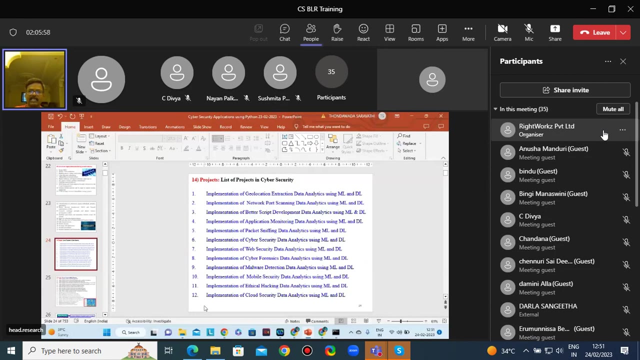 i have given malware detection, i have given mobile security, i have given ethical hacking, i have given okay. 12th one is cloud security. if anybody would like to do this project also very, very important. okay, 11 batches is over now. 12th, if anybody interested, is cloud security issues. 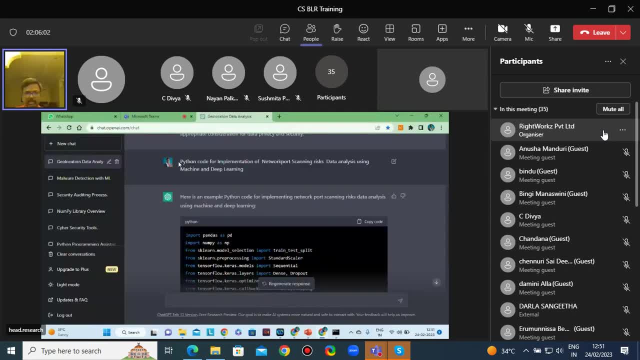 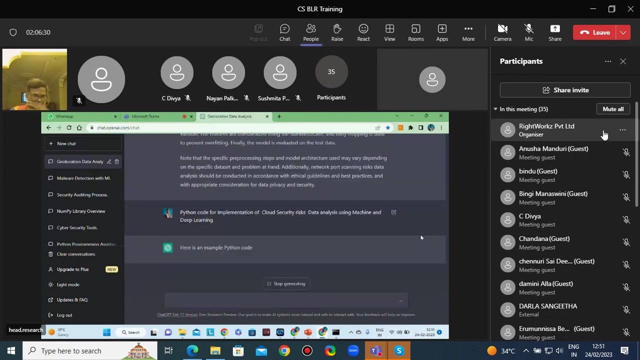 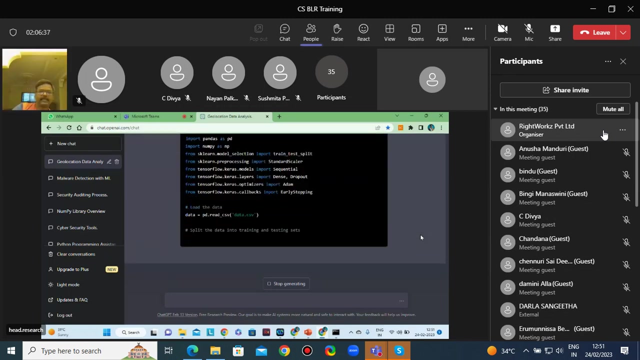 very important project. i am going to help you. i will take, i will take today. i am going to execute this. wait, wait now. security risks, cloud security risks, data analysis. so data set: you need to collect that. that is very, very important. once data is collected, you need to collect that data. if you are using cloud security, you need to. 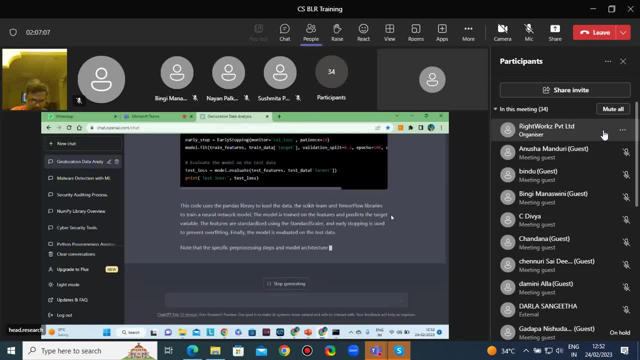 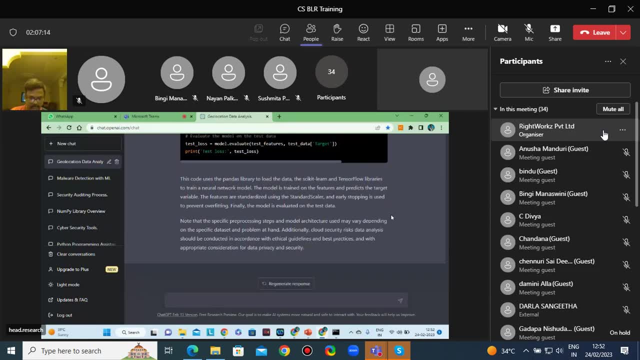 keep track of your data and that is very, very important. so just wait until the data is collected. so it will be very, very important to keep track of your data and to keep track of your data. i will see, Please. I am giving 12th project code if anybody is interested. please see cloud security. 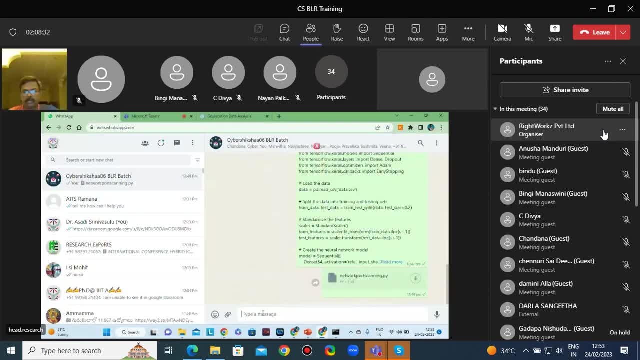 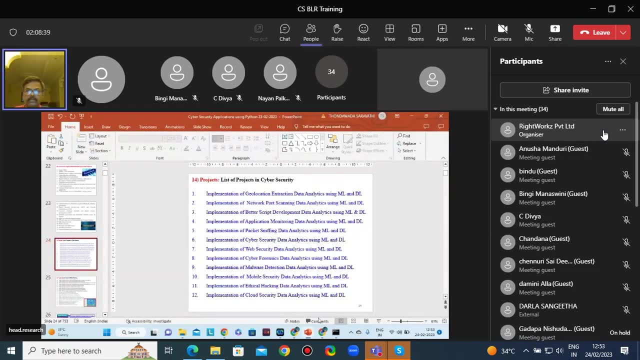 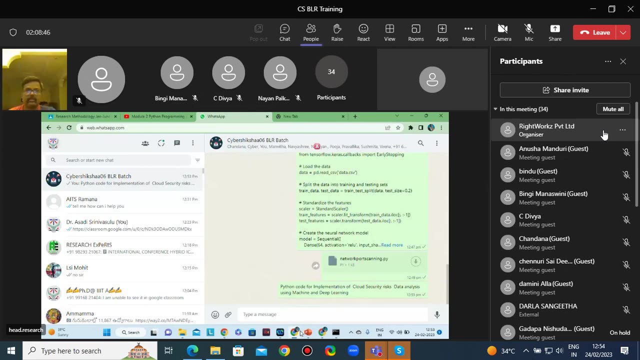 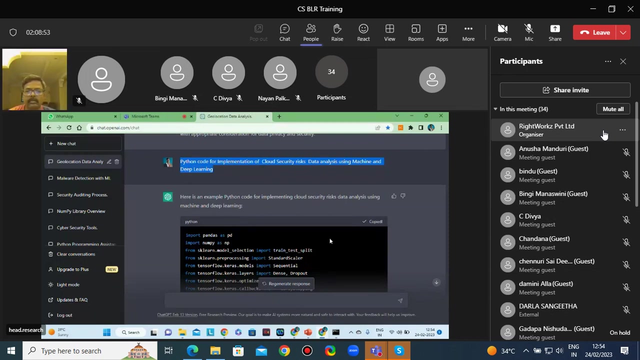 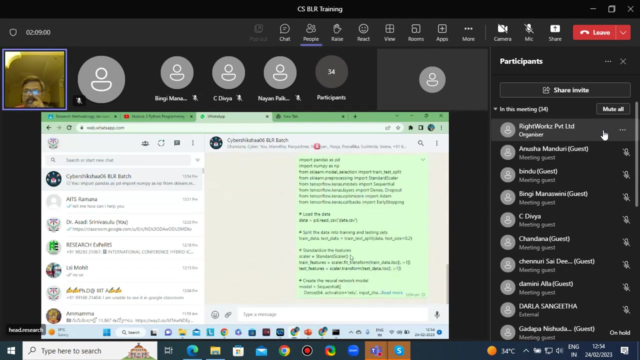 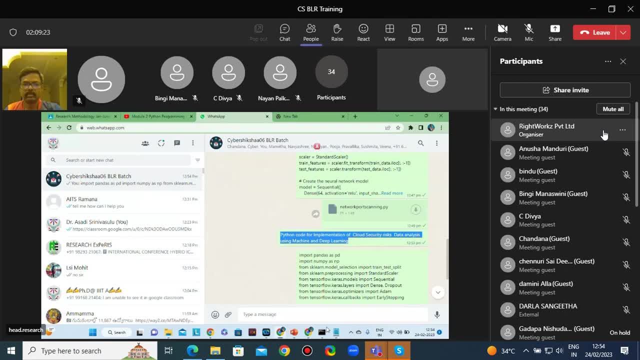 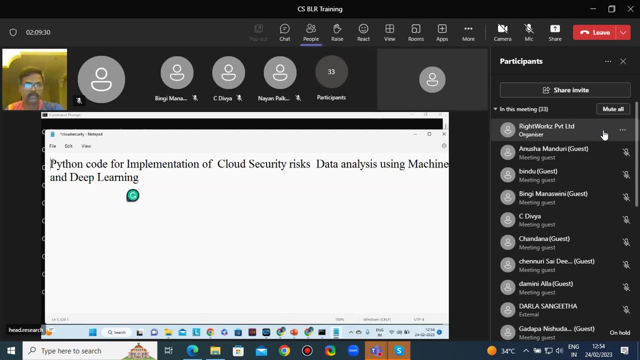 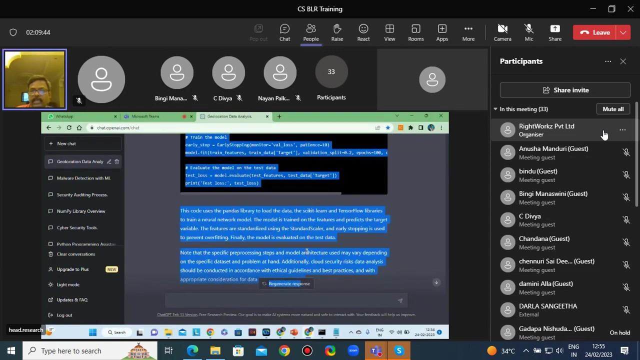 I am giving 12th project code. if anybody is interested, please see cloud security. I am giving 12th project code. if anybody is interested, please see cloud security. so with this one i am closing the project implementation. now i am giving 11 to 11 batches. 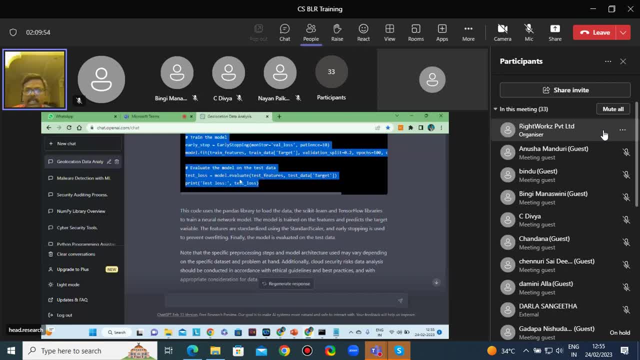 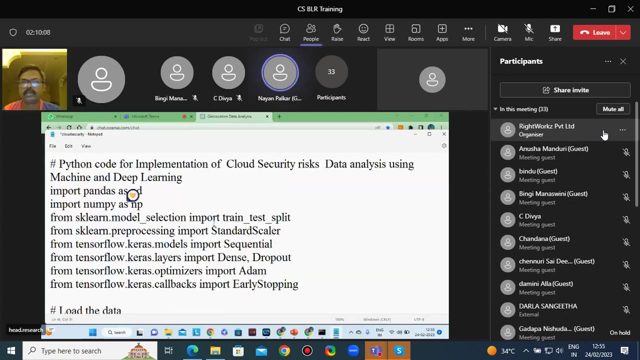 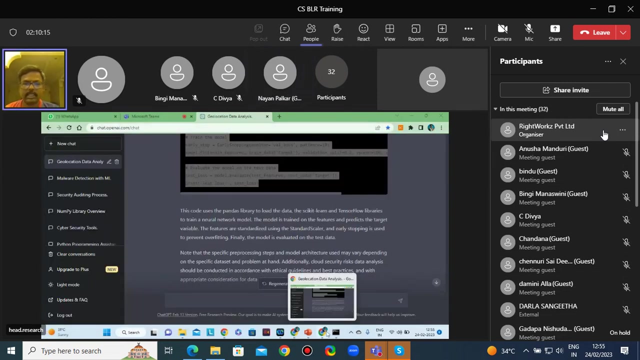 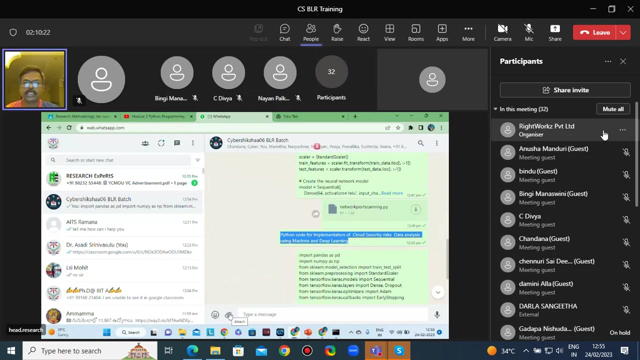 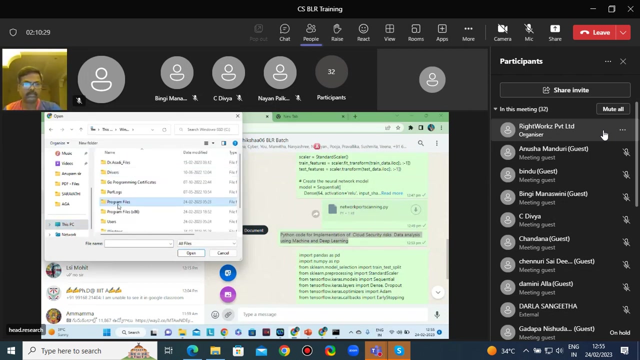 11 tools. please write down, nayan. i am giving the 11 tools- cyber security tools. you need to give presentation next week, including this one. nayan, please write down group one: okay, last project: this is the project. okay, please write down, nayan. i am giving the. 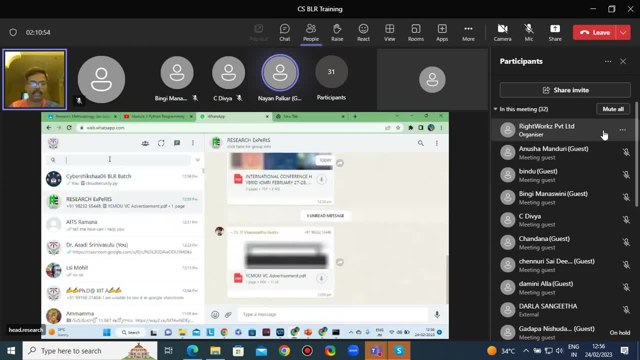 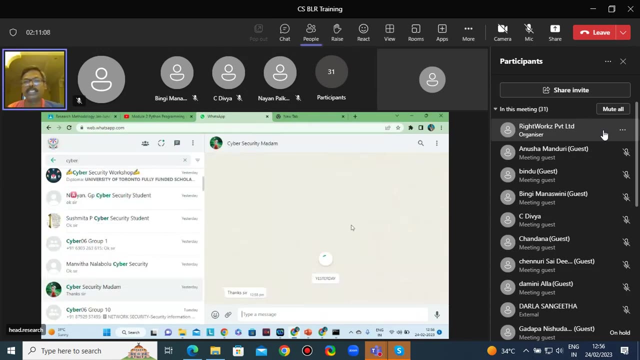 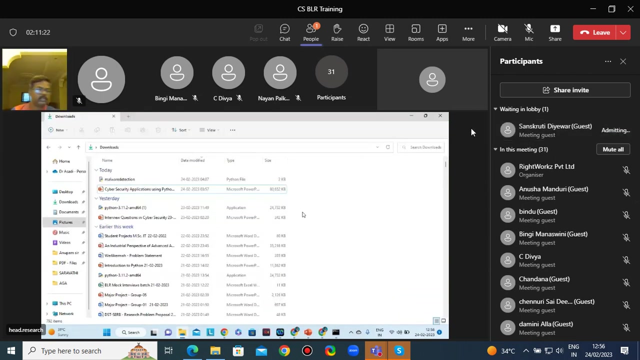 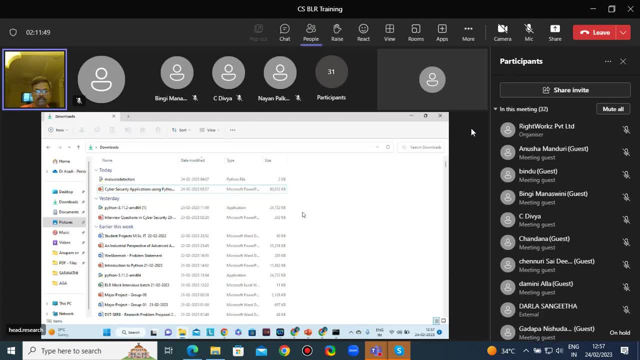 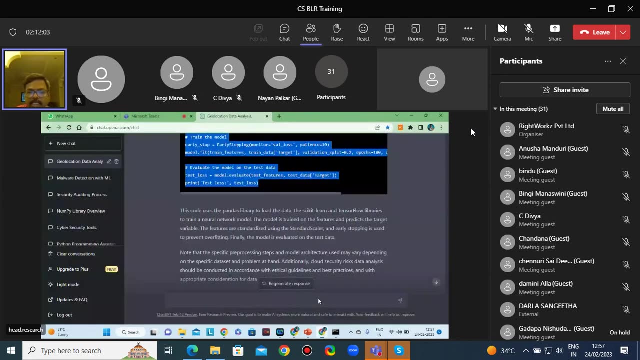 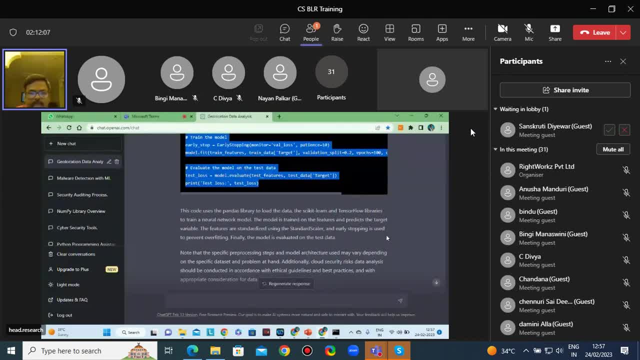 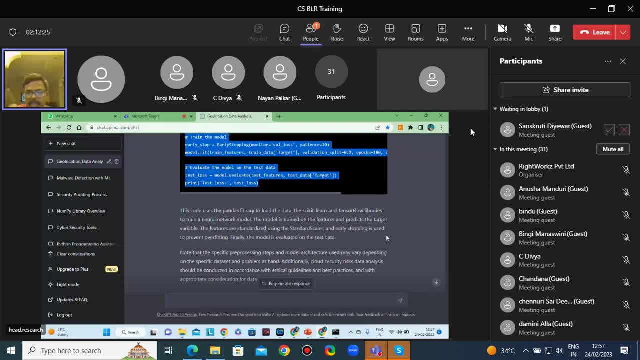 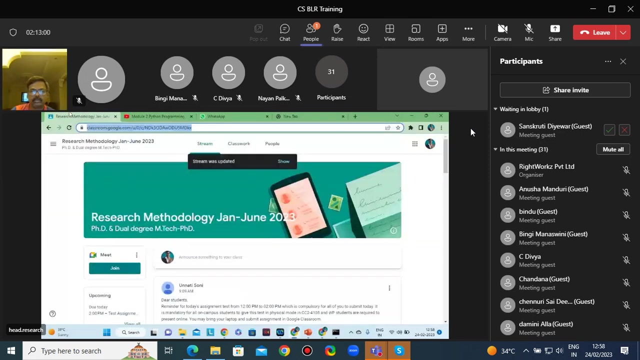 and practical example. Try for practical example Like that: 20 to 30 slides you can prepare about the tool. Next of second group: Second group: write down: metasploit, Metasploit, Metasploit. Next group: 2. Next group: 3. Wireshark Group: 3 is wireshark Group. 3 is wireshark Group. 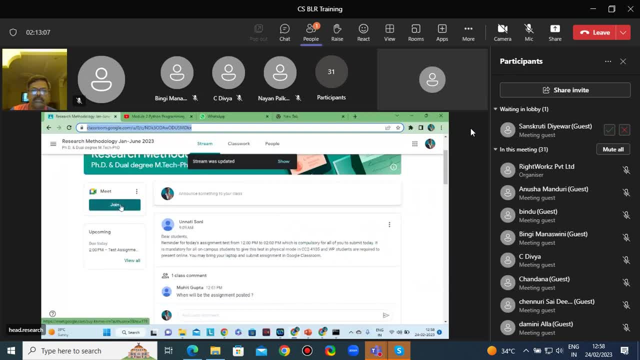 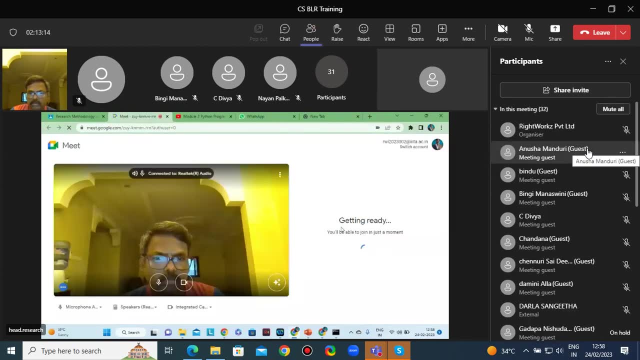 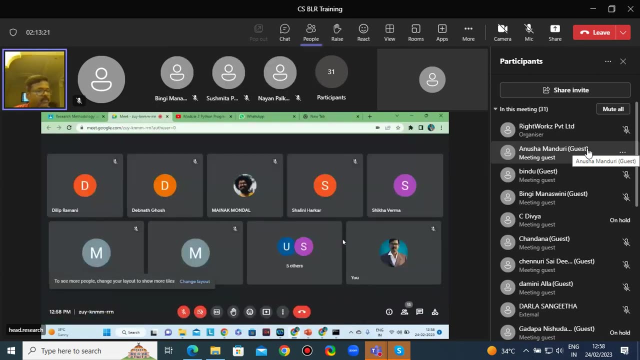 3 is wireshark. Next group 4. Purp- P-U-R-P Purp. Next group 5. Snort Nayan. are you writing? Yes, sir, I am writing sir. Group 5. Snort. 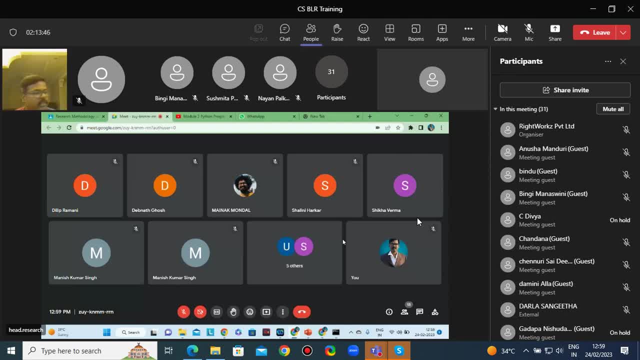 Snort. S-N-V-A-R-T is snort. Next Group 6. Nessus- N-U-S-S-U-S. Nessus, Next Seventh, one, Seventh, two: O-S-S-E-C. O-S-S-E-C. 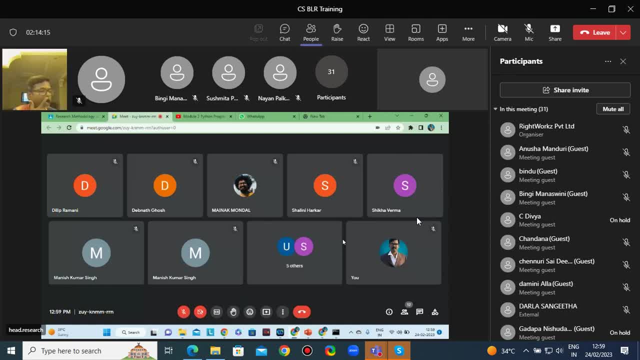 O-S-S-E-C. Next: Polylinex, Next batch. Next batch number Nayan. batch number 8-8.. Polylinex. Please write down. Next Ninth one: Aircrack-NG. Please write down Aircrack-NG.